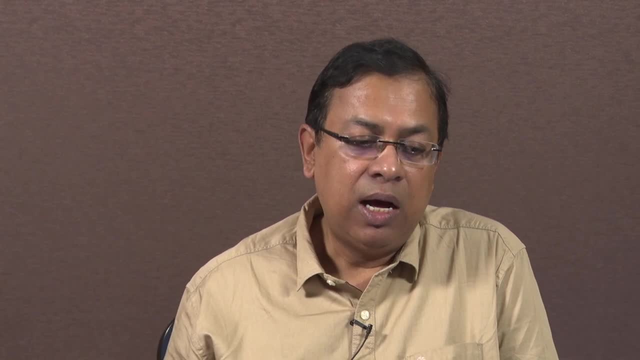 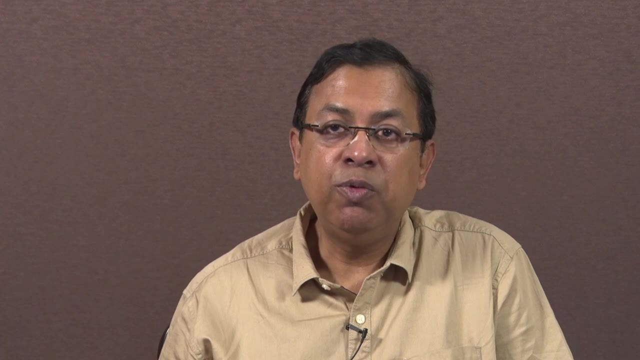 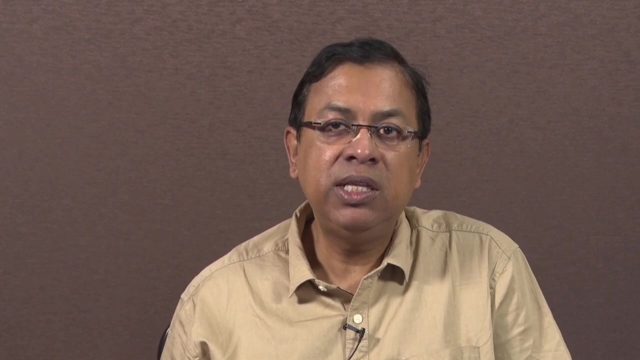 earlier and we will be talking about this. So the quantum mechanical nature of the electrons in presence of a magnetic field will have to be worked out, and we have to understand how these plateaus arise and why they are so robust, so much So that they actually 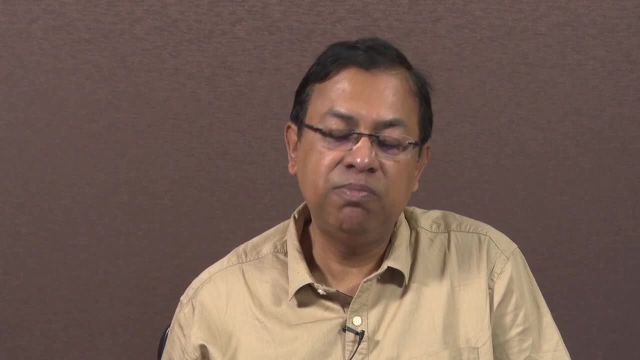 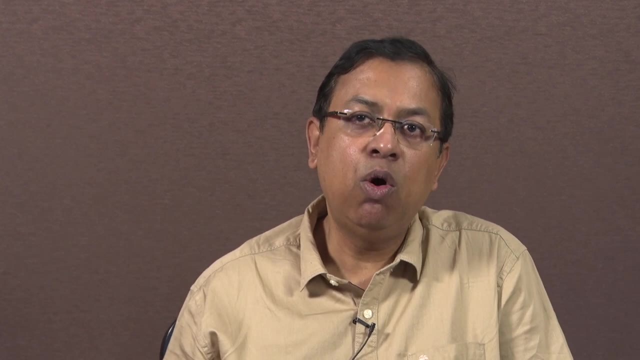 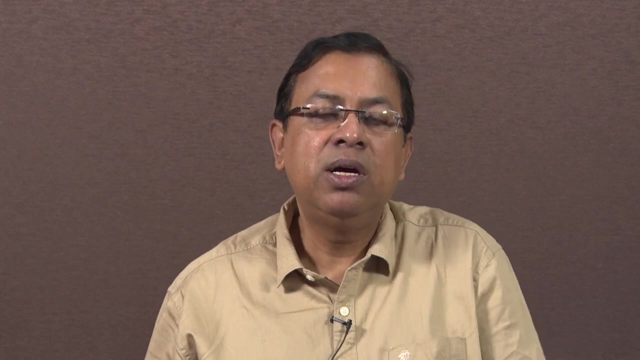 give the benchmark of resistance, the plateaus. actually, h over e square sets the scale of resistance, which is 25.813 kilo ohm. and we have to understand all that. But before that, for one last time, let me do the classical analysis in order to understand the behavior of charged particle. 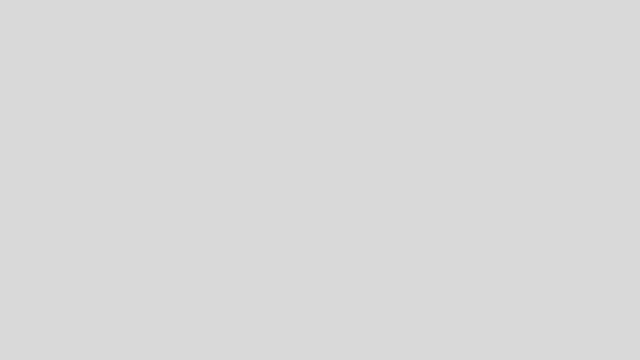 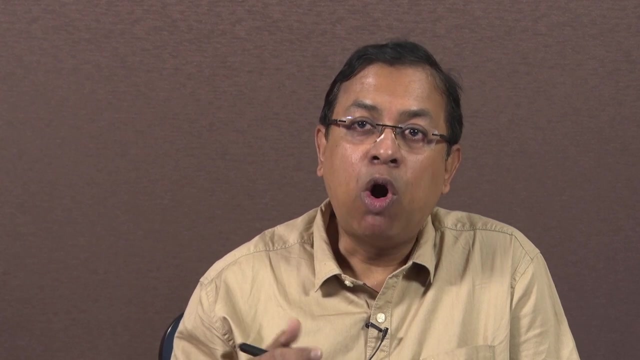 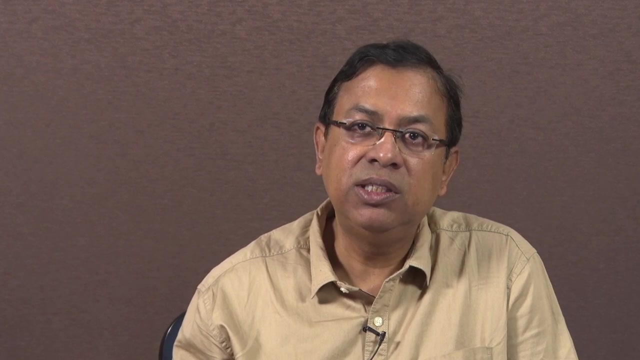 in a electromagnetic field or a magnetic field say, and we have of course done this problem at equilibrium and we wanted to understand that- what happens or how the Hall voltage develops in the transverse ages of the sample when there is a longitudinal current being sent from one end to another. and that was an analysis that was done and at equilibrium. 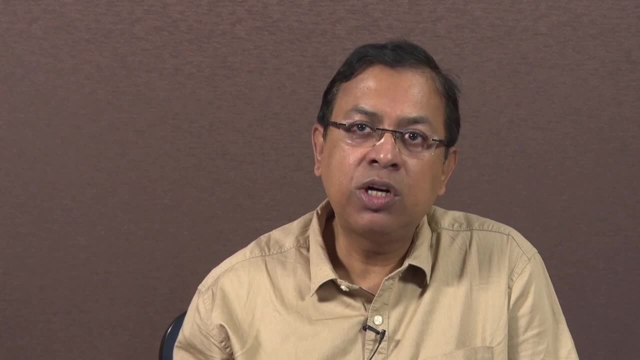 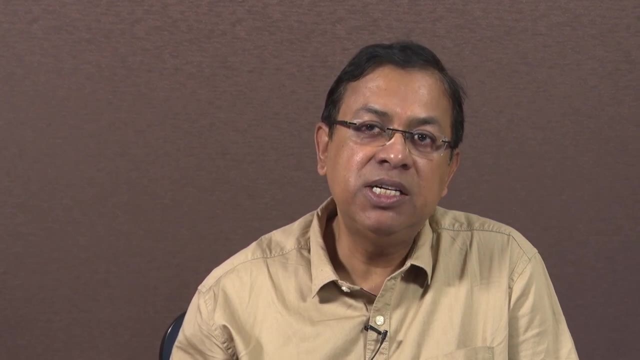 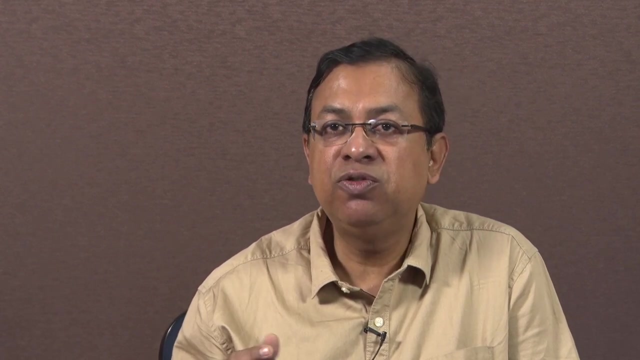 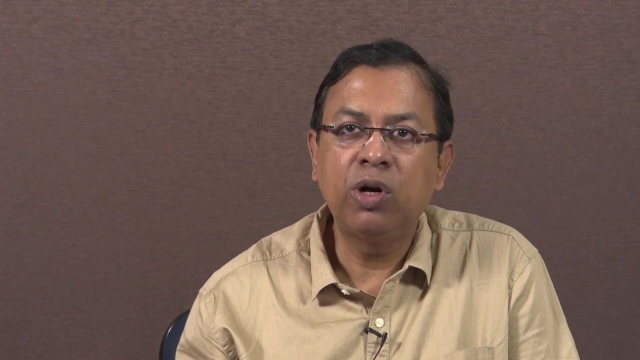 when the force vanishes. But we have not talked about what is the trajectory of the particle in presence of an electromagnetic field, And this is important because the trajectory being actually a path that is followed by a particle, a charged particle, should not really depend upon whether we are talking about classical 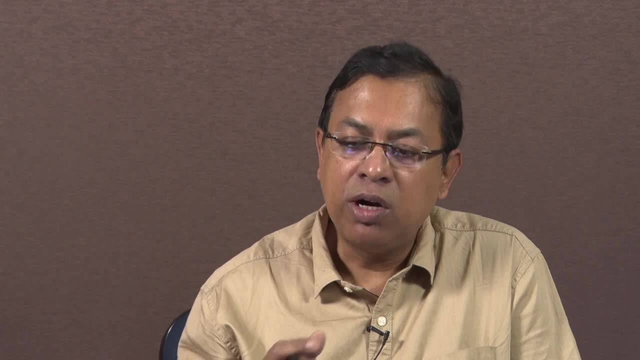 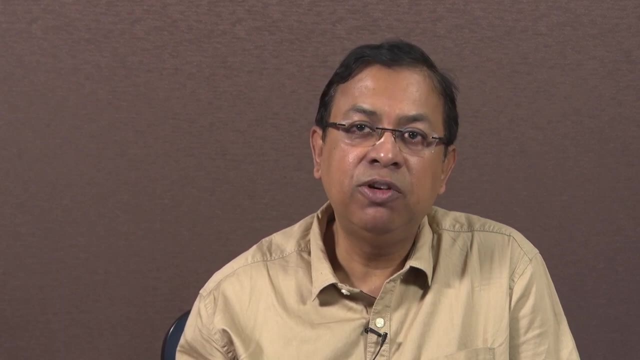 mechanics or quantum mechanics. Of course, in quantum mechanics we rarely discuss or worry about the trajectory of the particle, for the reason that the trajectory is it is. there is an uncertainty- And this is done with an intention- that there will be a range which will pronounced to the 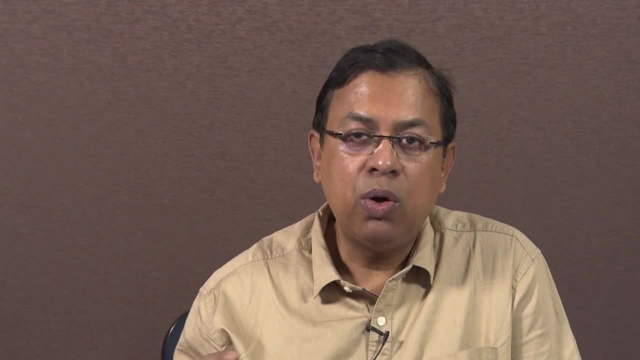 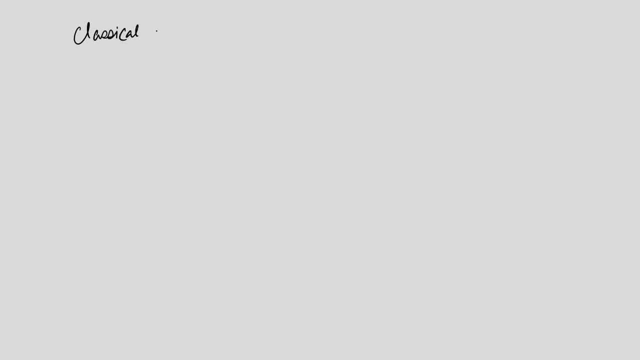 state of released randomly In the final inference for the complex stoichiometric belief Due to this thinking Ding is saying So. the goal is that we are talking of will be dealing with a quantum mechanical system soon. So let us talk about two cases. 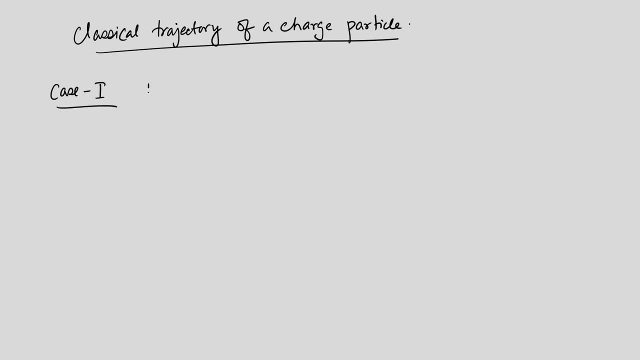 the case one being where there is no electric field and there is only a magnetic field, which is constant, which is not equal to zero, it is finite and it is uniform. So this is the situation one, that is case one, say, and the energy is constant. So please do not confuse. 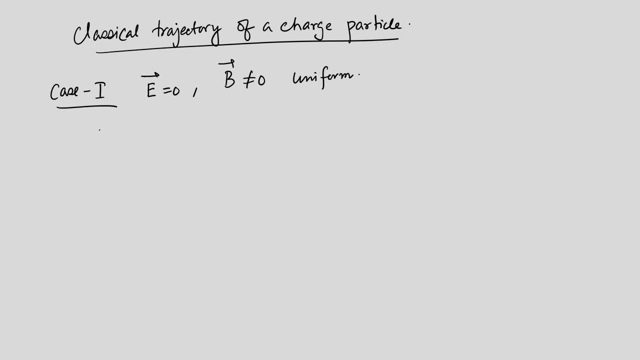 between the electric field, E, and the energy. energy is a scalar, So energy is a constant. and energy is constant because of the reason that the power delivered is equal to zero, which is nothing but the low range. force is V cross B, and that is why this is equal to. 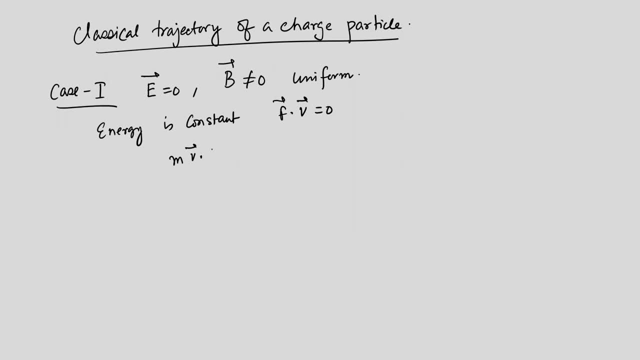 zero. So we can write this as MV dot, V dot, which is equal to DDT of half MV square, and this is equal to Q into V dot, V cross B, which is equal to zero. So this is your F dot V, because your F is the low range force. when there is no electric field, it is only the magnetic. 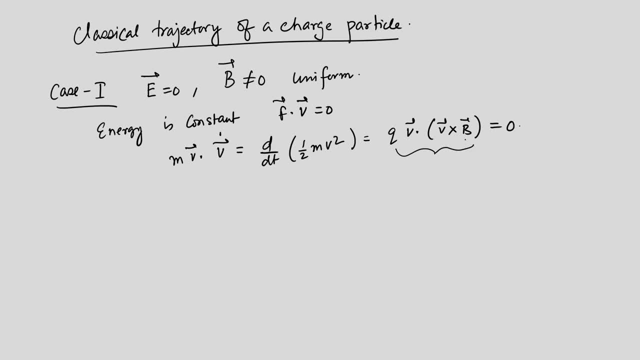 field will create a low range force. So V dot, V cross B equal to zero. the reason is simple. this V cross B is a vector which is perpendicular to both V and B, and that is why if you take a dot product with V, it will give you zero. and that is why a DDT of half MV square equal 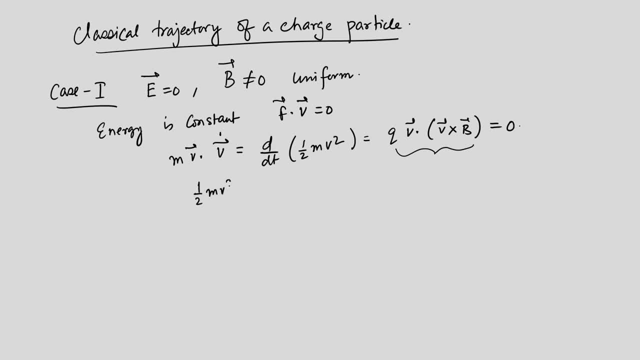 to zero, which means half MV square equal to constant. okay, and this is what we mean by the energy being a constant. that is only energy. that is left in the problem. So this is a perfect example. So its normal response is zero. OK, if you want to be able to interpret an energy being. 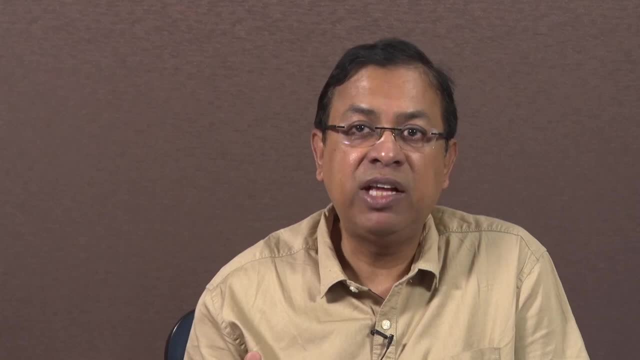 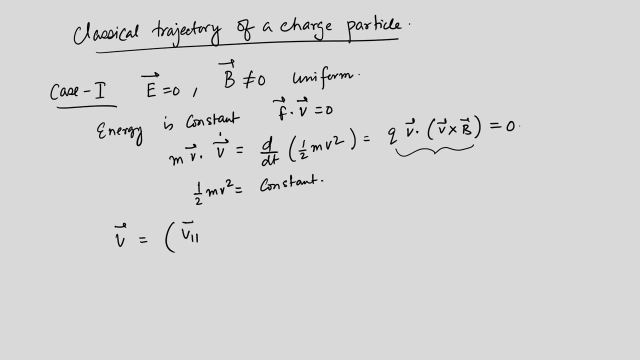 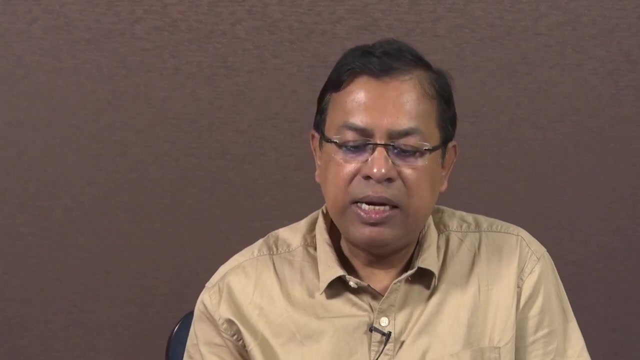 a constant. yourع Lösungsvered Look out for this point and you have a certainскan you want to interpret. the angle is zero, equal to zero, And it is going to define means your action number's going to be zero, And this point. 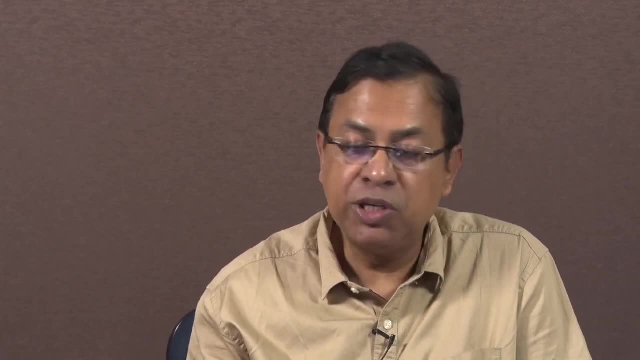 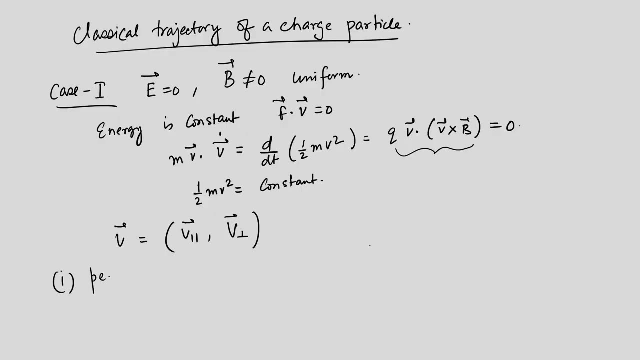 is going to represent with this equation. if you want it to be zero, this direction is exactly the dramatic half m Come to Q and this equation here is going to give you a reason for that. So let us talk about the perpendicular motion And what we mean by the perpendicular motion. 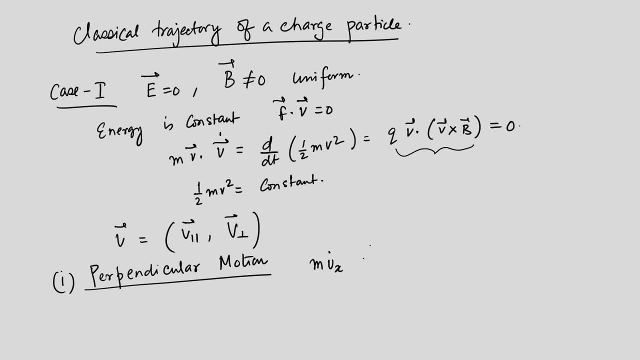 so we have MVX dot. this is equal to QVYB. So this is, say, equation number 1, and the equation number 2 will be MVY dot, equal to minus QVXB. We are continuing with the same situation where E equal to 0 and B is uniform and not equal to 0. 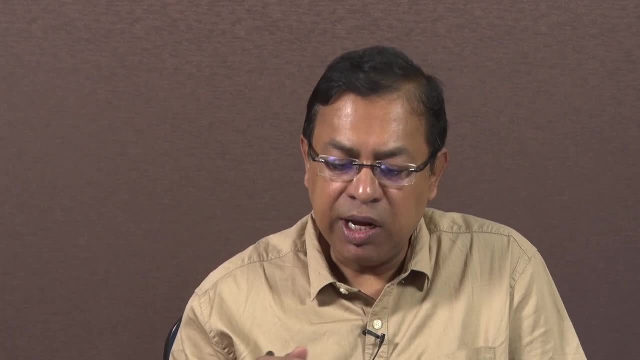 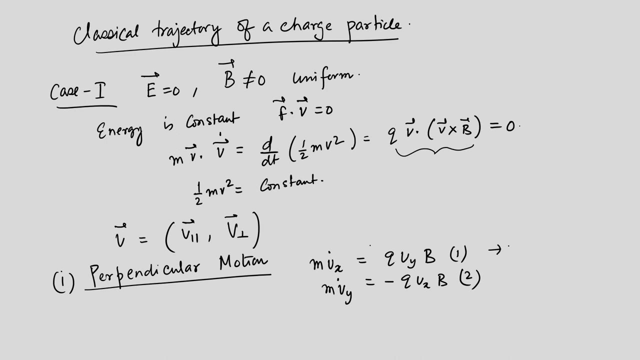 And we are just discussing, or rather deliberating upon the nature of the motion, and this is quite instructive. If you take a double derivative of this, so differentiate with respect to, with respect to time t, and then, of course, use 2.. So then, MVX double dot, so this is equal to QVYB dot. 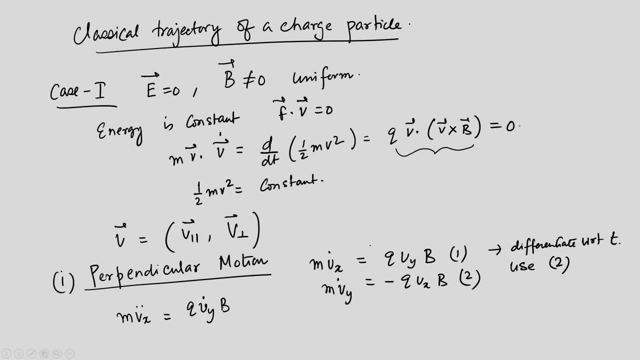 by B I mean into B, and then I can take this M to be in the denominator. This is in the denominator. So this- now I will use VY dot to be here- So this is equal to Q into B by M, and then this is equal to minus Q into VXB divided. 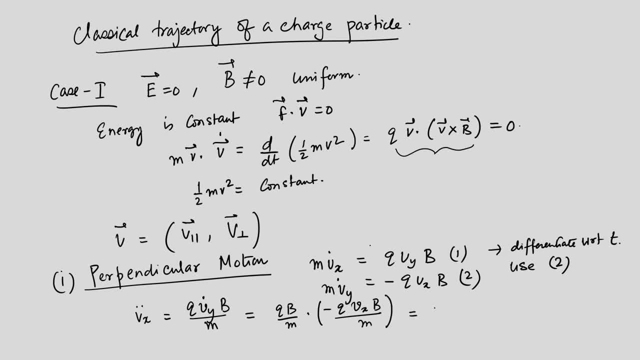 by M. So this becomes equal to minus QB by M square and VX, and this is equal to nothing but minus, which we have written it earlier, that omega B square, VX Or omega B is nothing but equal to QB over ām, which we have. 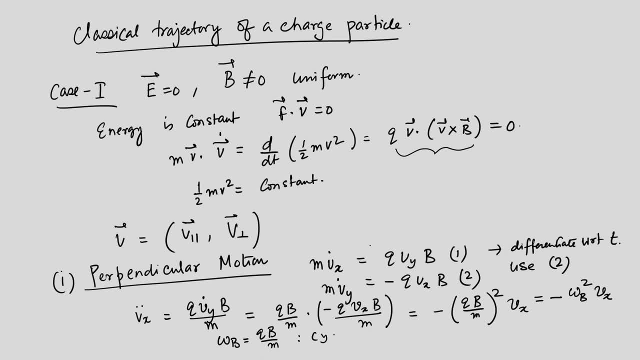 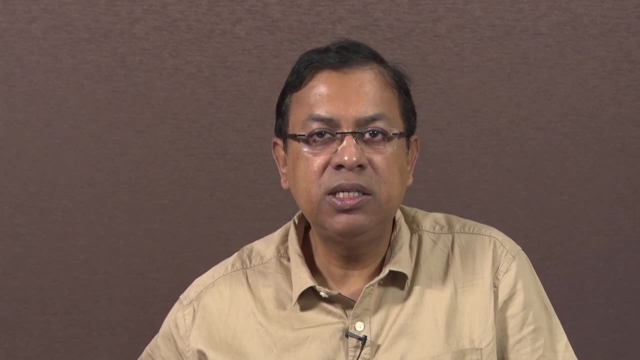 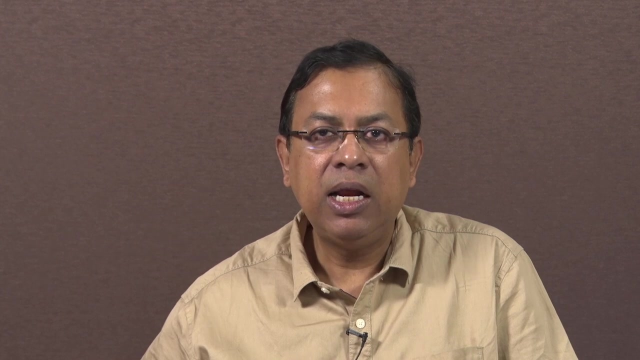 Which is D, called as the cyclotron frequency even earlier. So just a quick recap: we are talking about no electric field and a charged particle is moving with a velocity V, which is has components Vx and Vy. and this is there. is a B there, that 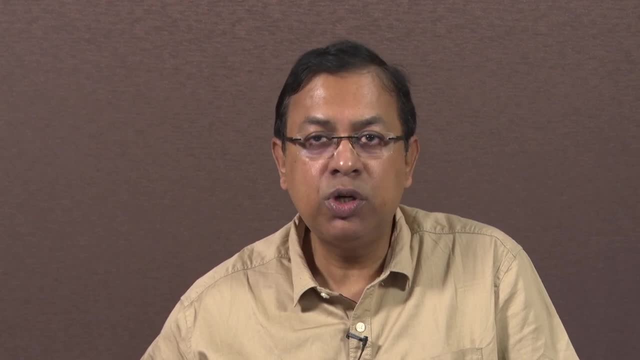 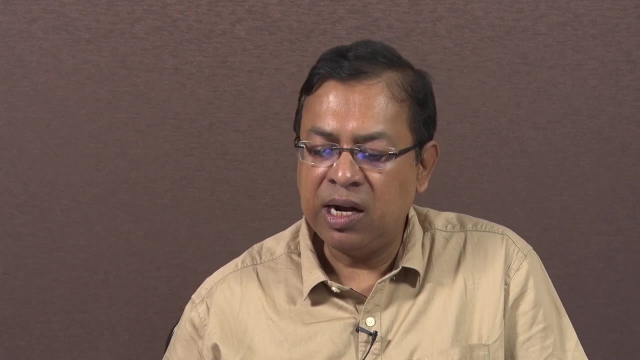 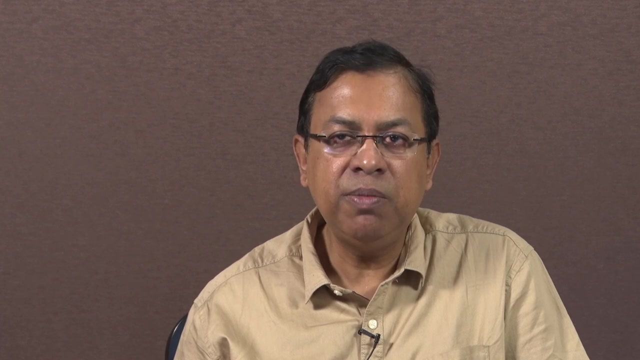 is a magnetic field. because of magnetic field there is a low range force and in this particular case we know that the energy is constant because the F dot V equal to 0, and now we are analyzing the motion by writing down the equations of motion. So MV x dot equal to Q Vy B, because F is equal to Q V cross B, and that is why the x component. 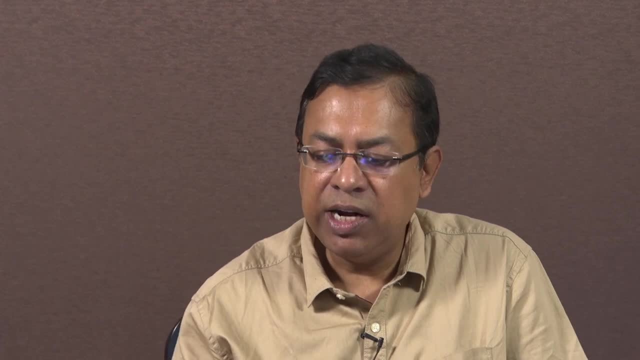 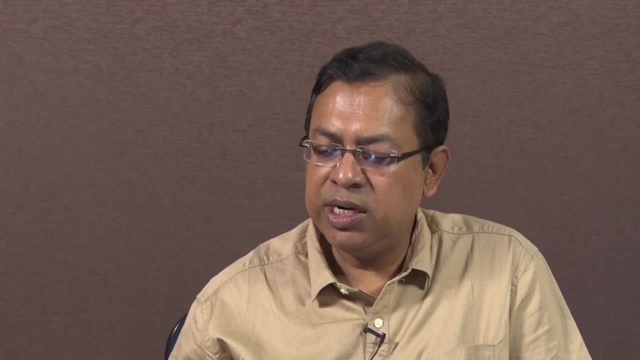 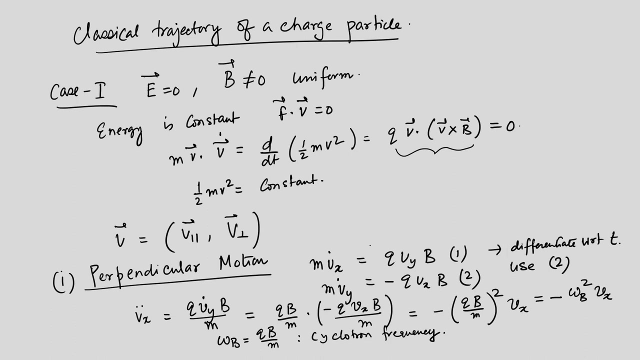 or the derivative of the x component of the velocity is related to the y component of the velocity. Similarly, for the y component is x component, but with a negative sign, and now I did some little manipulation here in order to write this Vx double dot. now the end result is that 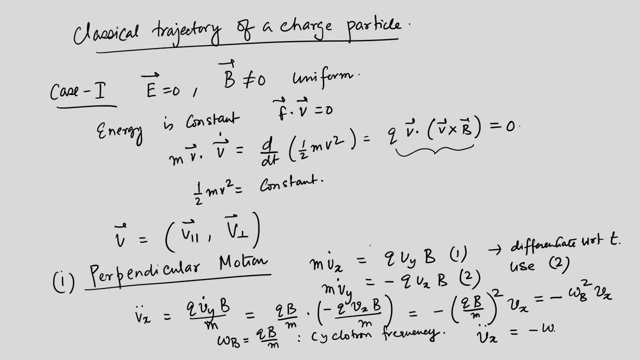 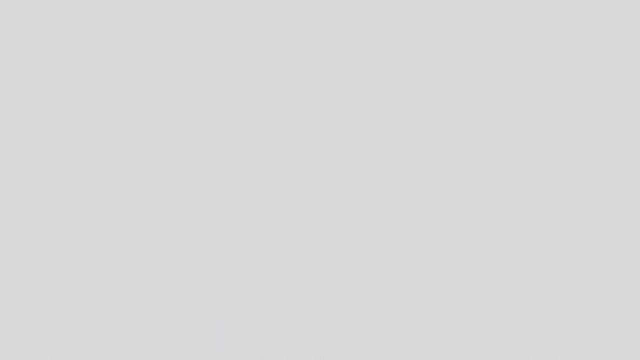 the Vx double dot becomes equal to minus omega B square V of x, and all of you know that this corresponds to a harmonic motion where Vx will harmonically depend on time, And so this is what the solution is, and the solution is that Vx is equal to V perpendicular. 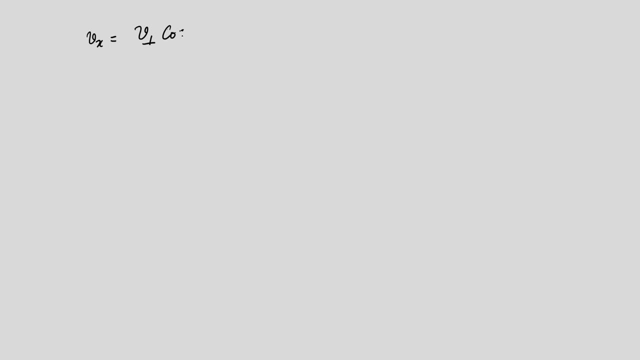 which is the, because we are talking about the perpendicular motion, and it is cosine of omega Bt. And similarly, if you do the same calculation for Vy, then Vy turns out to be M divided by Q, B into Vx dot, which is equal to a minus. 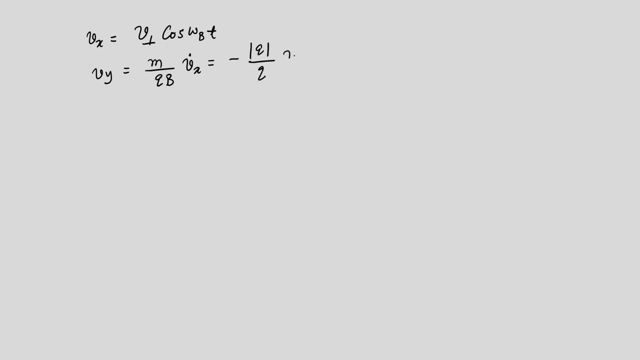 minus Q, divided by a Q and a V and a sin, omega t, omega b t. So this is the trajectory for the perpendicular motion. So this is the trajectory in the x direction and this is the trajectory in the y direction and why we are talking about the 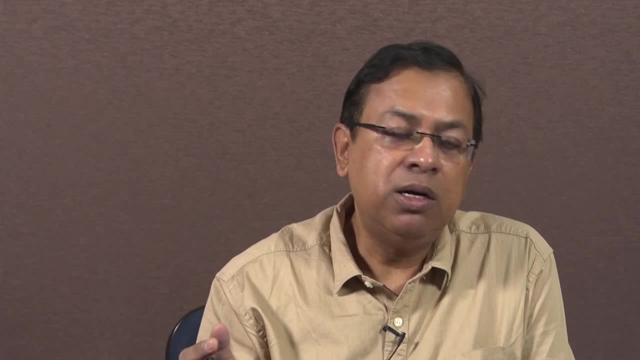 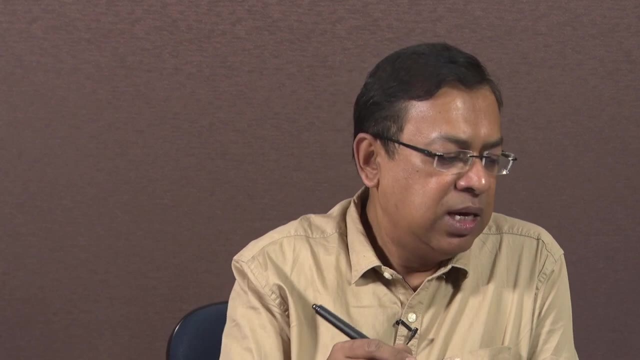 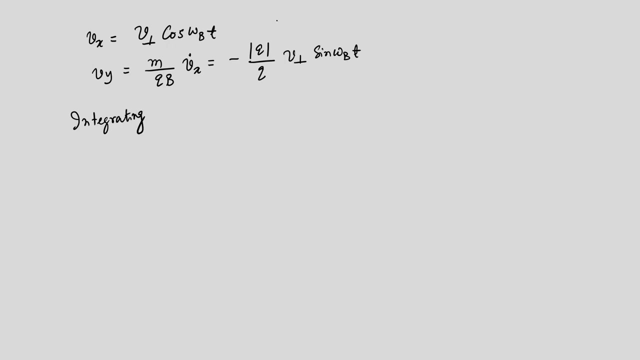 perpendicular, because we are considering perpendicular to the magnetic field. So if you integrate and want to know that how the trajectory looks like, then you will get. So, integrating these equations: we have already written 1 and 2, so this could be 3 and 4. so integrating. 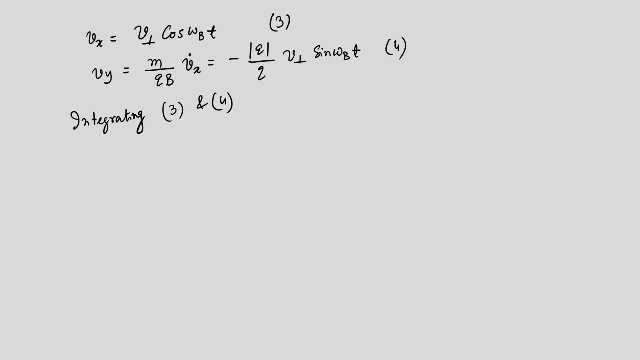 3 and 4 and using you know some initial conditions. So x is equal to x0 plus a V perpendicular divided by omega b and a sin omega b t, because I integrate it with respect to t. So this will give me the: 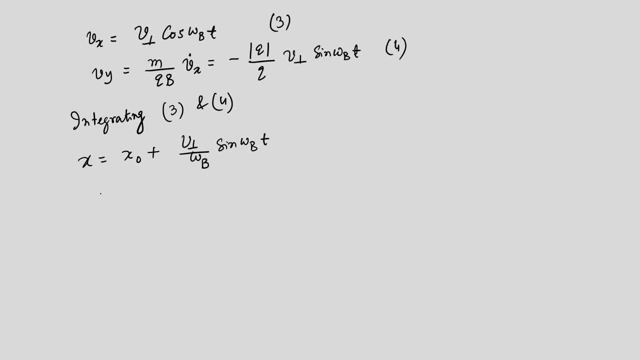 x motion and the y motion is almost similar, harmonic, but out of phase, by an amount, pi by 2, this is a cosine, omega b, t. So this is the x motion and the y motion, and it is clear that if you superpose this motion you get a circular motion. and let me show that. 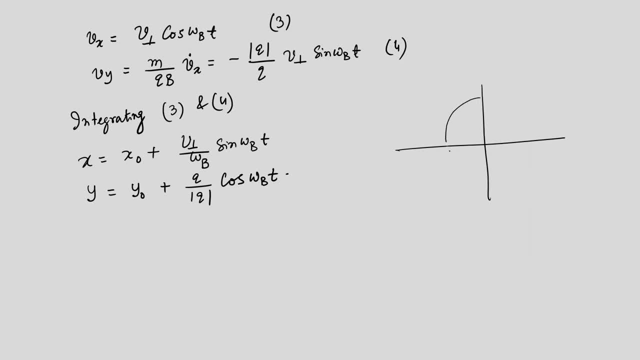 circular motion. Let us see how neatly I can draw a circle. not very good, but this is that circular motion that we are talking about. about this point: x 0,, x 1, x 2, x, 3,, x, 4, x. 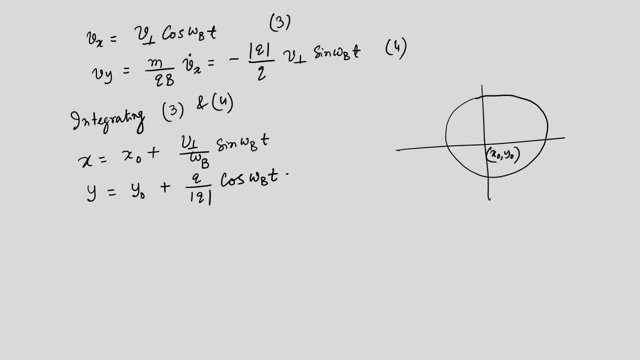 5, y 0.. It may look slightly shifted towards the positive side, but that is not what is intended and this things are, so this is the radius of that. So this is where the positive q motion of the particle that is clockwise, and this is the motion when q is negative. 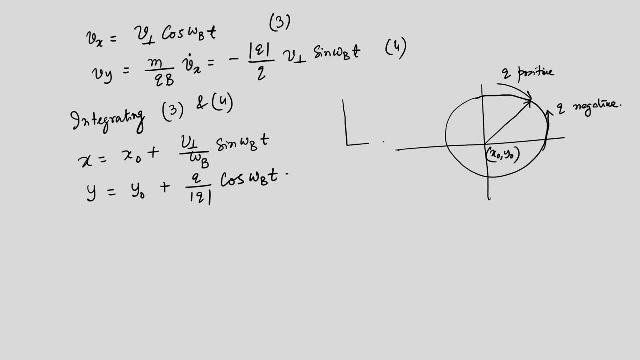 and if you want to know the, you know The axis, because this is very important. So this is the x and this is the y, and this is z and this is the direction of b. So b is in the z direction and this is the planar. 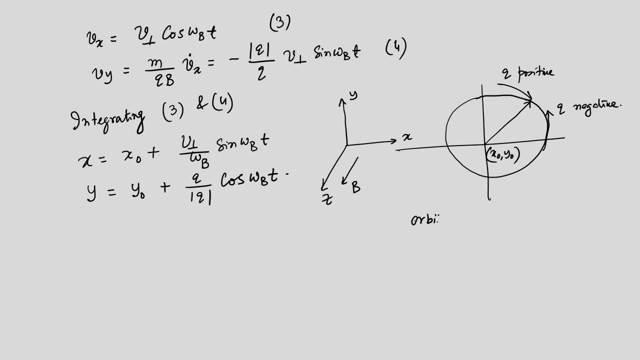 motion. So this is the orbit of a charged particle About a guiding centre, A guiding centre X 0, y 0,. okay, So this is called as a guiding centre, This point about which the motion takes place, and this is pretty much the motion of a charged particle, only in a magnetic field. 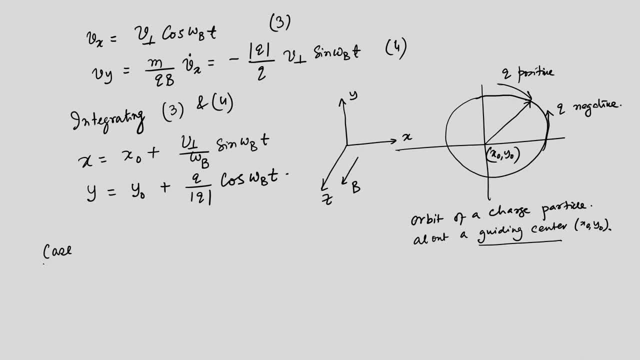 So let us look at case 2 now, when we will talk about E not equal to 0, B not equal to 0, okay, but E is perpendicular to B, okay, So it is basically a generalized condition of the one that we just saw, and we can write down the equation of motion, which is F, which 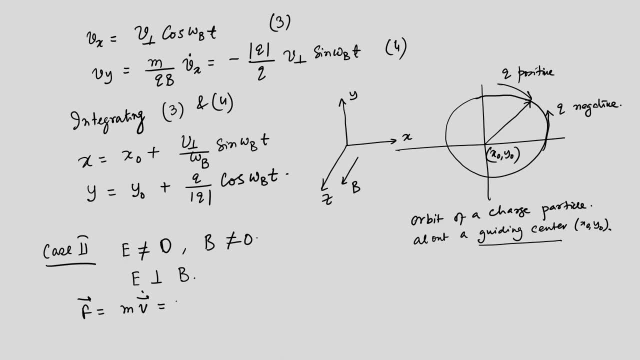 is equal to MV, dot, which is equal to q, into E plus V cross B. Okay, now the total force has a component, or rather a contribution coming from the electric field and earlier, of course, for E equal to 0, which is the case 1, which we saw, your V parallel. 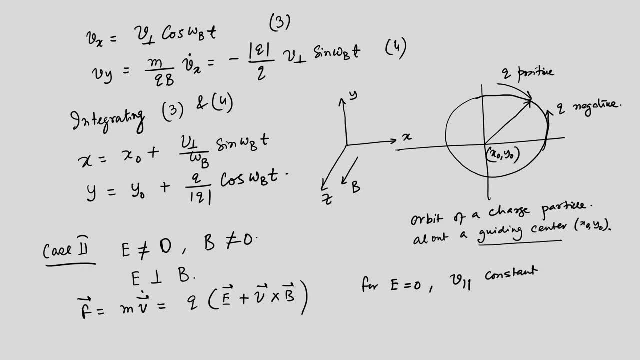 was a constant, So the parallel component of V, but now, because of this, the parallel component actually, Okay, an acceleration which is given by the q, e and the parallel component of e divided by m. So what happens is that there is no fixed guiding center that you are seeing here, the guiding center. 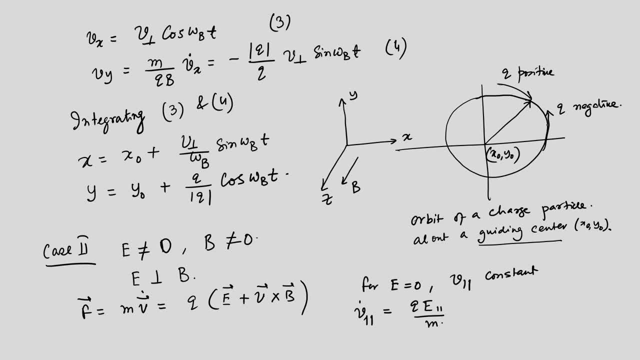 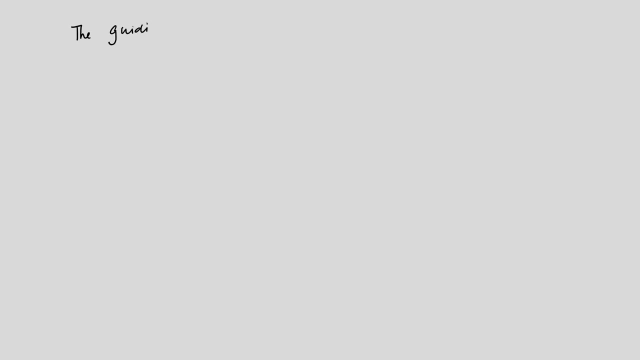 remains fixed and the charged particle, either in the clockwise direction or anticlockwise direction, depending on its sign, would just move around this circle. But now this guiding center keeps getting drifted because of the electric field. Let us see that. So the guiding center, which was earlier 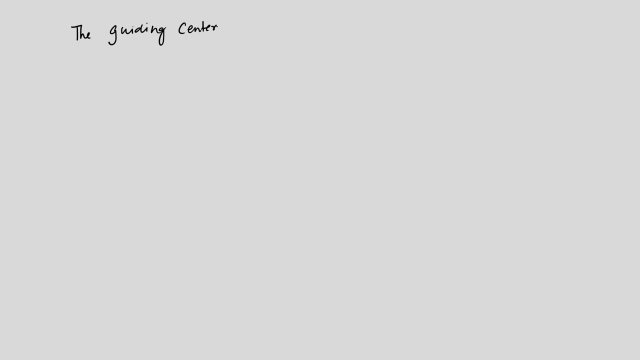 we have denoted it by x 0 y 0.. So this guiding center, x 0 y 0, it moves perpendicular to both E and B. Okay, So this guiding centre moves in that direction. So the charged particle drifts the charge. 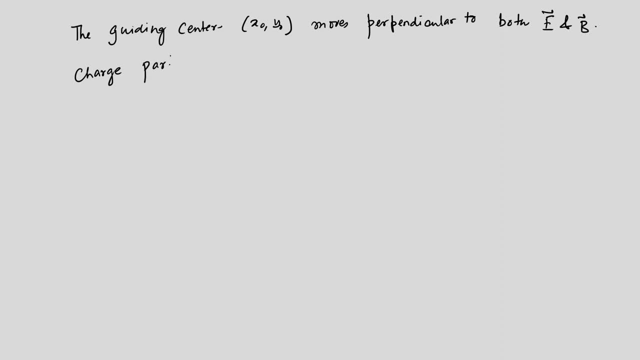 particle drifts with a velocity v d. Okay, Okay, Okay Okay. reason that writing this is that there is another component of velocity, or rather another contribution to the velocity, which you also will have to worry about Now. this is because of the guiding center that you know moves in a direction which is perpendicular to both. 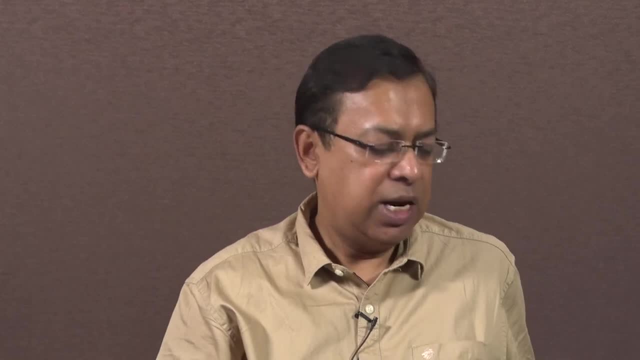 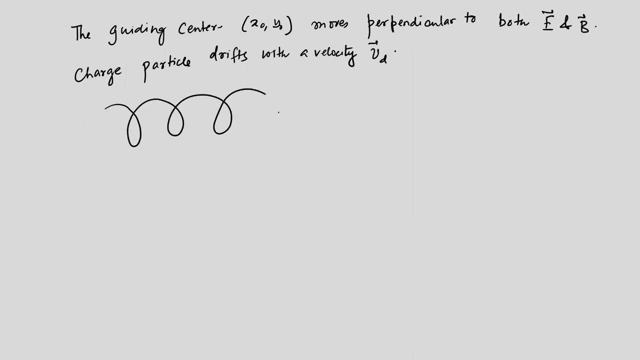 E and B. the charged particle has to drift and this drifting actually is represented by like this and so on. So the drift actually happens in this direction. and, in particular, suppose you have B to be pointing inside the screen so that you know this is usually represented, because you see. 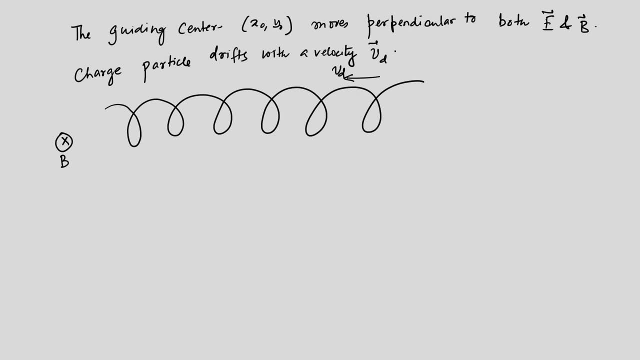 an arrow, the back of the arrow, if you see, it looks like a cross and that is why, when you write it with a cross, a direction, which means it is going into the plane of the paper, in this case it is a plane of the board, or this white board that you are seeing and we have. 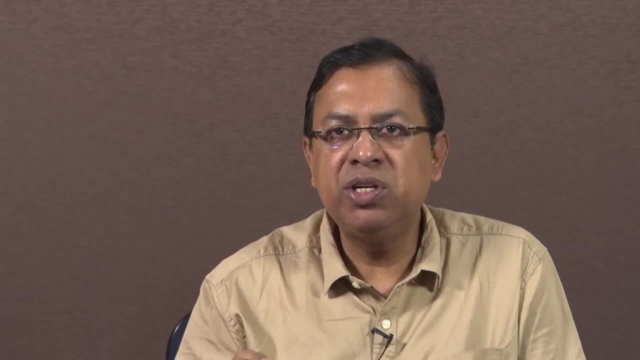 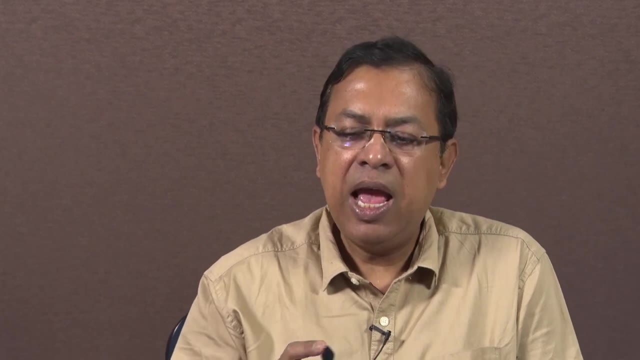 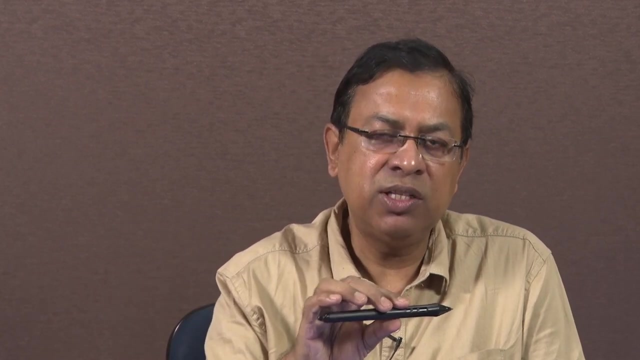 electric field in this direction. So one is going piercing inside the board and then the other. the electric field is in this direction and then the drift happens in a direction which is perpendicular to both, which, in this particular case, It happens in this direction, that is, from left to right. 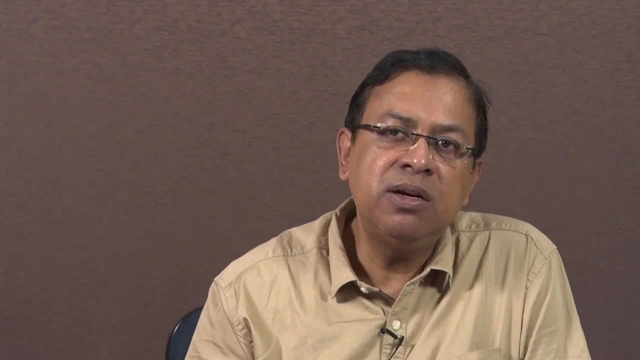 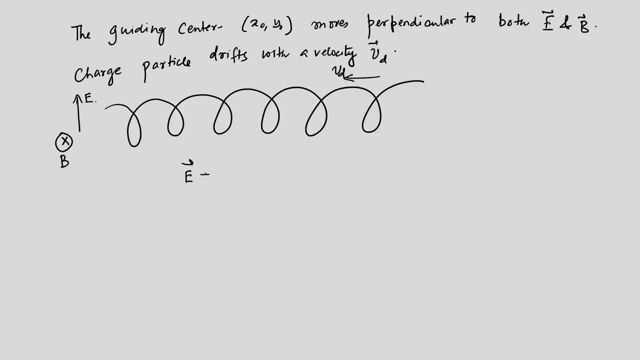 So how do we explain this drift velocity or what is the corresponding equation that it satisfies? the drift velocity satisfies this equation, which is V, D, cross, B, equal to 0. So this is: the net force is 0 and this is the equation that it would satisfy. 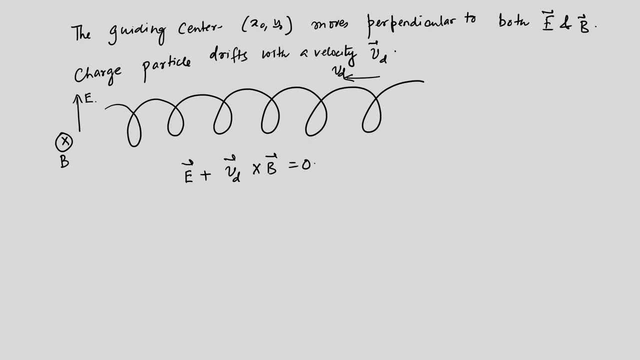 And defines this. V D is defined by this equation and so how do we get this so we can actually get, you can take a cross product with B, cross product with B. that gives you 0 equal to E cross B and V, V D, cross B cross B. I am sure you can. you have seen these kind of a cross product triple. 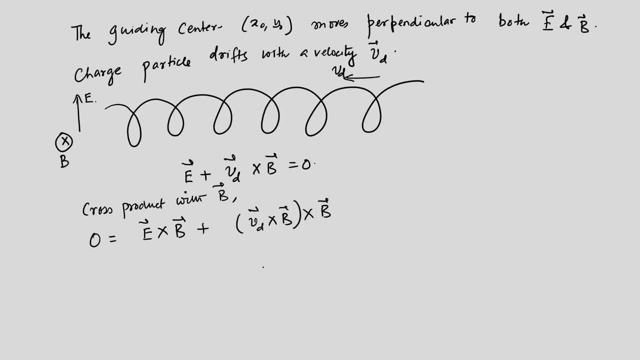 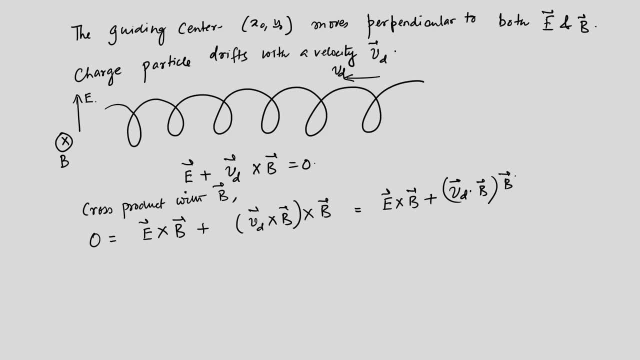 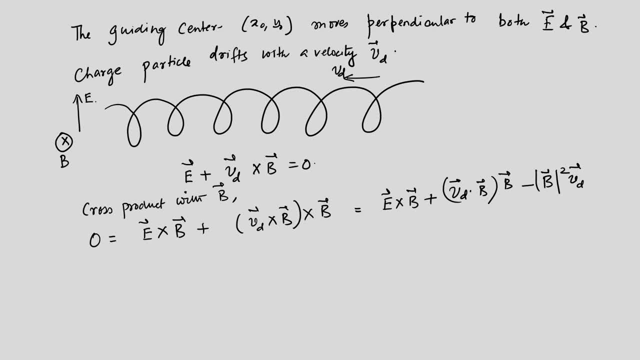 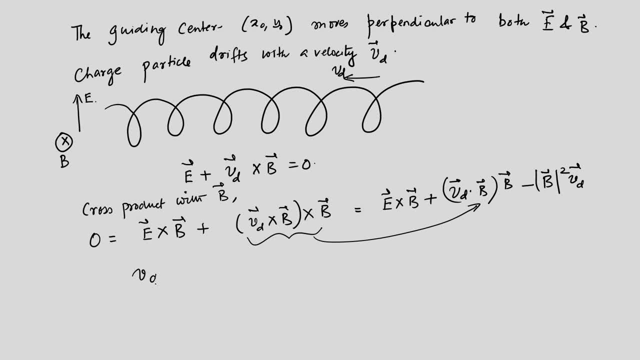 and then your V D becomes equal to E cross B divided by B square. ok, so B square. even write it with a square and a mod, but this also fine. So this is the drift velocity of the charged particle in presence of an electromagnetic. 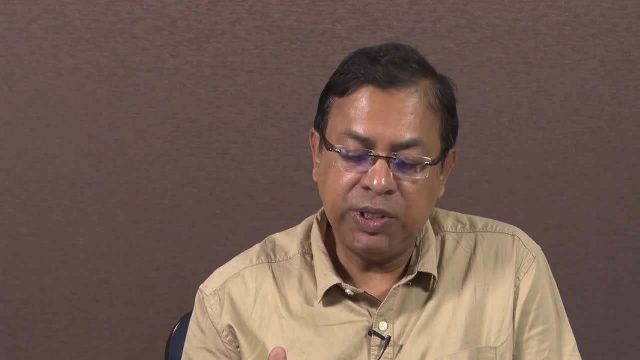 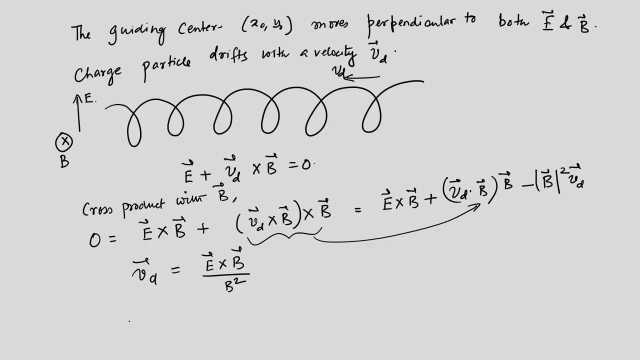 field where the electric and the magnetic fields are crossed with respect to each other, that is, their perpendicular with respect to each other. all right, So there is also another contribution to this velocity. in fact, this velocity is coming from even if there is no E term, that is, the electric field term. there will be a velocity due to the low range force. 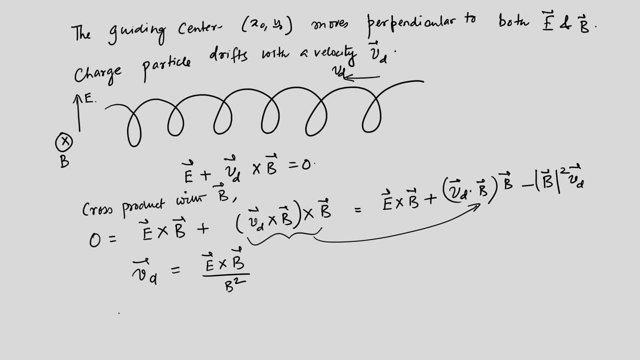 which is what we have seen earlier, and so this let us call it as VL, and this L stands for low range force, So let us call this as a low range velocity. and this low range velocity can be found out by taking a DDT of these orbit that we have talked about, and this is like exponential. 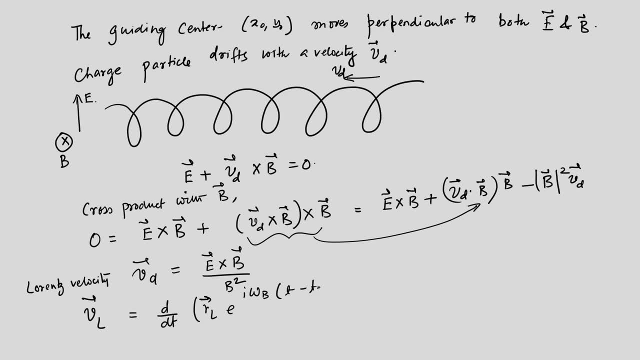 I omega B T minus some initial T0.. So this is purely because of the low range force, which is nothing but. so FL is nothing but QV cross B. So this is a low range velocity. this will get added to the drift velocity and the net velocity will become equal to. so it is a VL plus VD. 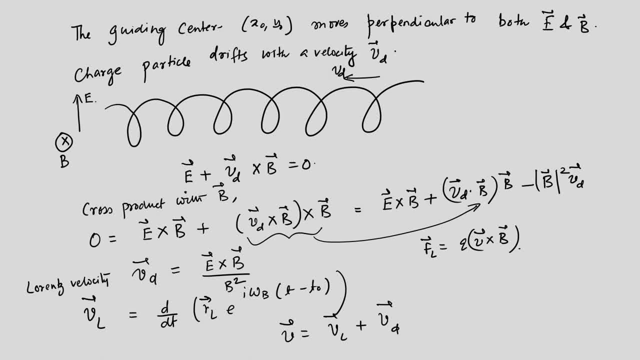 And of course, because of this, this electric field, there is also a velocity which will be there, which is the parallel component of the velocity, and this is the total velocity of the particle. and this total velocity can be integrated in order to find R as a function of T, and this is done in all books, classical electro dynamic books, and especially one can. 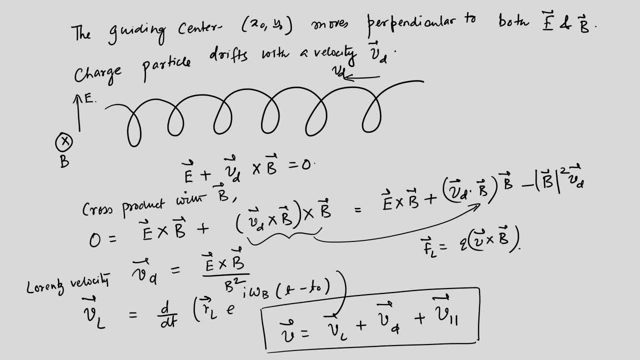 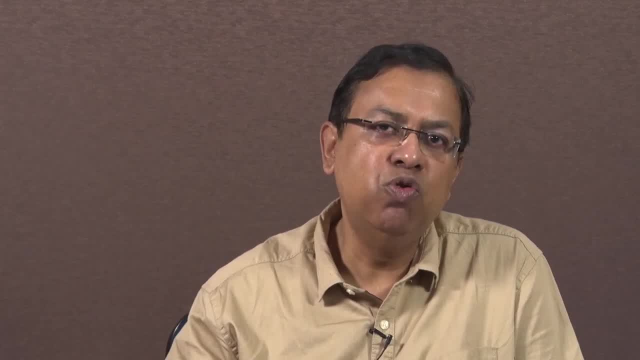 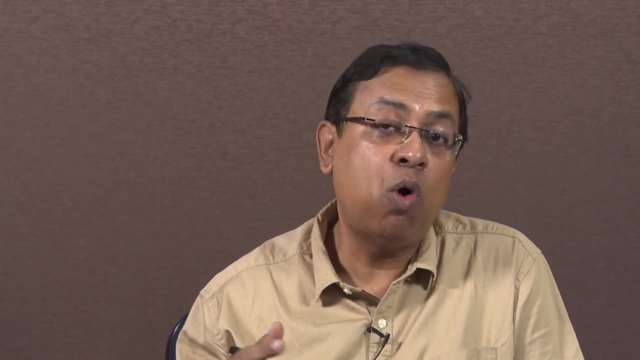 look at. So it is book on electro dynamics and it is nicely worked out there that it is actually a helix, a moving helix which you know sort of moves in a direction which is perpendicular to both E and B, and if you have non uniform B, that creates another complication and in 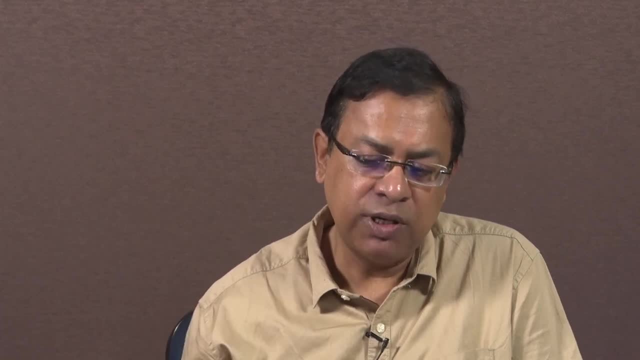 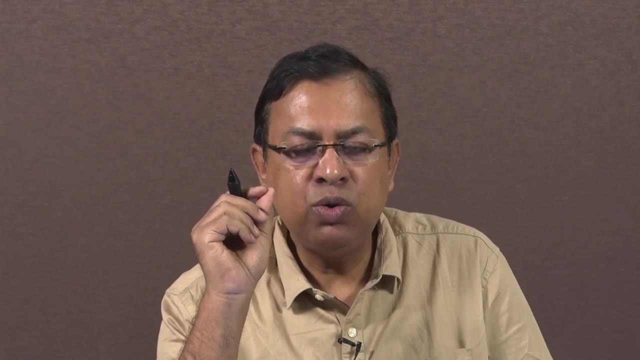 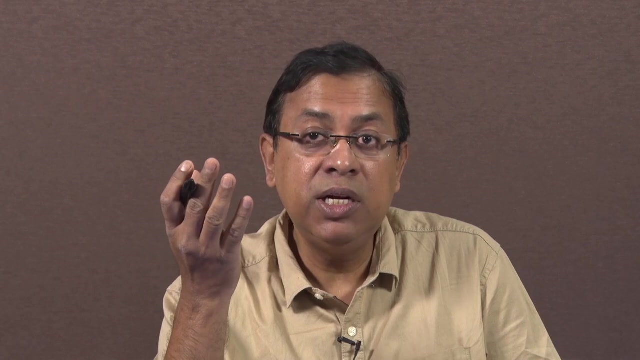 which may be, you will have. you know, the radius of the moving orbit changes, and so on. The reason that we have Discussed is that we needed to understand the trajectory of the charged particle, and we are really dealing with electrons in an electromagnetic field or in a magnetic field. 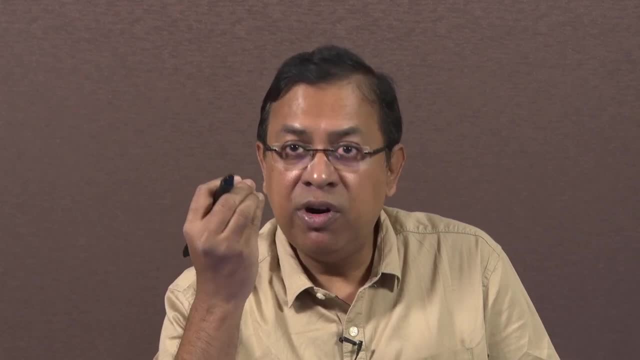 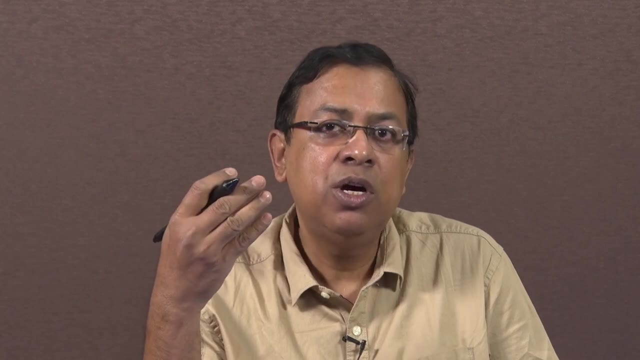 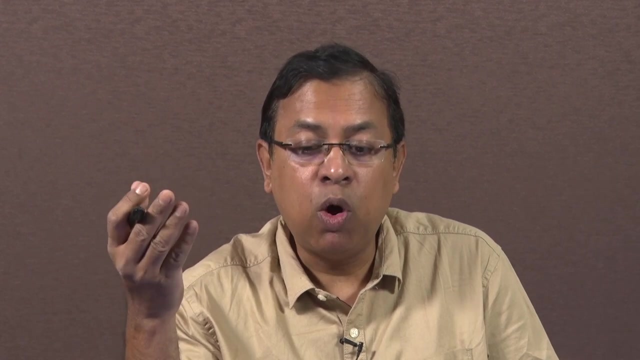 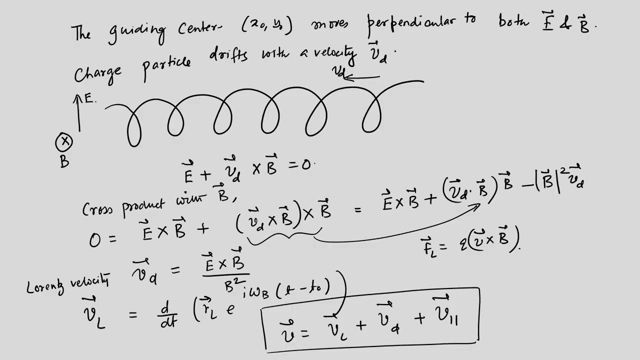 So, and these electrons are governed by laws of quantum mechanics and we will have to do a quantum mechanical treatment of this problem and the, finally, the problem would lead to giving us this quantum Hall effect, or the integer quantum Hall effect which I showed you even at the beginning of the discussion today. all right, 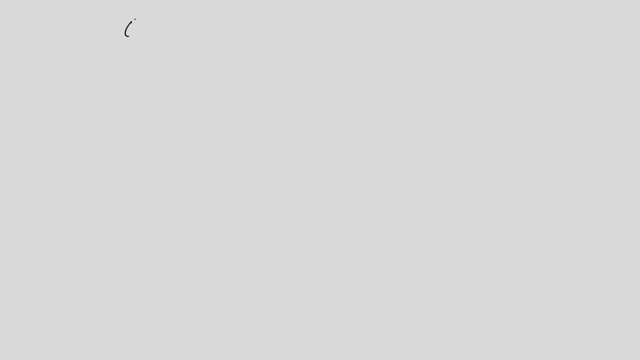 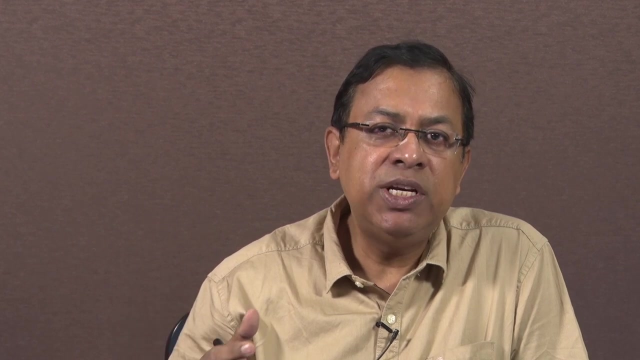 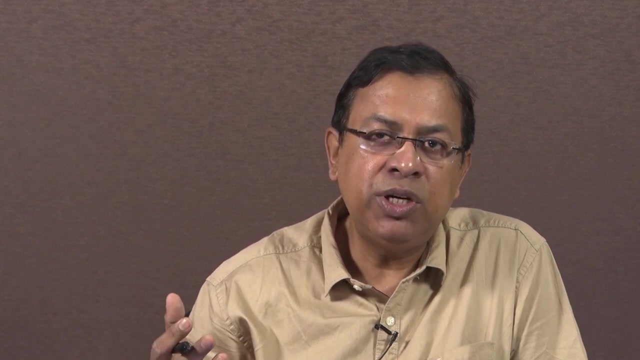 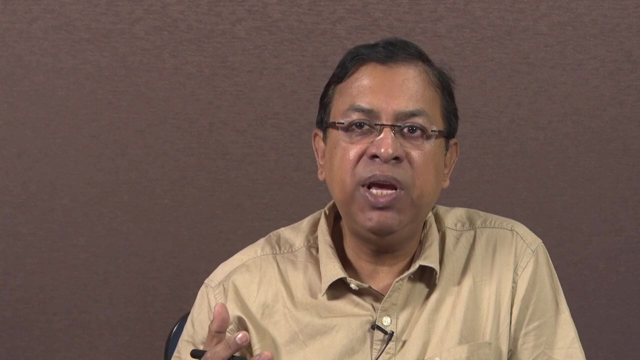 So let me sort of do a quantum mechanics now. this is of course a large number of electrons involved, but they are mostly semiconductors or metals that we are talking about and they have electrons which- the large number of electrons Being there, but still the inter particle interaction- can still be ignored. So you can talk about. 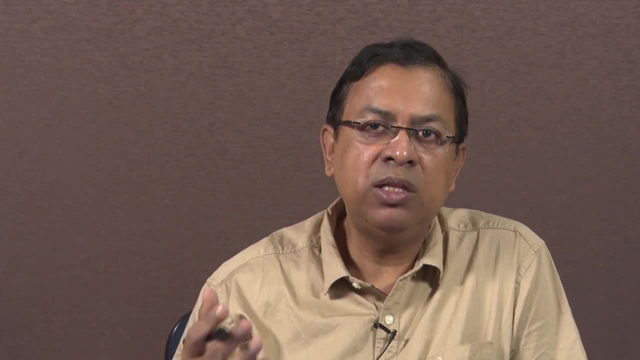 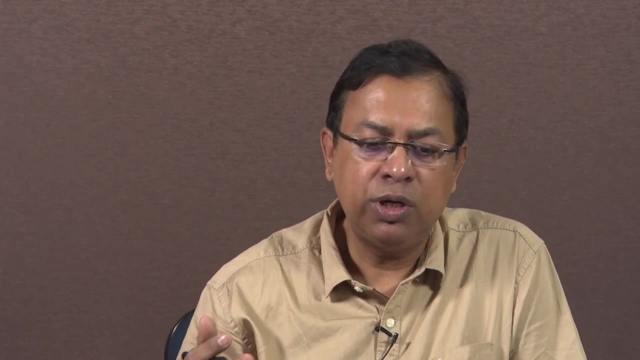 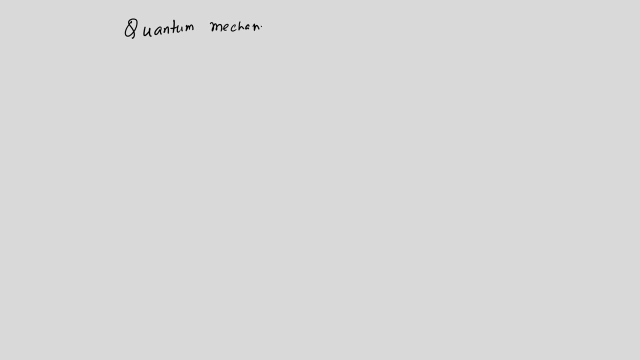 them as free electrons and, with the Drude theory, would explain their the conductivities and the resistivities as we have talked about. Let us write down a quantum mechanics of a charged particle, And first let us do it only for the magnetic field, and we will see that the physics is. 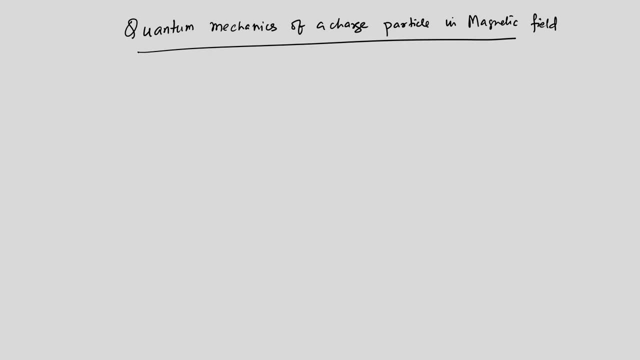 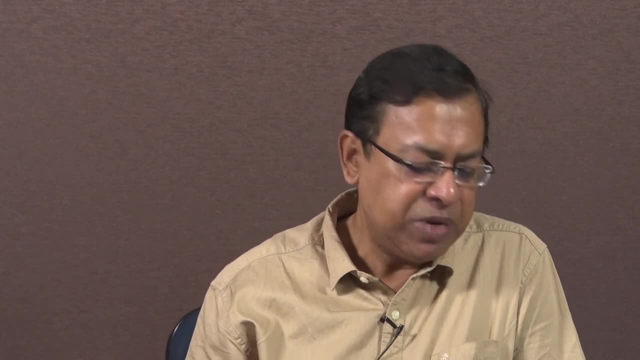 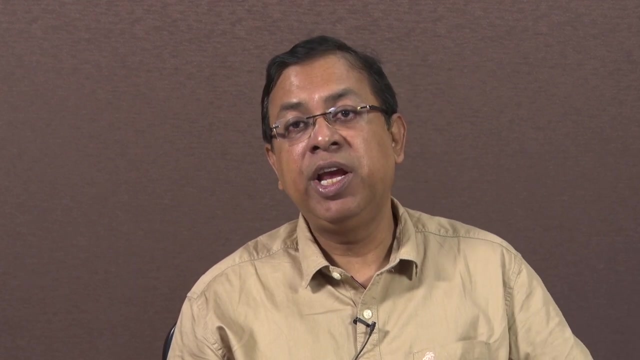 not radically altered when you include the electric field. there are some ramifications of that which will talk about. okay, And how do we do this problem, since we are talking about single charge particle, because the Electronic interactions can be neglected here. they are weakly interacting or they are not. 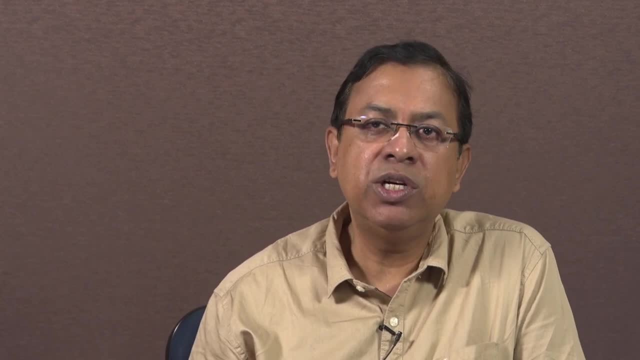 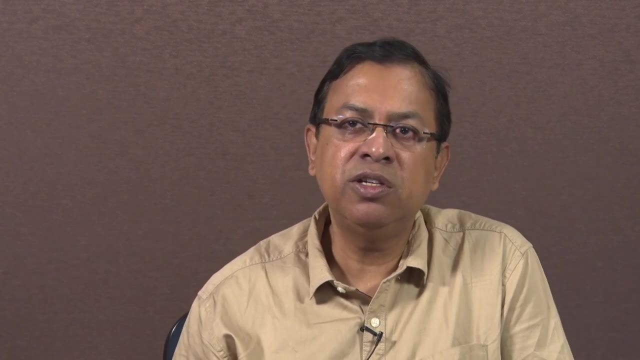 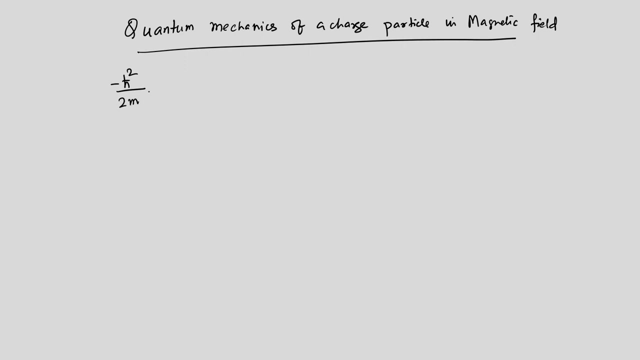 interacting at all. we can solve a Schrodinger equation in presence of a magnetic field. So how does one solve a Schrodinger equation in presence of a magnetic field? So let us write down the Schrodinger equation in its simplest form. it is minus h, square by 2 m. 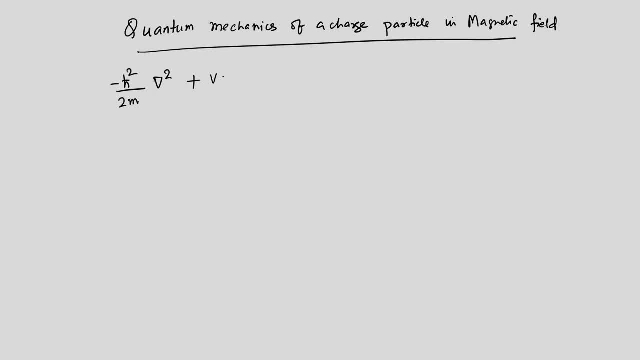 and del square, and a v of say r, And this r is: well, there is a psi here which is a function of r, and there is a function of r and this, if you write it the time independent Schrodinger equation, then this is a formula. 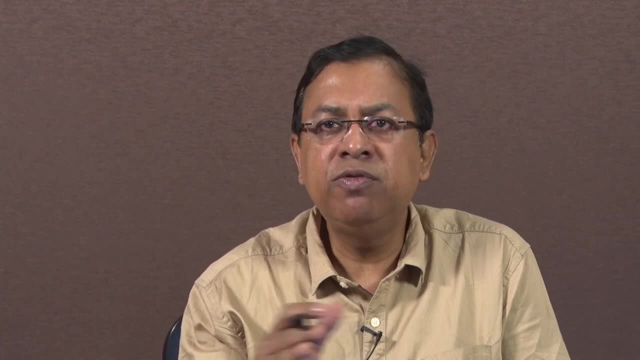 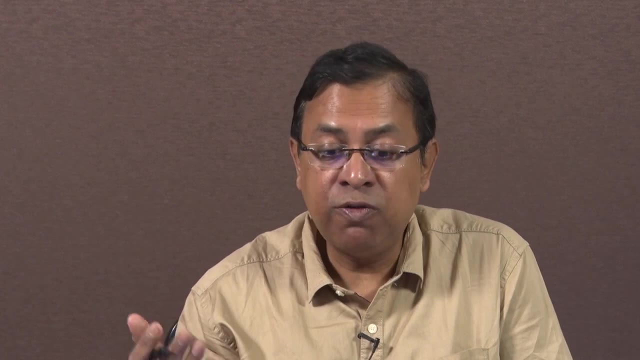 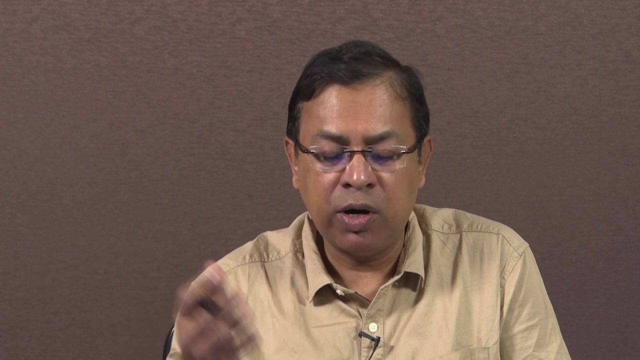 or rather, there is a equation that you need to solve- and you have solved it in a variety of situations in which you had, say, the particle in a box, say, for example, in which v r equal to 0. And it is equal to infinity. at the walls, or rather, outside the box, it is infinity. 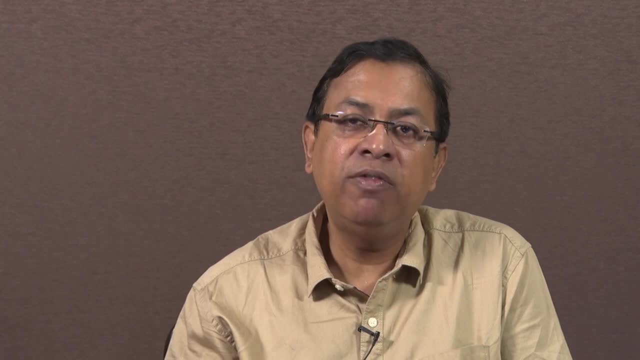 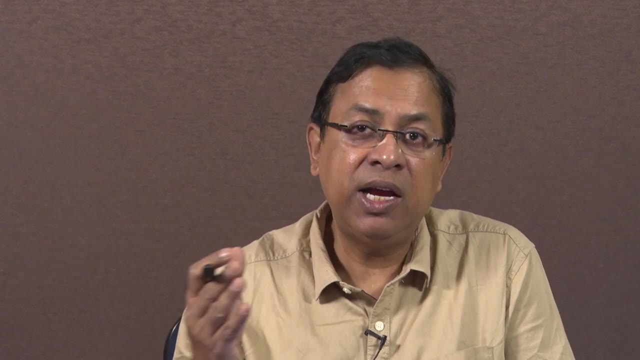 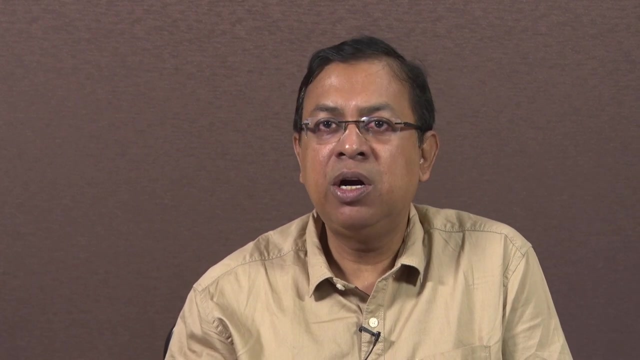 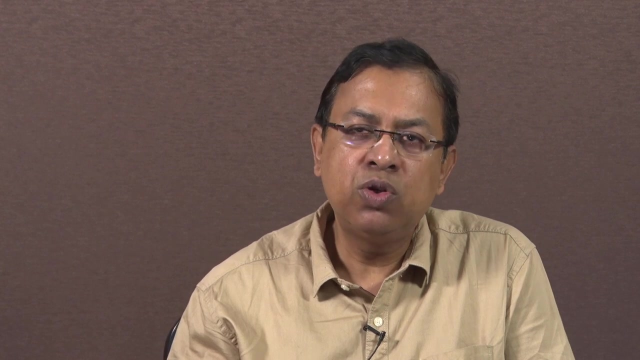 which means that the particle cannot escape, or you have done a problem in which these are finite steps, or their finite wells, or their finite barrier, or their infinite barriers, such as a delta function barrier, and so on, so forth, which are all part of the quantum mechanics course, first course on quantum mechanics that you have learnt. Now we are going to 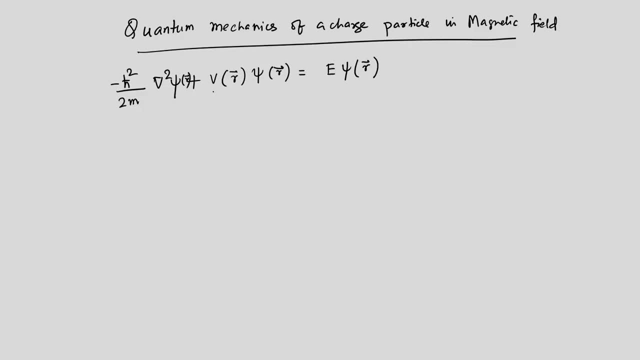 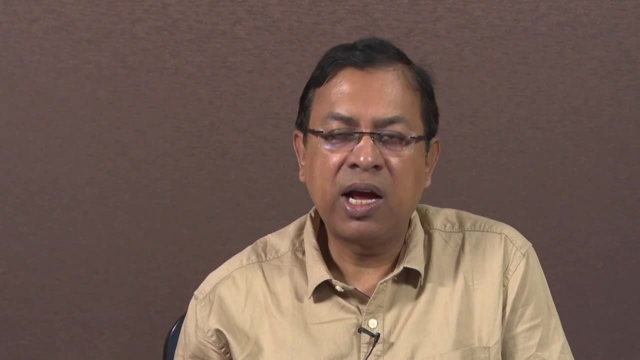 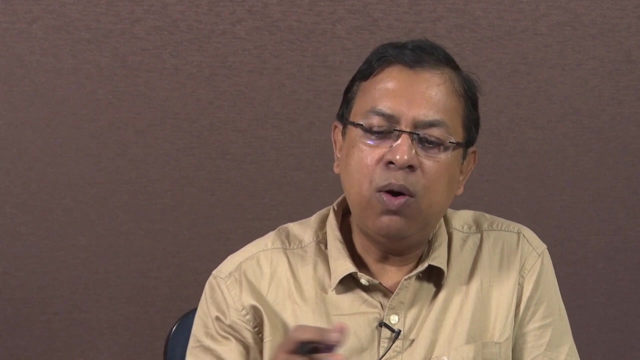 solve the same problem, and we are going to put this equal to 0 because we claim, rather assert, that there is no interaction that needed to be taken into account. even if it is there, it is very small and can be ignored. and now you have to somehow include the presence of 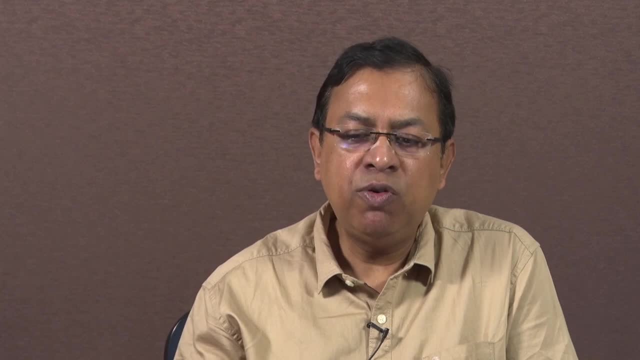 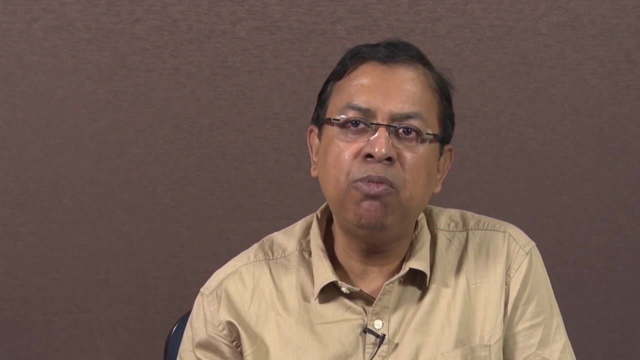 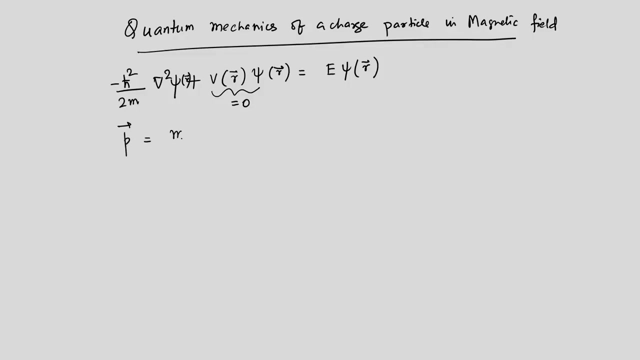 the magnetic field. okay, And if you remember that the magnetic field for a particle charge, particle that enters through the momentum, so the momentum which is written as P, which was without any magnetic field or any other thing, is equal to M into v, which is called as the mechanical momentum. This thing changes into presence of a magnetic field. 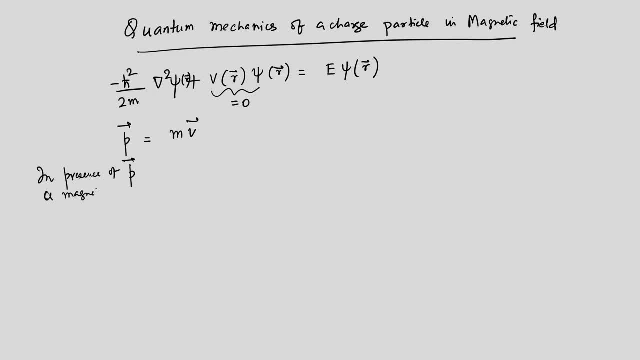 So this is P minus EA. so if this changes from P to P minus QA, where Q is the charge and A is the vector potential- and this vector potential is an important quantity and we know that the B actually is given by curl of A- okay, So this fixes the gauge Now. 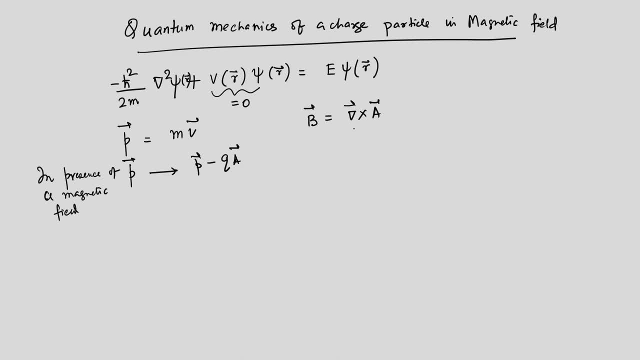 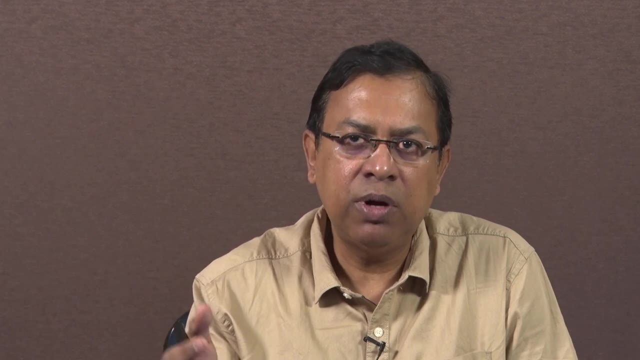 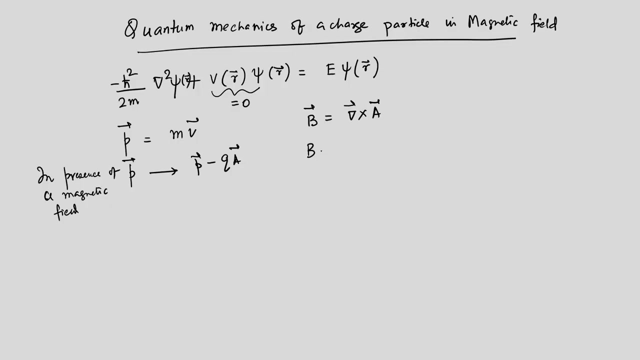 why I say a gauge? because you know, when B is perpendicular, that is, in the Z direction, then A can be either in the X direction or can be in the Y direction, or can be in any of X and Y direction. I mean it is in a direction which is perpendicular to the Z direction. okay, So say you have. 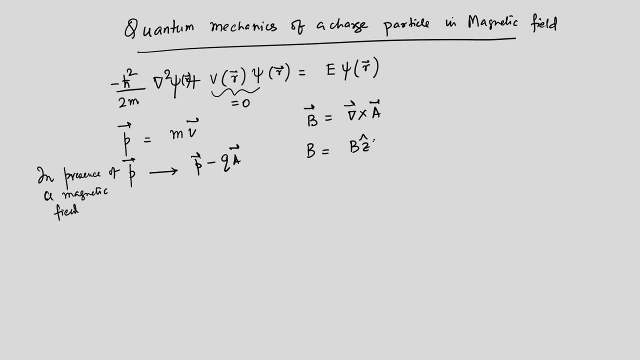 asserted that B is in the Z direction. okay, So the understanding is that we have a sort of planar charges, So there are charges here, okay, and which is, you know, a material like this, say, for example, a thin material, and there is a magnetic. 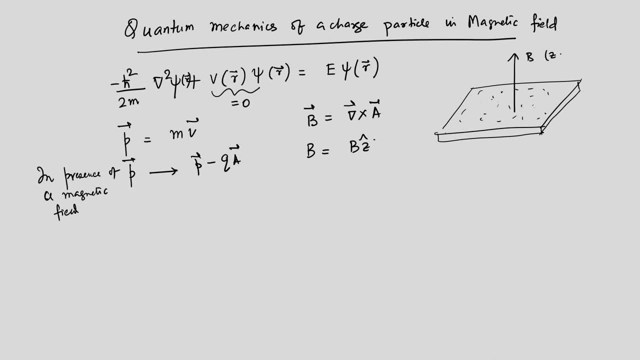 field which is perpendicular and acting in the Z direction. So this is the Z direction, all right, So B is equal to BZ cap. in that case A can be equal to, you know, minus BY- that is the X component- 0, 0,. it can also be 0, BX 0 and it can also be, you know, half equal to. 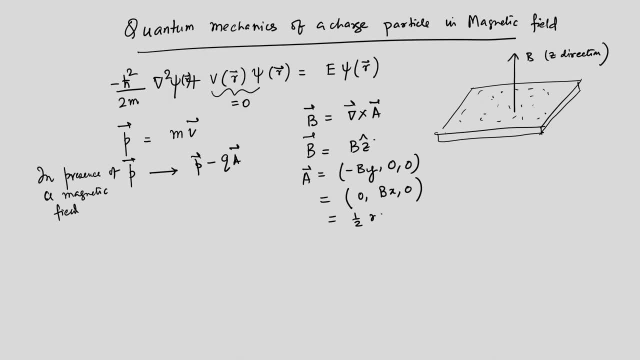 half R cross B, and this for a constant magnetic field. So this is equal to like BY by 2 minus BX, by 2 and 0, okay, So these are B into Y and B into X. okay, So all three forms of the vector potential would create the same B which. 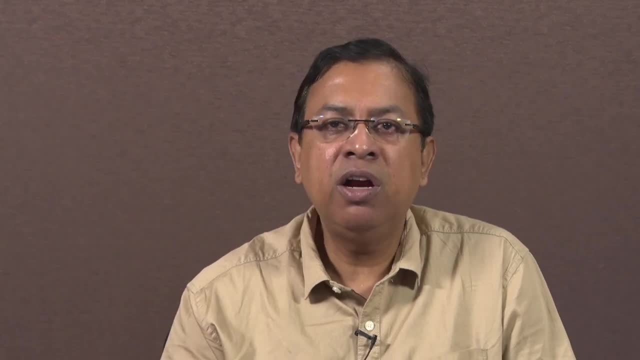 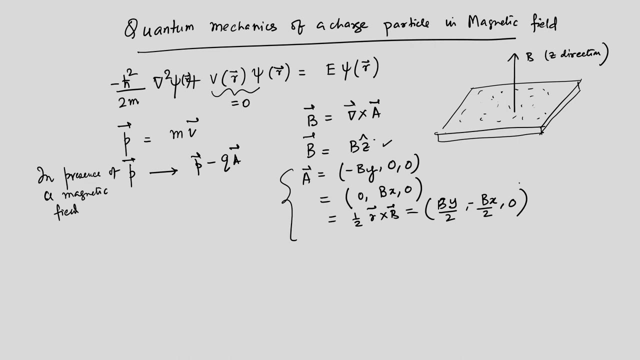 is in the, which is constant, and in the Z direction. You just have to convince yourself by taking the curl of this. and so these are called gauge freedom, you know? I mean in the sense that it, the final result, would not depend upon which A you use. okay, The A is also you can. 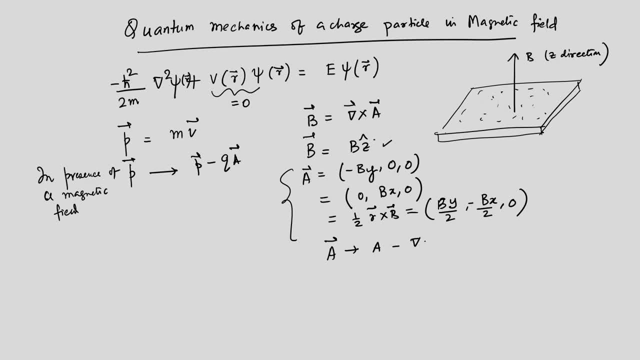 add or subtract, say. for example, you can add a gradient of a scalar quantity and see this. scalar quantity does not matter, because when you take a curl of this, a curl of a gradient would always be 0 and you can understand it in this particular fashion, that a gradient 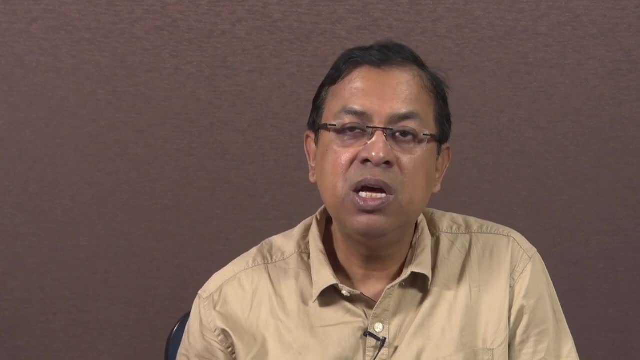 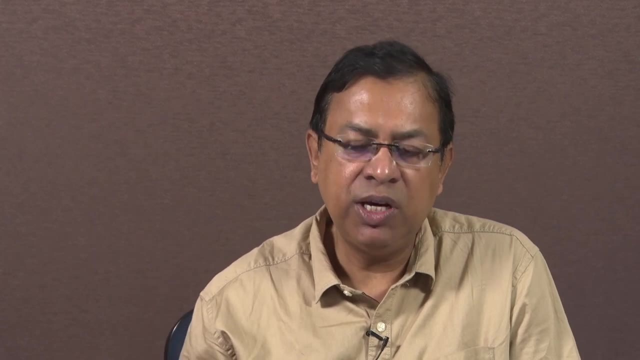 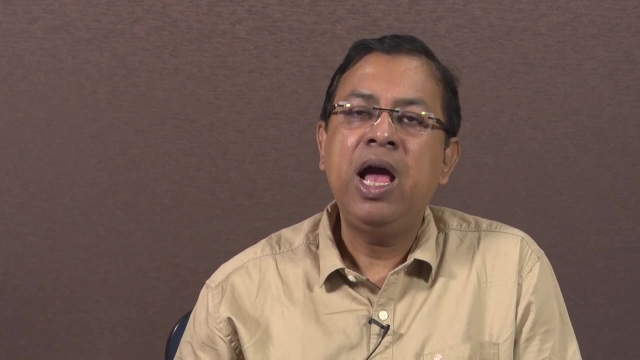 has a particular direction in space in which you ask this question, that if lambda is a scalar quantity, say it is like a heat density or something, or there is a sound wave that are or sound field that are produced because of some loudspeakers and so on, and they are 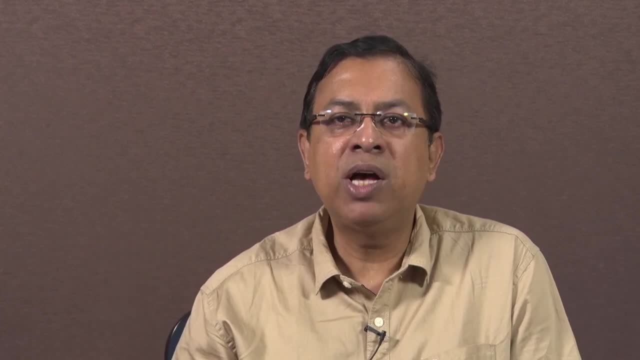 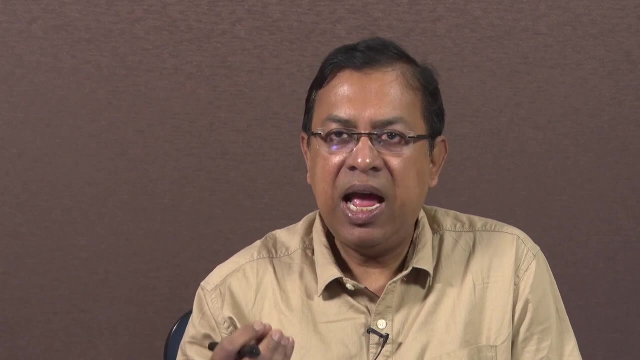 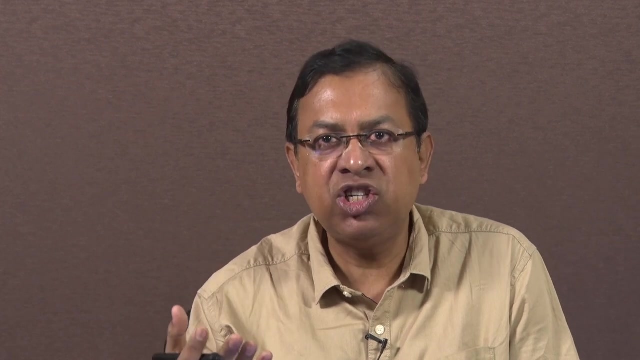 placed in four corners of the room and you may want to ask this question- that in which direction the sound intensity changes the fastest and in which case you have to find the gradient in which it changes the fastest. and the gradient is actually a direction and because it is a direction, if you take a curl of a particular direction, it has to give you. 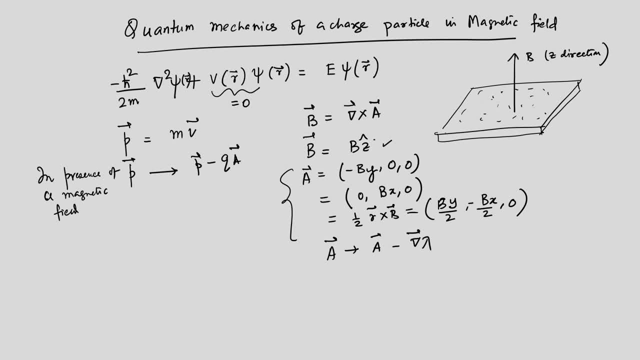 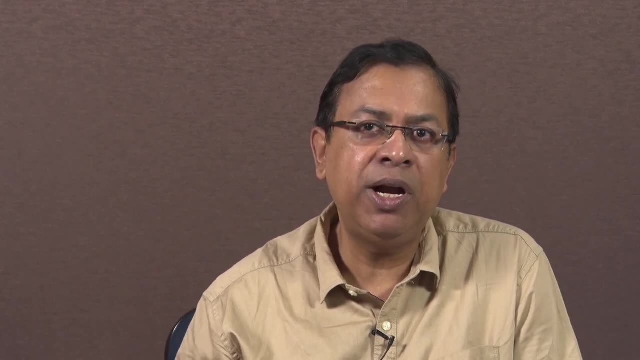 0.. So that is why there are these choices of a, along with this minus gradient of lambda, that these are called the gauge choices. finally, the results that you get are physical results, physical observables, So they would not depend upon which choice of a you have taken, or whether what choice 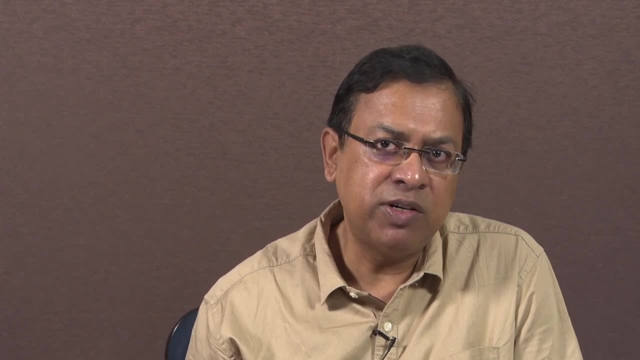 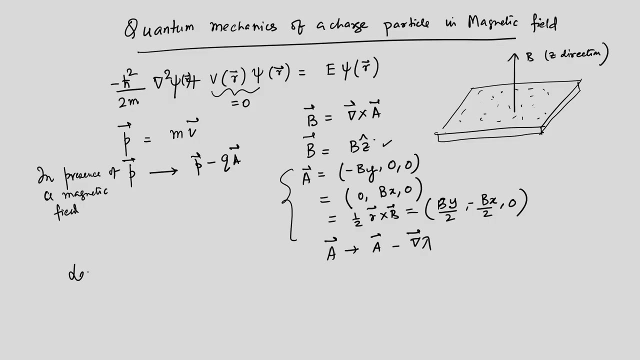 of lambda you have taken and it there is, a final result would not depend upon that, all right. So let us take this gauge, So let us fix the gauge to be equal to Ax. equal to that is the x component of A is minus. 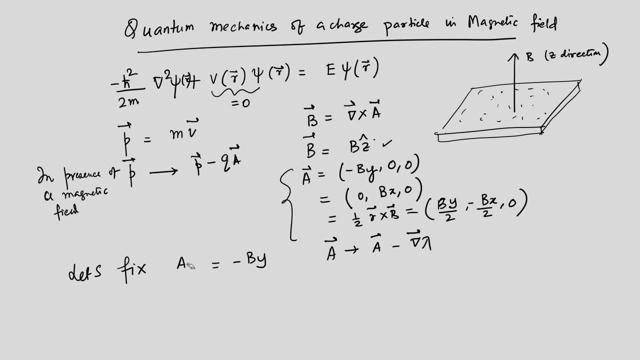 By. So A is equal to. so the first choice that we have talked about. let us take that, but it really does not matter. and this is called as a Landau gauge, Okay, Okay, So we do this and then put this in the Schrodinger equation and now make sure that your Q is: 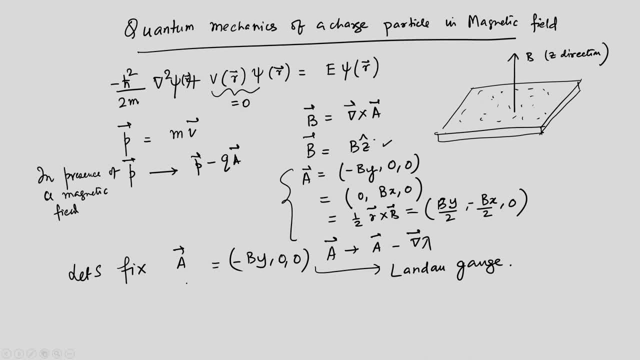 nothing but minus E, because we are talking about electrons specifically. So we will have this equation, which is 1 over 2 M, because it is a P square over 2 M. So we have a Px minus E by square, Okay. 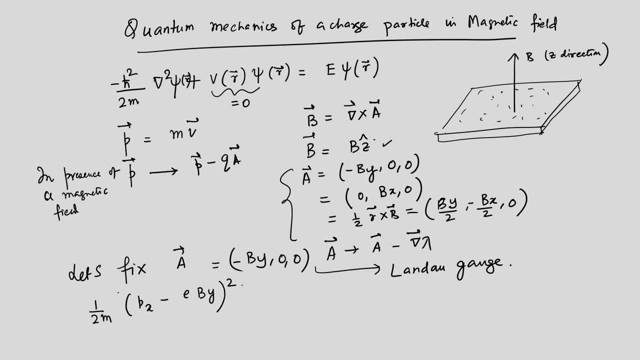 Okay, Okay, Okay, Okay. So we have a Px plus a Py square over 2 M and a plus Pz square over 2 M. you can actually put the 2 M outside. maybe let us do that So that I do not have to write these. okay, and this, the only thing. and then this psi. 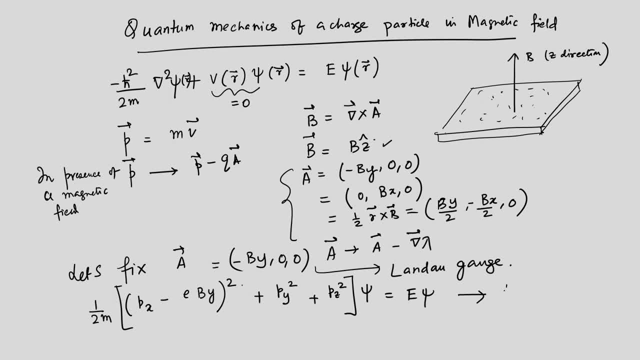 is equal to E. psi is the equation. So this is the Schrodinger equation. Okay, Okay, Okay, Okay, Okay, Okay, Okay, So this is the equation, So this is the equation, So the equation that you have to solve. 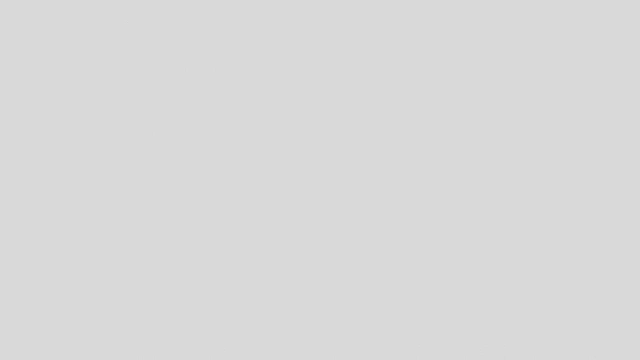 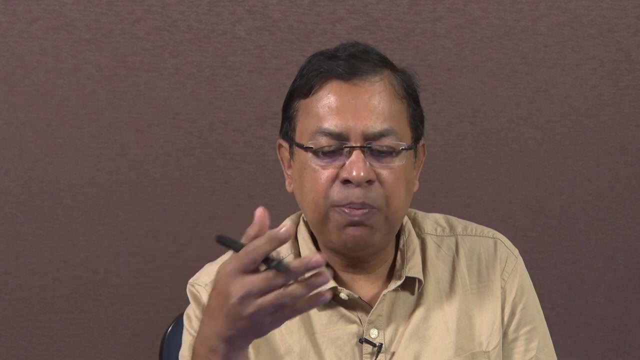 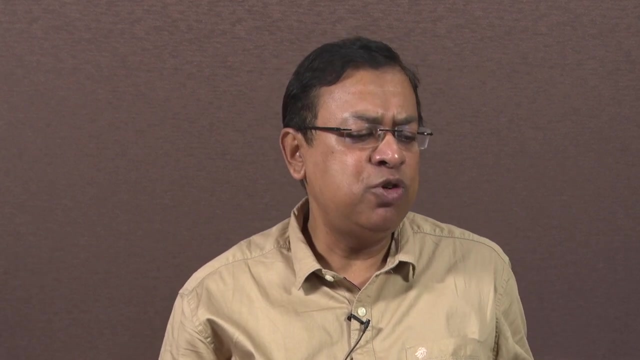 Okay, Now it is very clear that the motion in the z direction is exactly like a free particle, is just like a particle in a box, and that direction is quantized. and in fact it really does not matter if you are talking about perfectly two dimensional electron. the z component cannot. 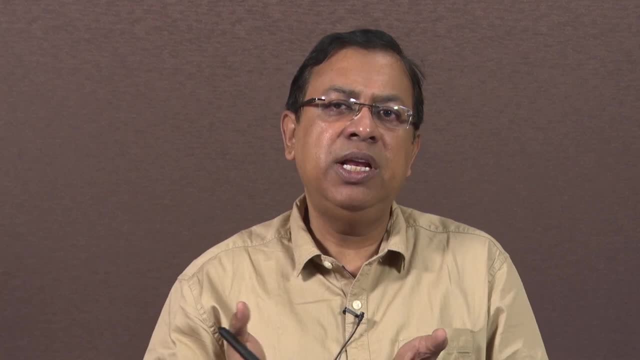 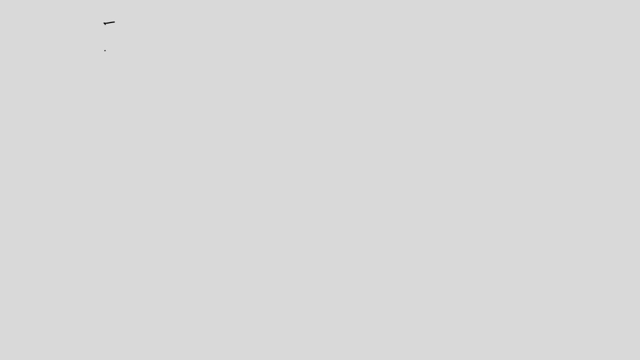 be there is there, it is quantized. So the electron cannot escape in the z direction because we are talking about a two dimensional problem. So that problem. then let us eliminate the z part of the kinetic energy, or this P z square over 2 m, and let us simply write it as like: 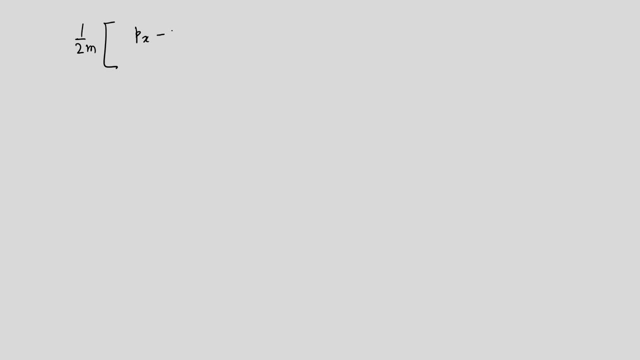 a 1 over 2 m, and then the P x minus e by whole square, plus a P- y square, and so on. Psi is equal to. now this psi is a function of x and y only, and this is equal to. let us talk about an energy. let us say that is denoted by epsilon: psi of x- y. I hope you understood. 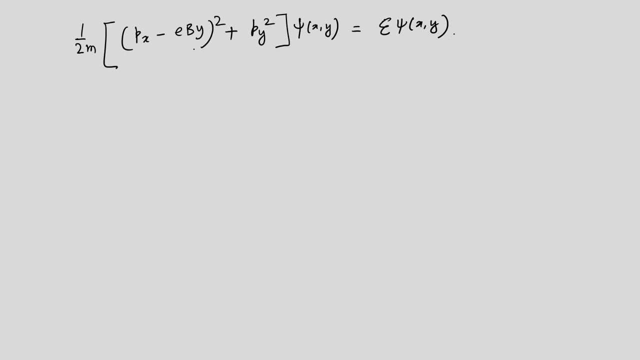 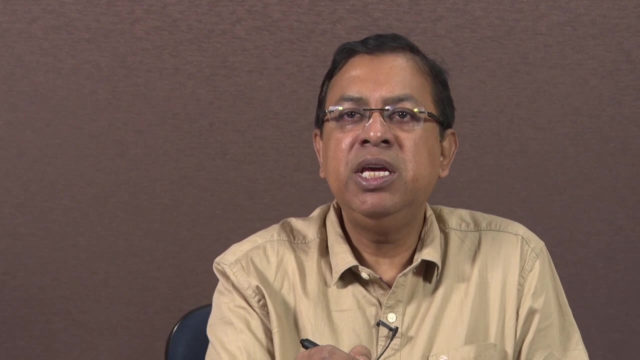 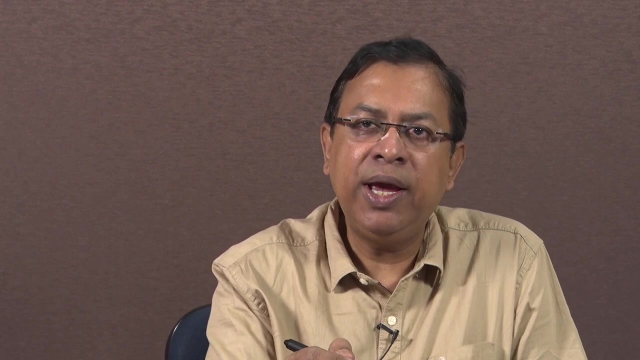 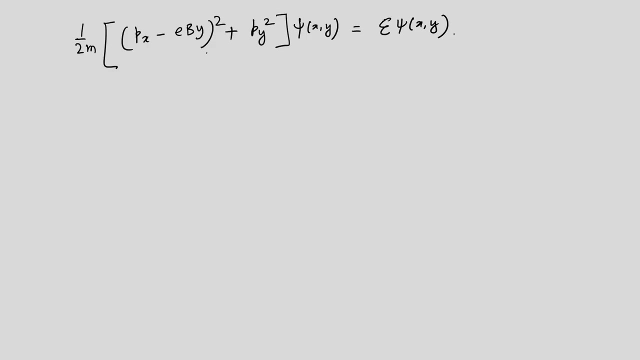 that px minus eby is written because the vector potential is assumed to be only present in the x direction. So it is p minus ea or p plus ea, rather because p minus qa, so p plus ea, that a has only x component. so only the px changes and nothing else. the py remains. 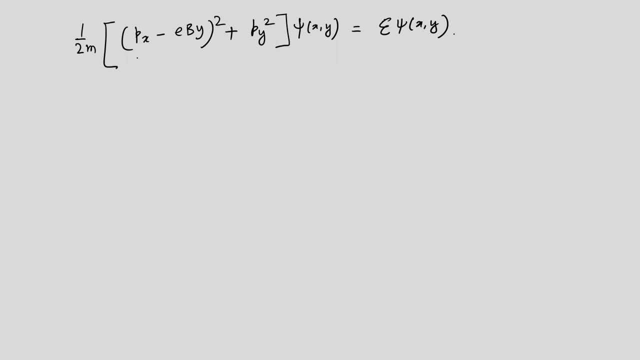 as it is okay. Now, this is, of course, a two-dimensional Hamiltonian. you can call it some hxy. so if you write it symbolically, it is like hxy, psi xy, equal to epsilon psi xy, and this is what you have to solve for. So you have to solve for the eigen solutions and the eigen solutions. 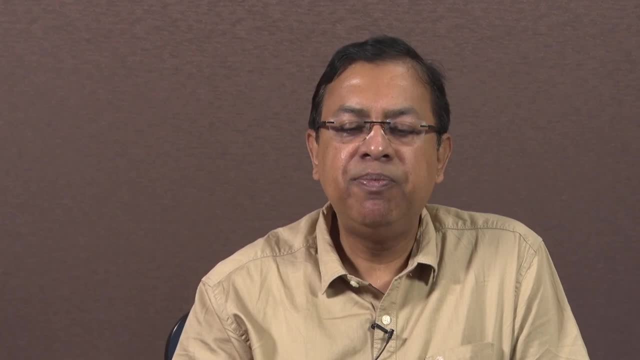 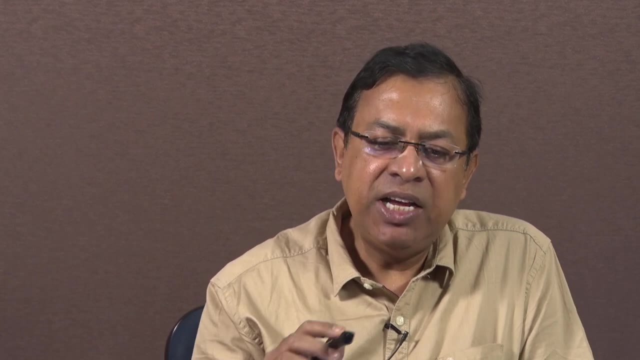 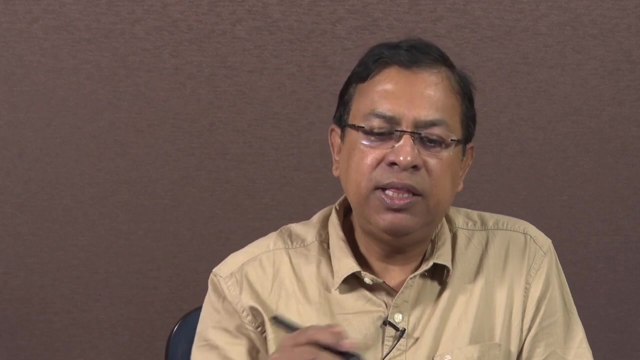 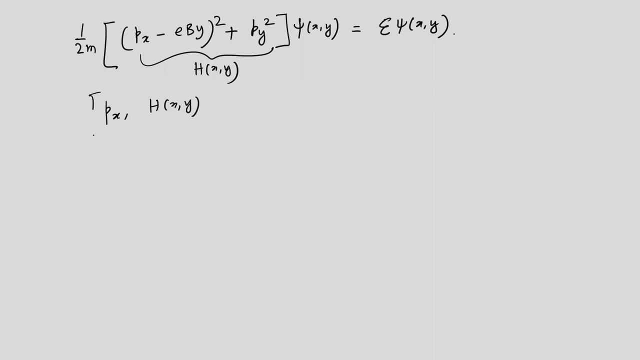 are nothing but the psi, xy and the energies are epsilon, are the two things then one has to solve, for There is something interesting that happens here. if you want to ask that which component of the momentum is conserved, then it is easy to see that this px and hxy is conserved, and 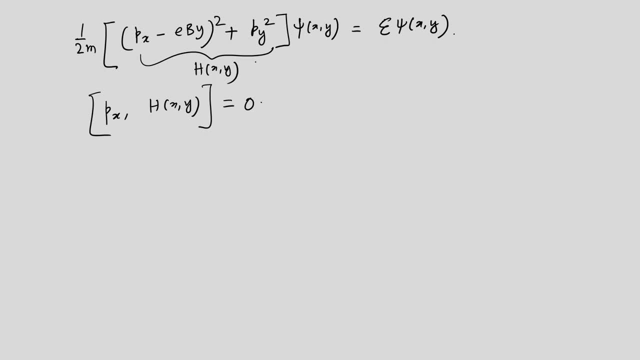 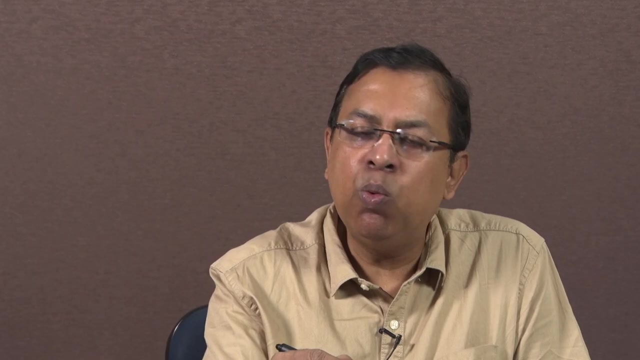 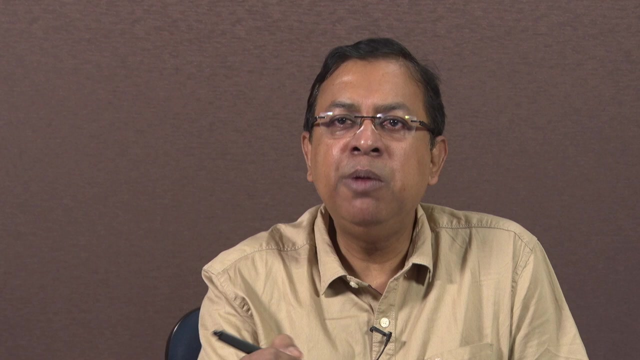 the reason is that there is no x variable here. Had there been an x variable, then there would be no commutation between px and h, but because we have decided to take the vector potential in the in the x direction and with a by. that is why it, this px is, commutes with the Hamiltonian and from elementary quantum mechanics, as you. 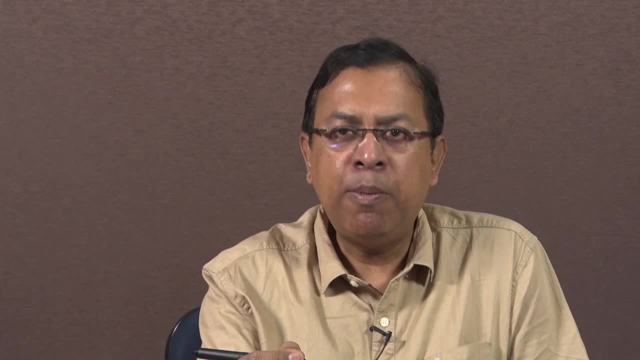 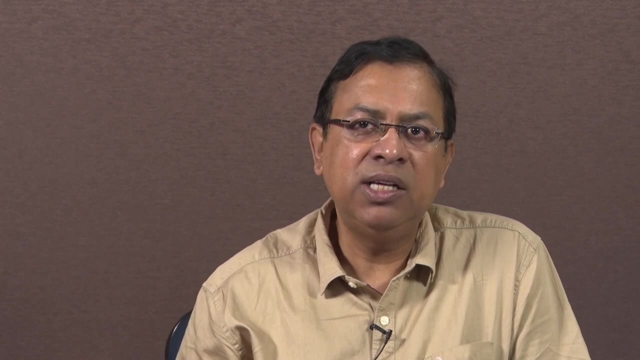 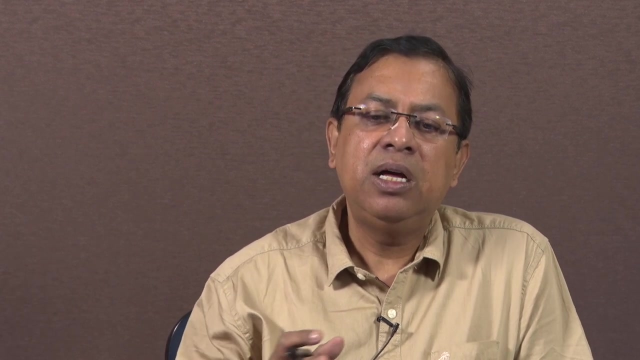 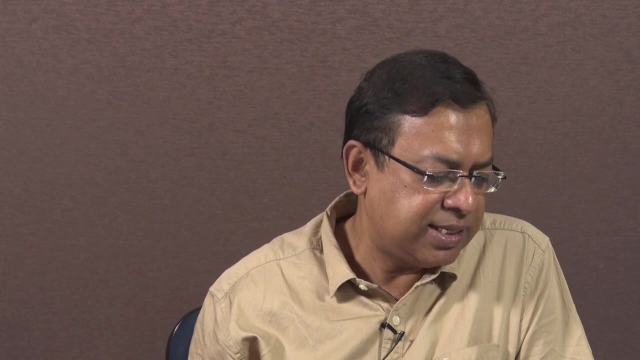 know that if an operator commutes with the Hamiltonian, then the corresponding quantum number remains conserved, or there are quantities that remain conserved here. of course, the px, that is, the x component of the momentum, remains conserved, and the quantum number or the sort of quantity that remains conserved is called as a kx. ok, So kx is h, cross kx, so px is equal. 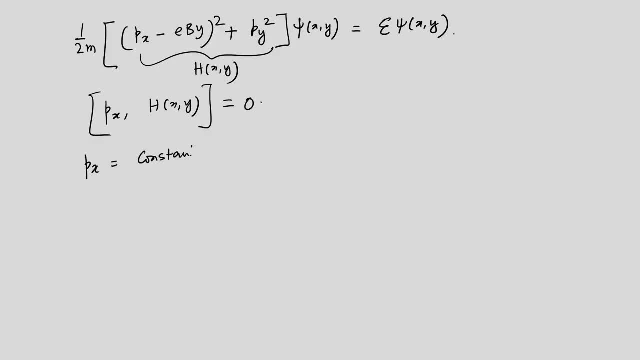 to constant, which tells you that h cross kx is equal to constant. ok, So h cross kx is constant. So this kx, because we are talking about a quantum mechanical problem, this kx is quantized as 2 pi over, you know, nx divided by lx. ok, It is just that, just the way we have learned. 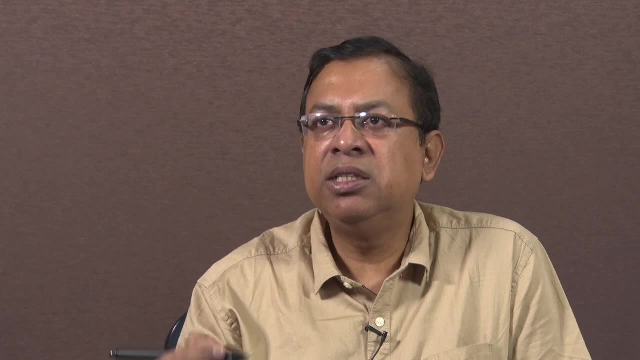 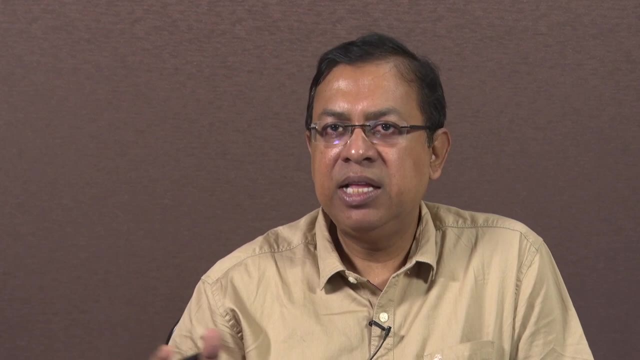 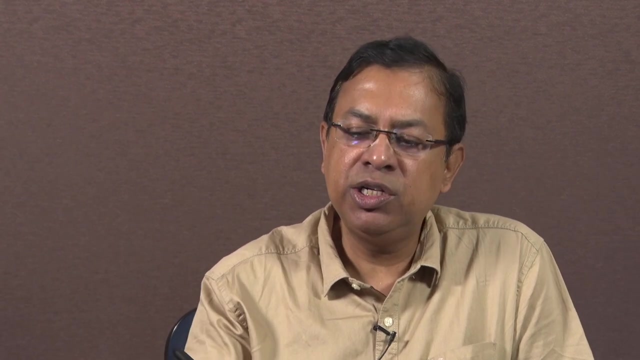 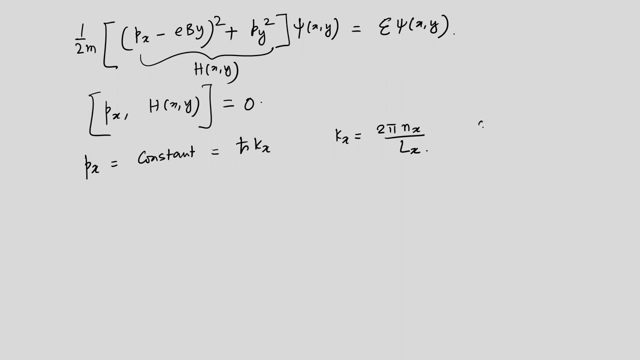 that particle in a box, the k vectors are quantized. the k vectors are quantized because of the presence of boundaries there And that is, we have seen that k equal to you know, n pi over l. here, because of the periodic boundary condition, you get a factor of 2.. So this kx is equal to 2 pi nx by lx and nx. 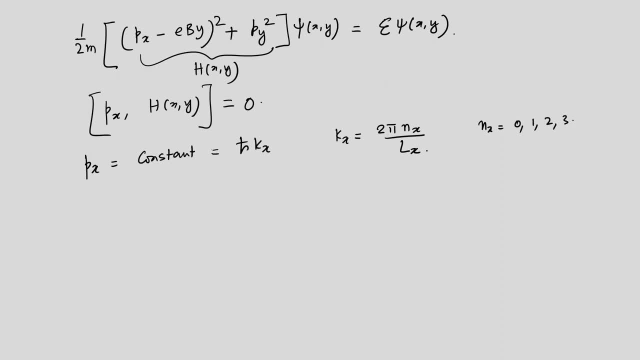 are 0,, 1,, 2,, 3 and so on. ok, So these are the values that are. sorry, 0 can be neglected, because 0 means that the particle is not there. So it is. it is actually 1,, 2,, 3 and so on. 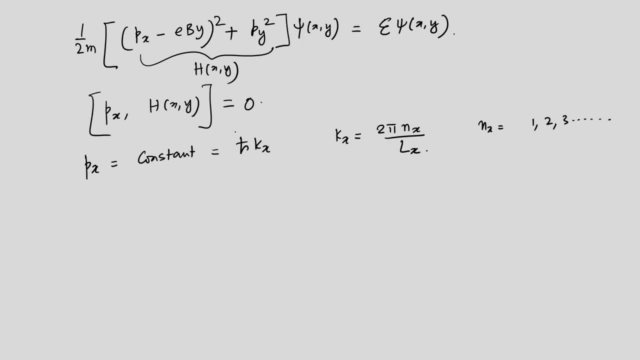 Ok, So any integer, The rest of the relation can be written as: so: if px is a constant, I can absorb it as a constant in the Hamiltonian and can write down the resultant Schrodinger equation as follows: ok, So this is equal to p y square over 2 m. p y is not conserved. 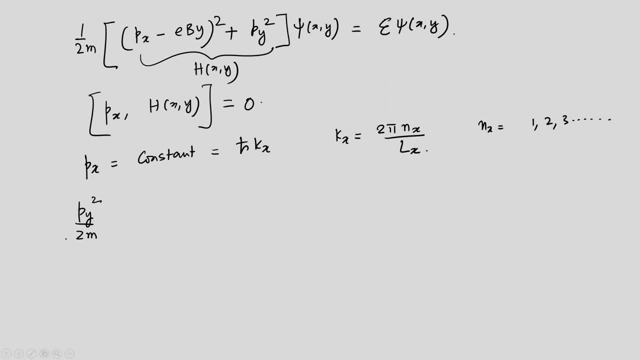 for the reason there is a y in the Hamiltonian and p? y and y do not commute. This is the uncertainty principle that you have learned, and particularly y and p? y is equal to ih cross. ok, This reason that p? y is not constant, and I can write down then this 1 by 2 there: 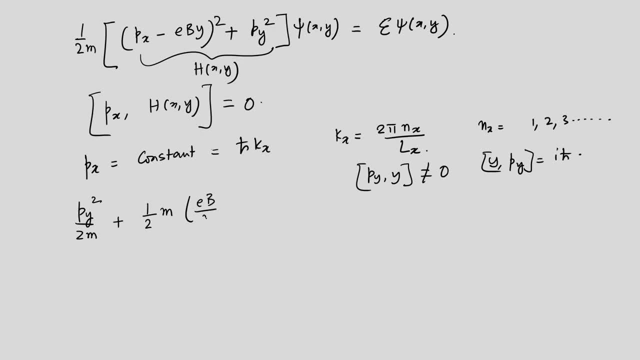 is half m and E b over m square and y minus y0 square, And now my wave force is going to function- actually becomes function of only one variable, that is y, because you see there is no x anywhere in the Hamiltonian, So I can write this as simply f of y and this is: 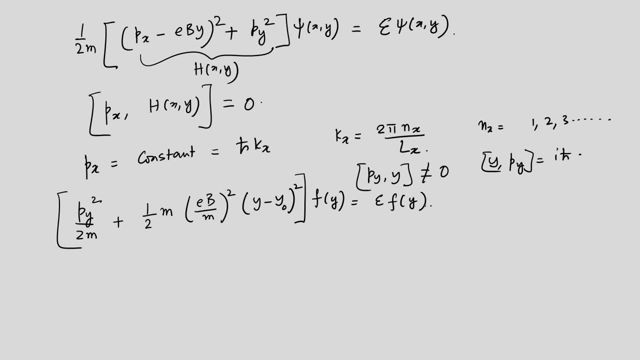 equal to epsilon and f of y. okay, and what is the y 0,? y 0 is the constant thing, which is p x over e b, and this p x is the x component of the momentum, which is argued that y is constant and, of course, for a given problem, e and b are constants. b is the uniform field. 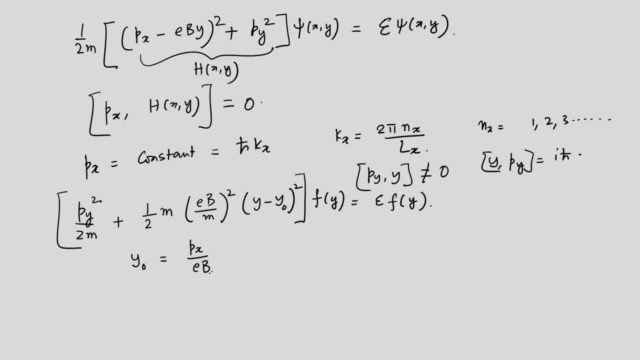 So this y 0 is actually p x by e, b, and this is. it has a name called as a magnetic length and written as l b because it depends on b, So we can write this as simply f of x, and this is the x component of the momentum which. 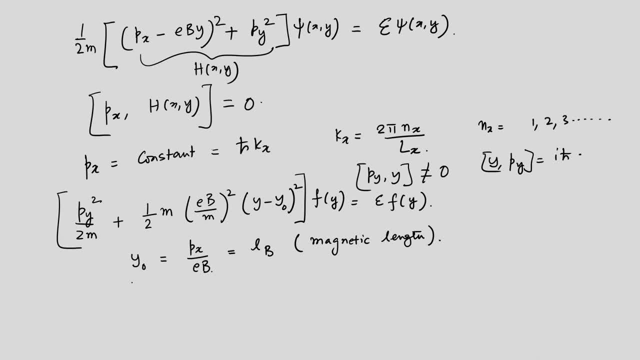 Okay, now this tells you that if this is a constant, there is a p y square and then there is a half something m into some cyclotron frequency, So it is a half m omega square, and then y minus y 0 square, and then you have this wave function, which is only a function. 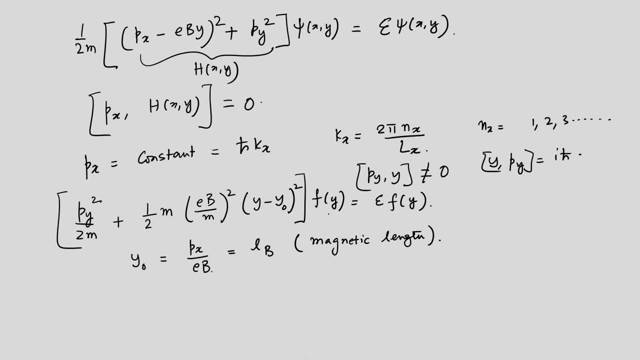 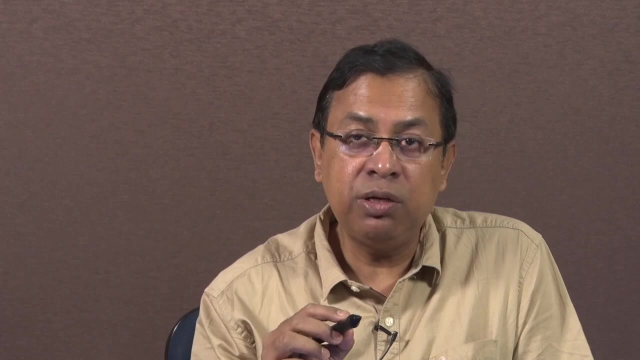 of y, and that is why from psi x, y we have written in f of y and then energy into f of y, and this clearly represents that the equation for, or the Schrodinger equation for a harmonic oscillator oscillating in the y direction, about, not about 0, but about this y 0 or the 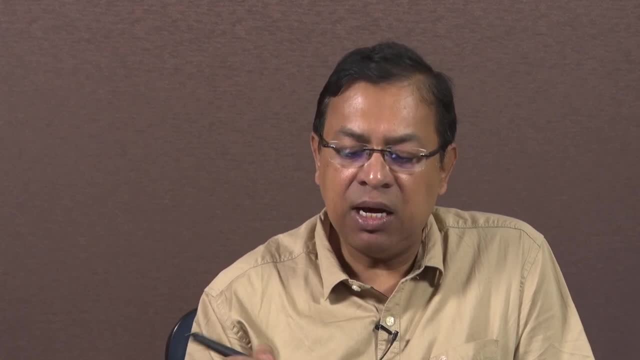 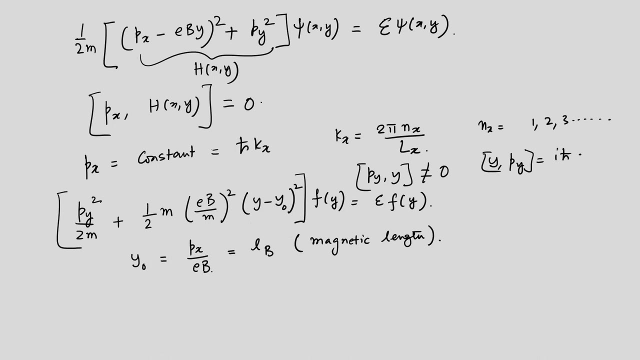 magnetic length which is given by this p x over e b. okay, So if it is a harmonic oscillator problem, then we do not need to solve any further. We can Get this, the solution to be exactly of the form which is epsilon equal to n plus half. 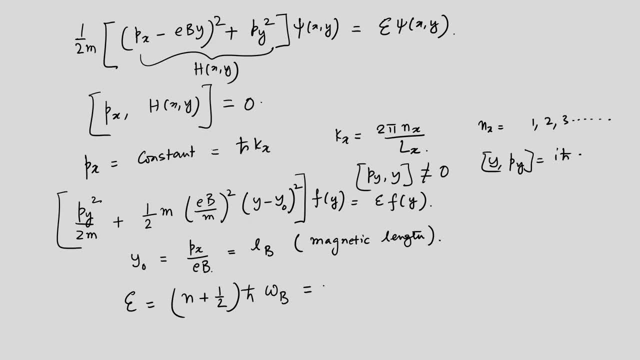 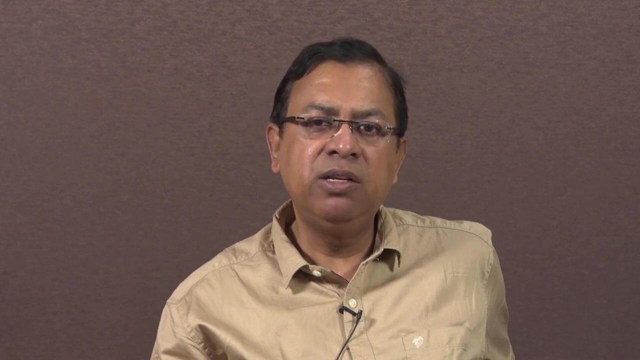 h cross omega b, where omega b is equal to. of course, omega b is equal to e b over m, which we have said several times that this is equal to the cyclotron frequency. okay, So a problem which was Simple enough to begin with. we find the solution, at least till now we have found the energy. 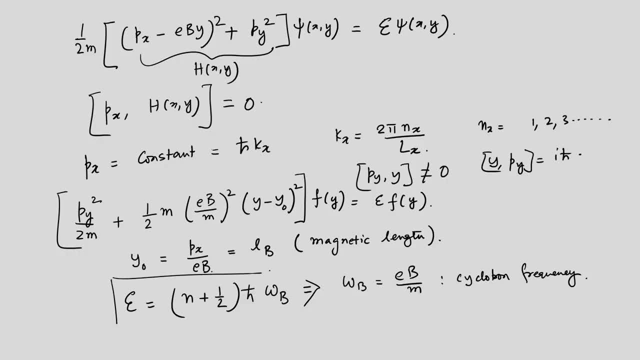 So the energy is nothing, but it is n plus half h, cross, omega, b, just following the solution for the energy. for a harmonic oscillator, n can have 0,, 1,, 2,, 3,, etc. all the integers, and here it can be equal to 0 because the harmonic oscillator allows for a solution with. 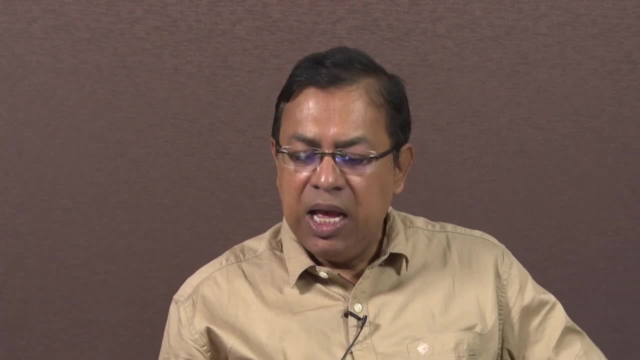 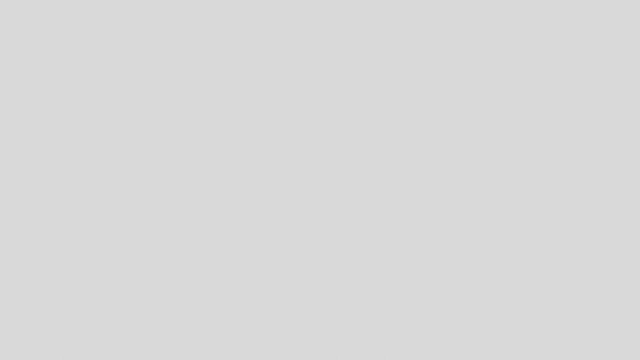 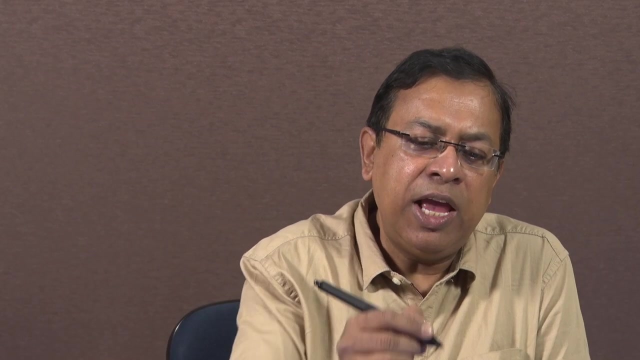 a quantum number n equal to 0.. Okay, So this is the energy, or the Eigen values of the problem. Let us see the Eigen function. So the Eigen function, now let us call it, because we can solve for, of course, f of y, that is. 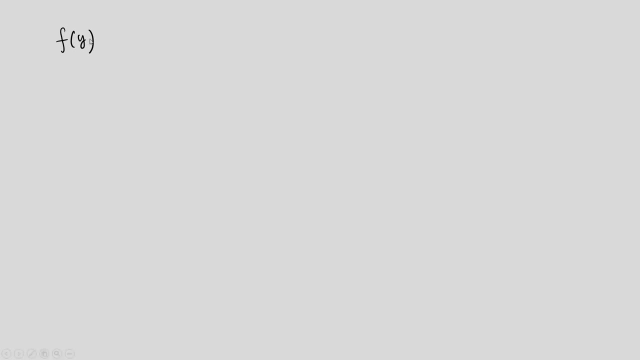 what we will do. but then we know that the total wave function, which is equal to f of or psi of x- y, psi of x- y- is actually A free particle in the x direction multiplied by this f of y. okay, This is the total wave. 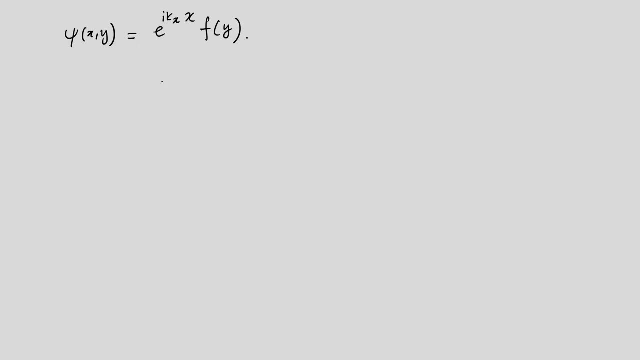 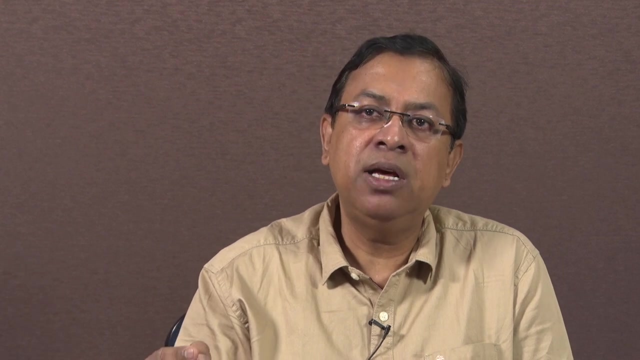 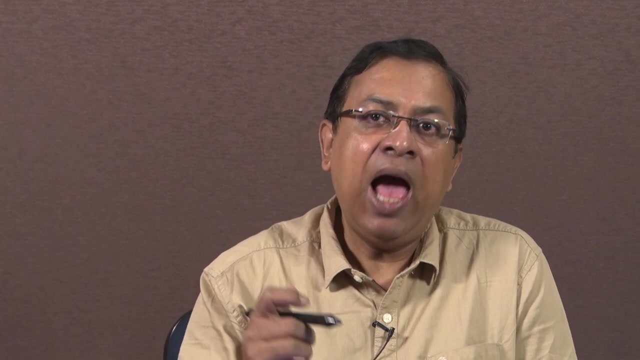 function for the planar motion of the electron that is, in the x direction. if you take this as the x direction, it propagates like a free particle because p- x is constant or k- x is constant. So it will propagate like a free wave there and will have a harmonic motion. 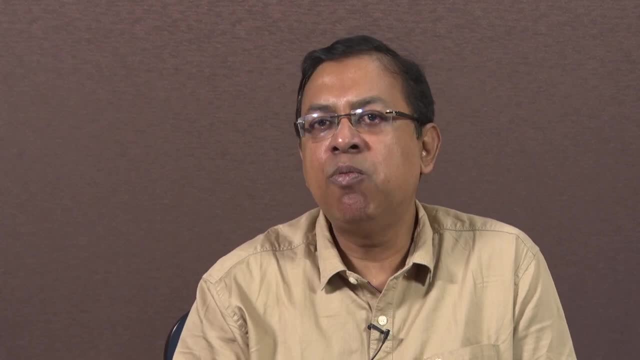 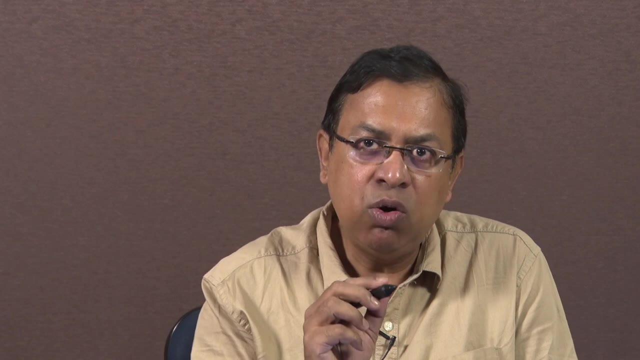 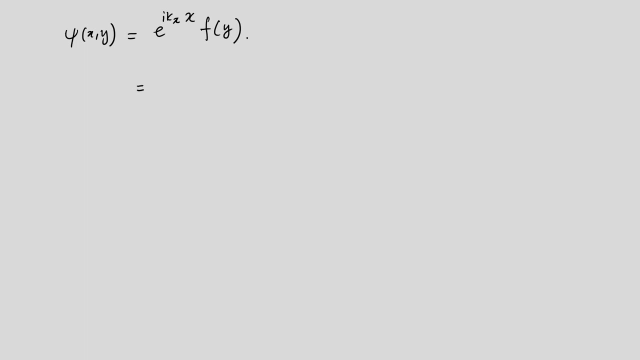 in the y direction. So in the y direction it will have a harmonic motion, will make a execute a harmonic motion about a point which is given by y 0, and this y 0 inversely depend upon b. okay, So this is nothing, but I use a normalization for the x direction box normalization. this is equal. 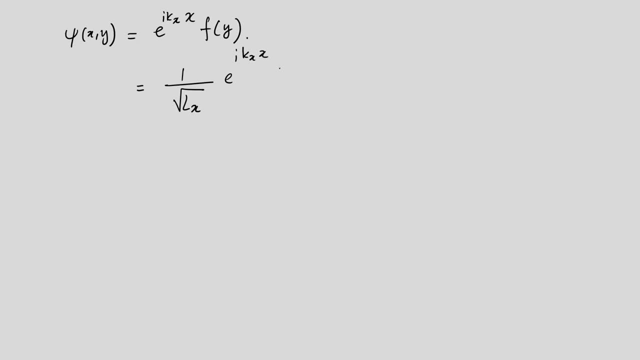 to exponential i, k, x, x. and now I do not try to normalize. it Is not, you know, required here. I use this as normalization constant and use this okay. So let me write the normalization not with the capital N, because you have a small n. 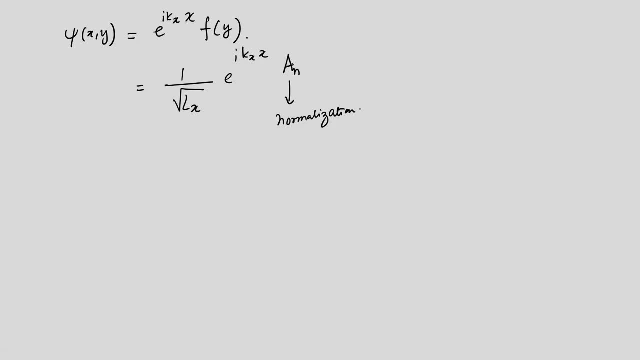 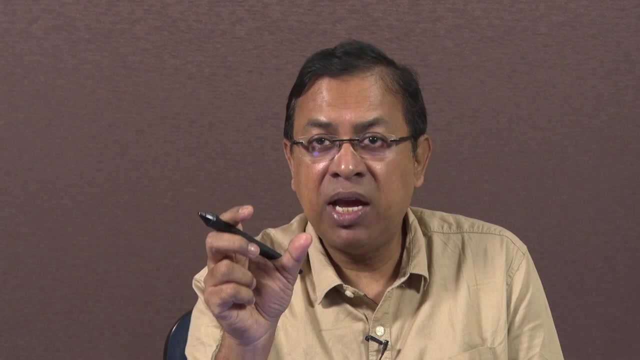 this thing there. So let us write it with A n. so A? n is a normalization constant And the wave functions are, for a harmonic oscillator, are known to be a convolution of a gauge, n, which is exponential minus alpha x square or alpha y square, multiplied by a polynomial. 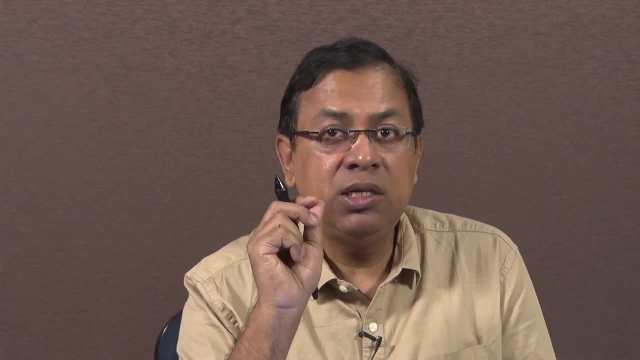 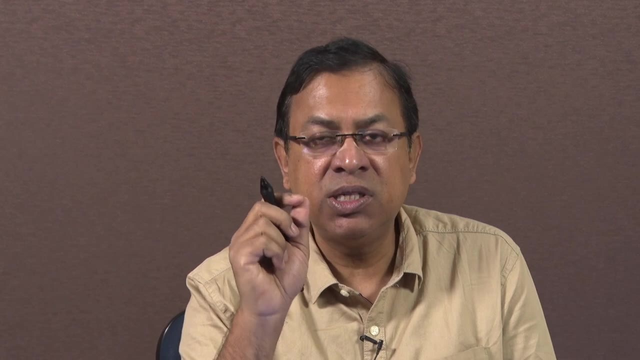 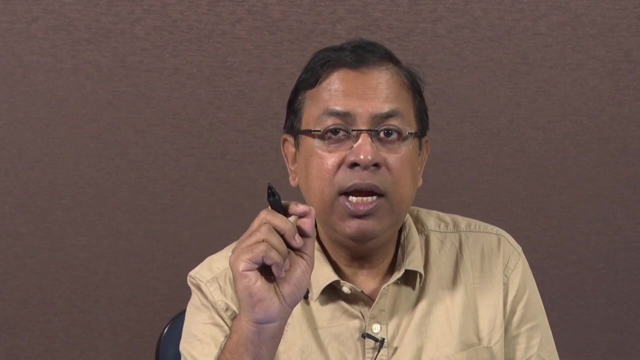 function which is called as a Hermite polynomial, and this polynomial has a property that when n is even, the polynomial is even, that is, it contains terms such as x to the power 0,, x square, x to the power 4, and so on. When n is odd, it contains terms which are x, x, cube. 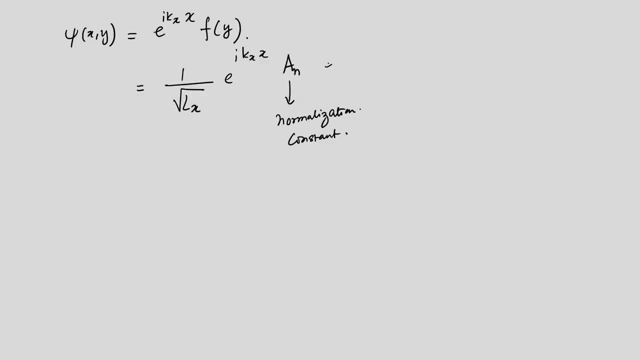 x to the power 5, and so on. So this is that form that we have to write down. So this is equal to Eb, whole square divided by h cross, which is the Gaussian part. Just reminding you that this is the harmonic oscillator and you have a Gaussian like this: 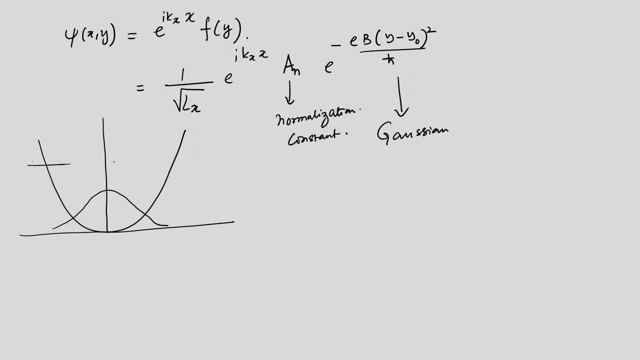 for the, for the ground state, And this is for the first excited state. it is like this, and so on. So this is an odd function, So this is a ground state, and this is the first excited state, and so on. So, and then, 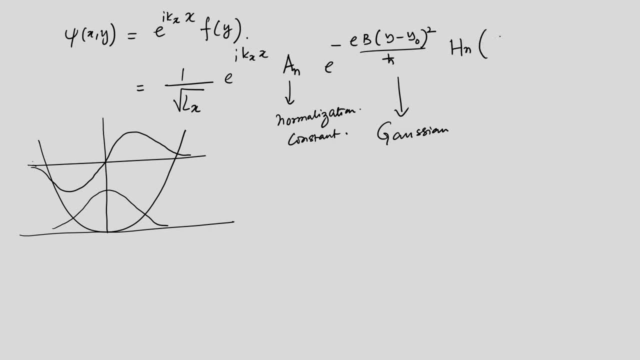 there is a Hermite polynomial, and this Hermite polynomial is written as Eb y minus y 0, divided by h cross, etc. The exact form is not important for us at this moment, but we need to know that at least this: there is a Hermite polynomial. 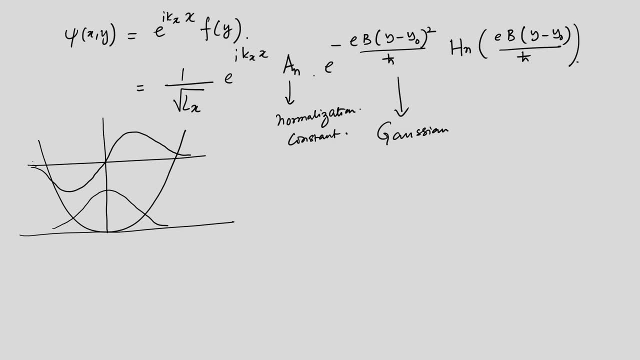 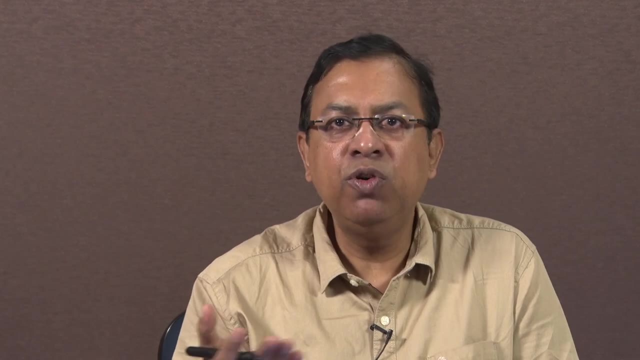 and then there is a Gaussian term which comes with a normalization constant, and this part is purely because of the x part and this is because of the y And, as I said, that the z component, even if you consider it is like a free particle in the z direction, In particular, 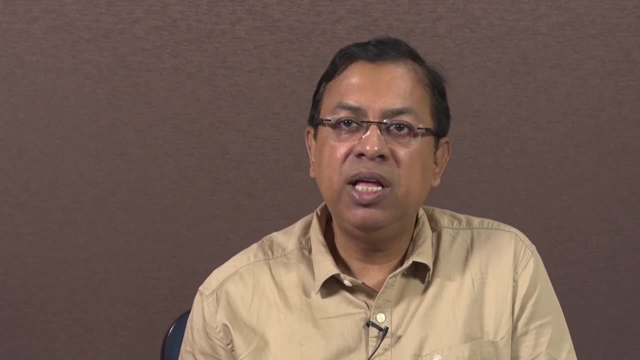 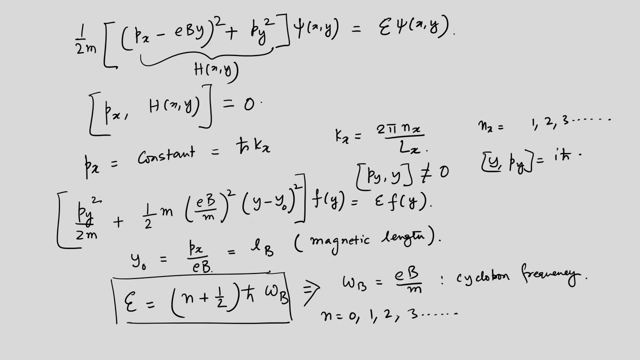 if you confine electrons in two dimension, Then that term does not arise. Now, if you go to this last slide, you have n plus half h, cross omega, And this n equal to 0, 1, 2, 3, etcetera. these are called as the Landau levels, So the energy. 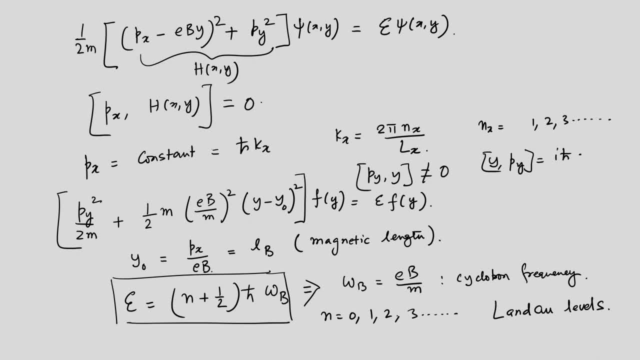 levels have a name which are called as a Landau levels, And Landau is a Russian physicist and the wave function is actually Stauffer, Chrom, Ellis, logic, And here are other things missing because of the khác structures. hereTION result is everywhere: x, log, n, log, n. So this: 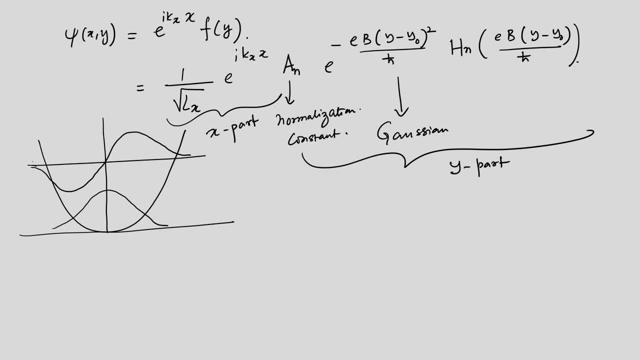 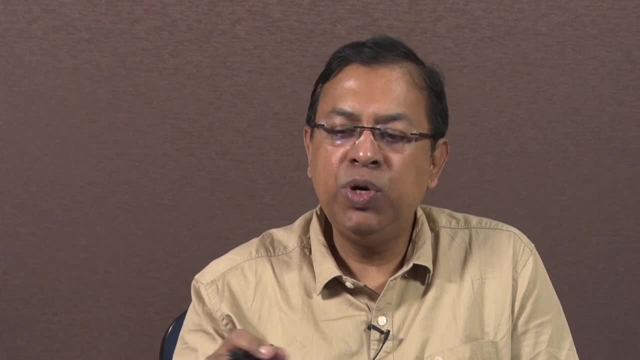 is actually true. now, Пол分 persuad deber. x log of a Kb square bra assassin ở x cole. objective: a freely propagating part in the x direction multiplied by a harmonic part which is executing a harmonic oscillation which has a Gaussian term and a Hermite polynomial n when n is. 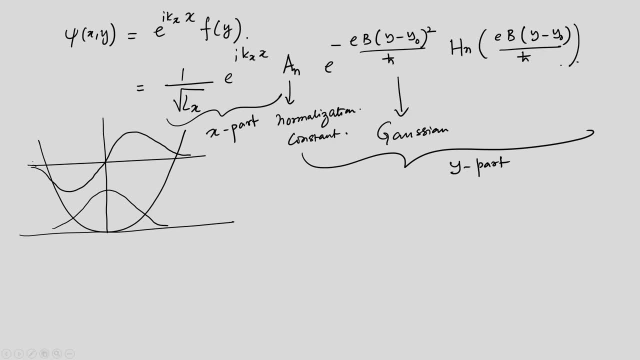 even the polynomial is, even when n is odd, the polynomial is odd, These Landau levels. so if we really plot it, how does it look like? the Landau levels will simply look like this: Okay, they are equidistant. okay, for a given value of b. so this is say: 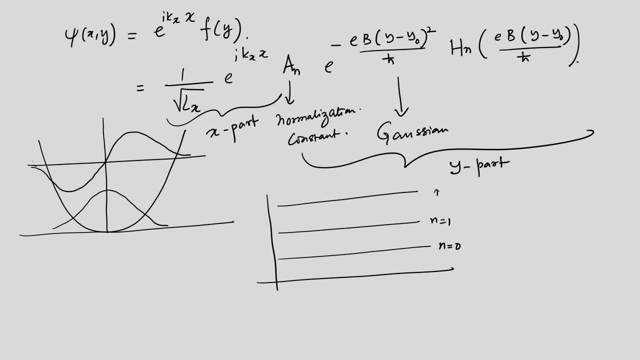 n equal to 0, n equal to 1, n equal to 2, and so on. but if you draw for another magnetic field, it may look like this, and so on. Okay, so then, n equal to 1, n equal to 2, n equal. 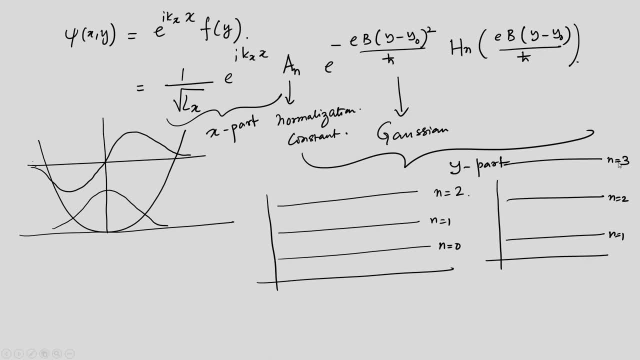 to 3 and so on. okay, And the reason is that, Okay, omega B, which is the cyclotron frequency, it is directly proportional to B. So as you increase B, let us say that this B1 for a magnetic field, B1 and this is for B2, and of 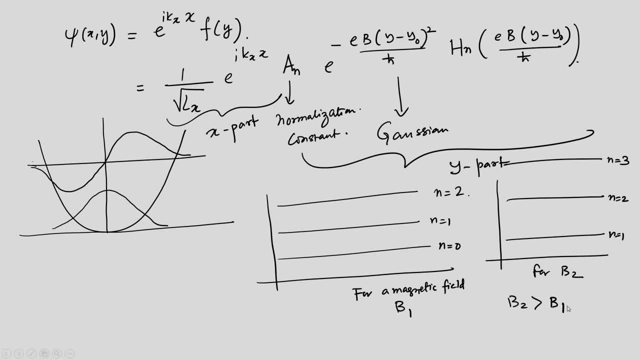 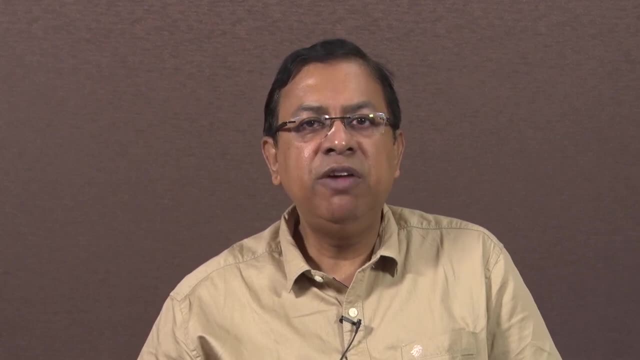 course, B2 is greater than B1, and these are called as the Landau levels. So now, what are the properties of the Landau levels? and we would eventually get to that that these Landau levels are the most important things in understanding the structure of the. 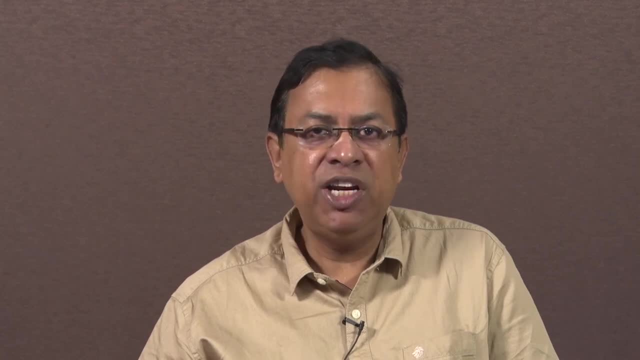 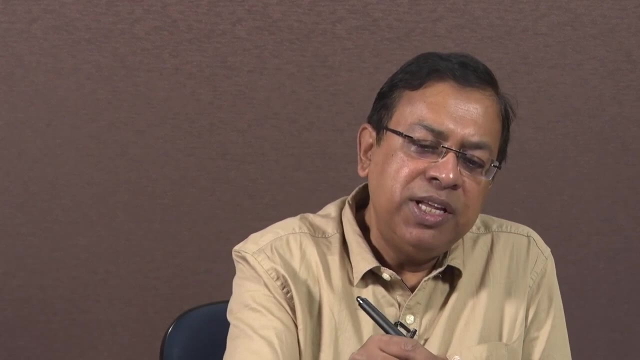 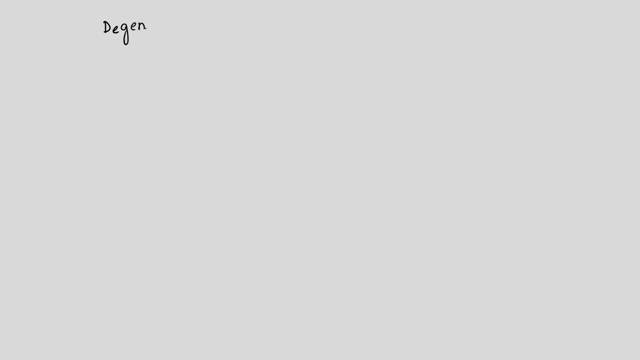 plateaus and these are not really very sharp levels because of disorder, these get brought in. we will come to that. There is one very important things: that these Landau levels are infinitely degenerate or their degeneracy is very high. So degeneracy of the Landau. 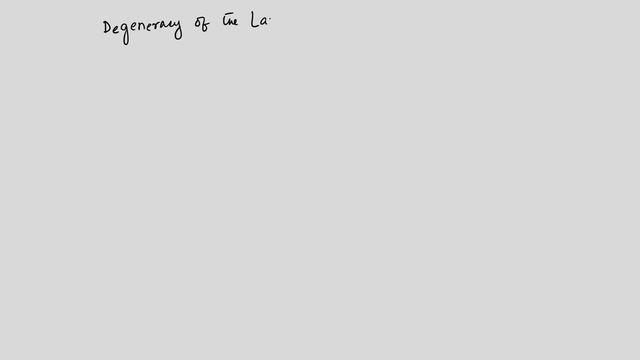 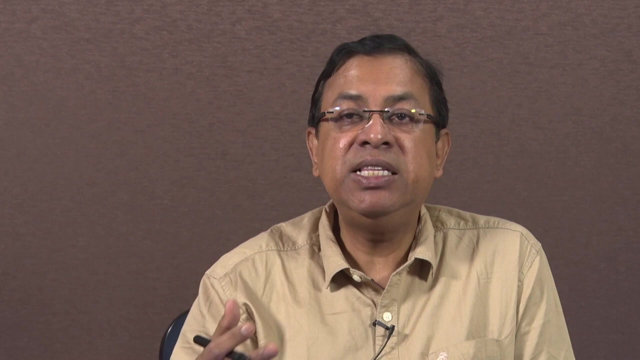 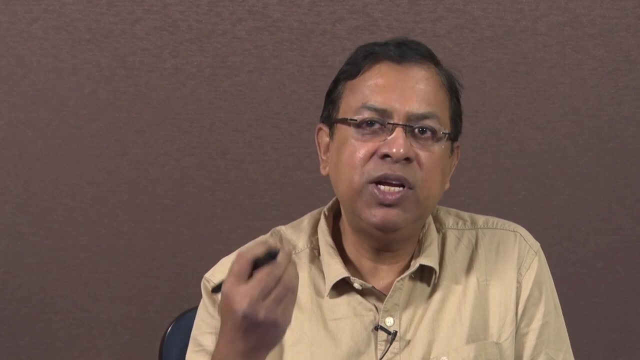 levels. So there are many, many states corresponding to each one of the n values. So n equal to 0 has very large, Which means that these states can be occupied by electrons. So each Landau level is occupied by many, many electrons. So let us understand the how that degeneracy arises and where does 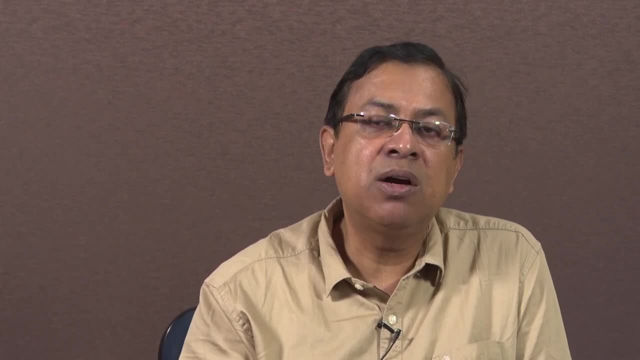 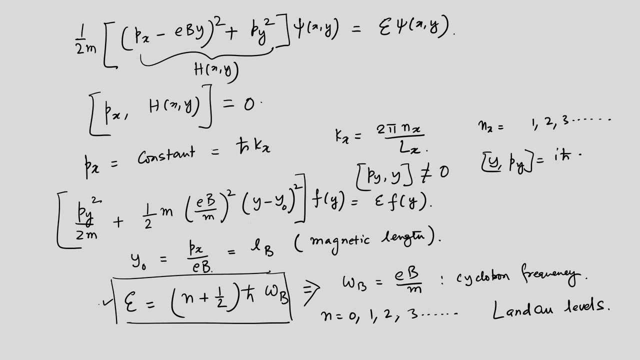 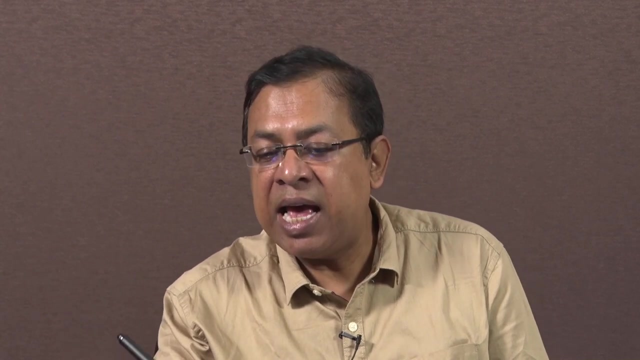 it come from. It comes from the value that kx is a constant and this result that you have got is independent of kx, So kx does not play a role here, which means any value of kx would give rise to this level, And this kx has a number of states, which means that 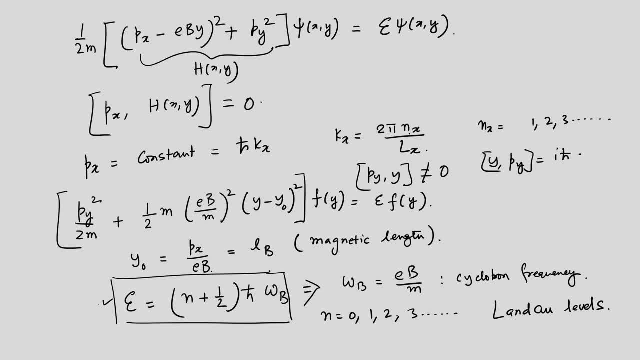 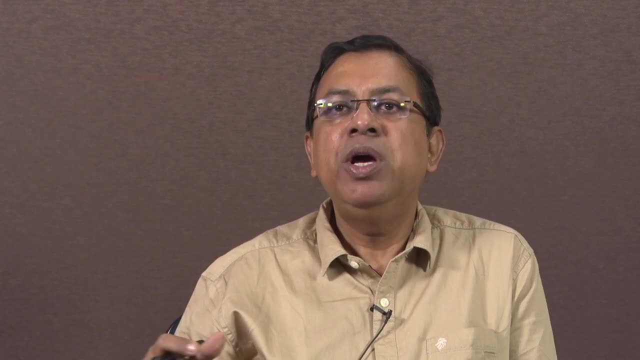 states which has nx associated with it, which denote a quantum number of the states, Which means that corresponding to any value of n- here a given value of n, there could be a very large number of values of nx that are possible. So in principle this is infinite, but the degeneracy 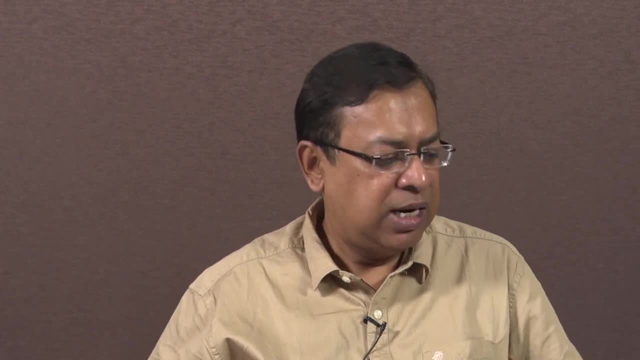 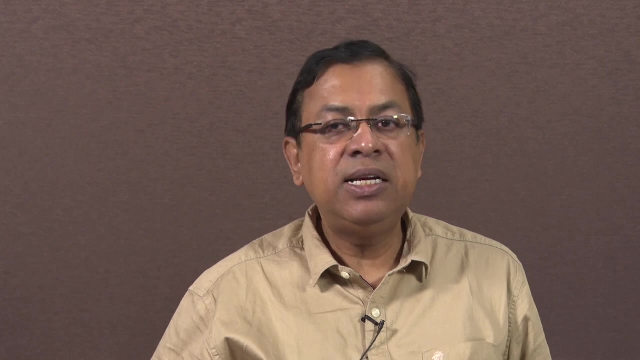 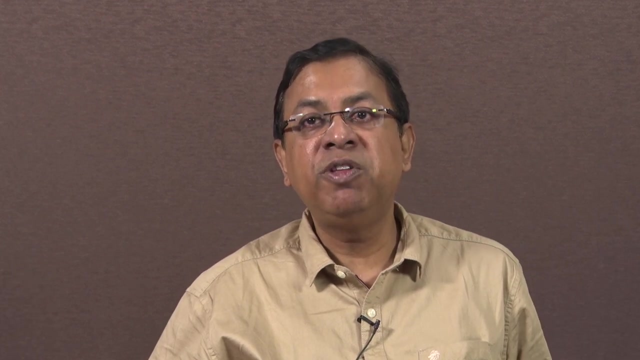 is actually limited by some factors, And let us try to understand that. what factors do they depend upon? But I hope that it is clear that these levels are heavily degenerate and the degeneracy is because they are coming from the fact that any value of kx would satisfy this. 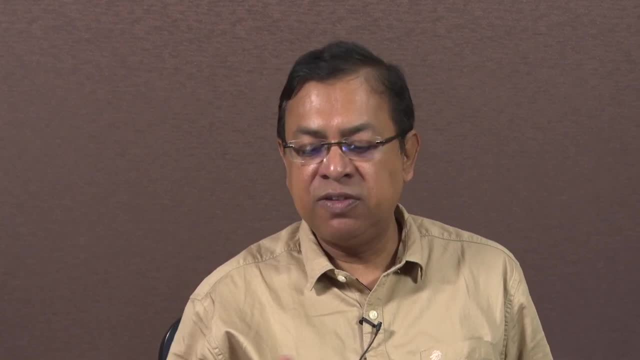 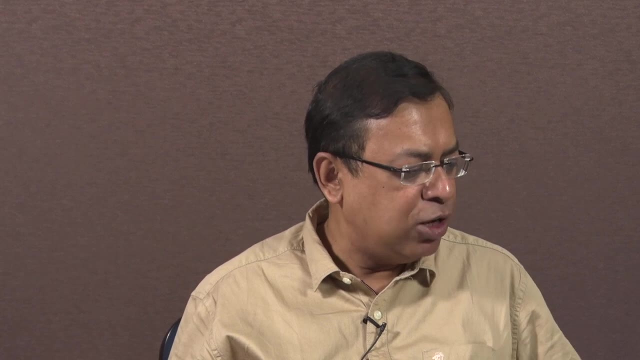 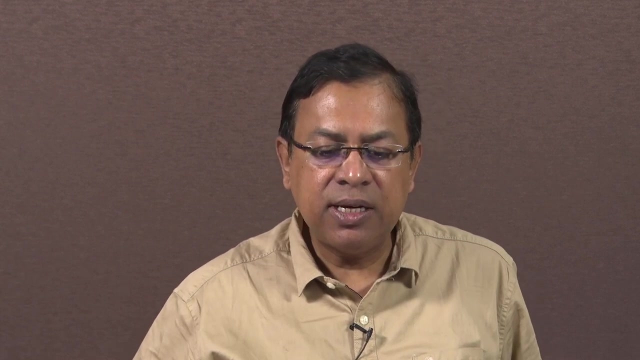 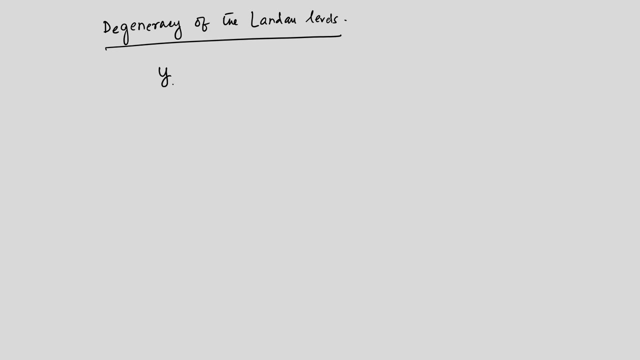 equation, or any value of nx would satisfy these energy levels. So each of the energy levels do not depend upon on nx and any value would be then acceptable solution. So if you want to know the degeneracy, let us look at this. So we have written this down earlier that the y 0 is. 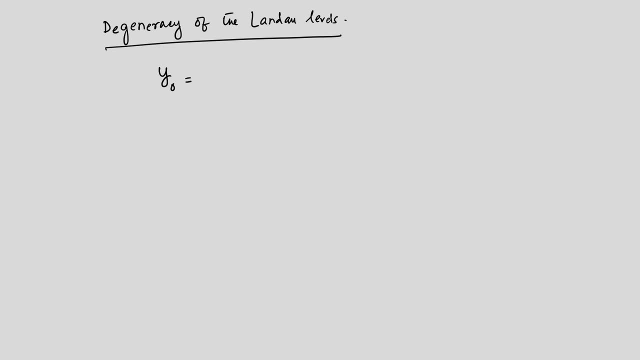 equal to. So we have y 0, equal to Px over Eb- We have written this earlier- and which we called as Lb. Lb is equal to Px over Eb. the magnetic length, and this is nothing but h cross kx divided by E, b, because px is h. 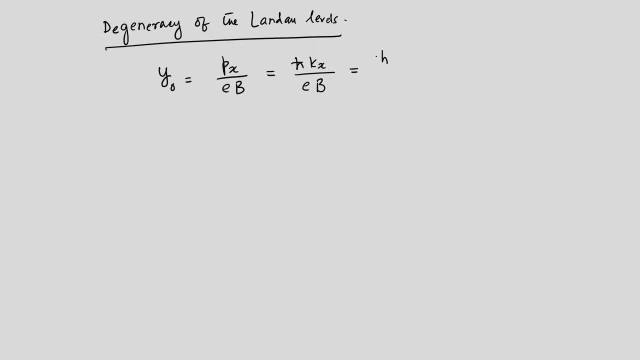 cross kx and this is equal to h cross kx is 2 pi nx by lx. So this is your y 0 and we want to find that what is the maximum degeneracy? So we want to find what is nx max. Ok, and 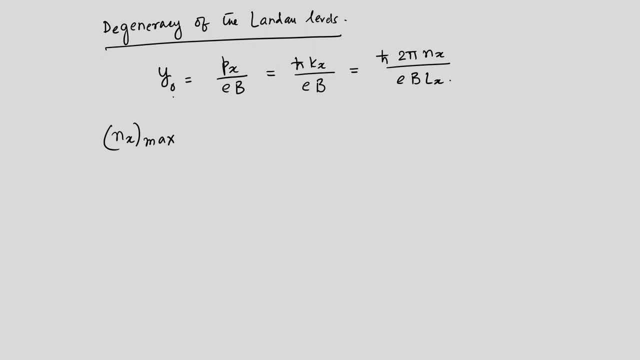 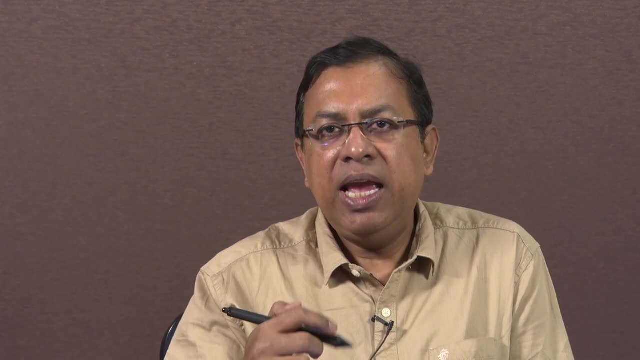 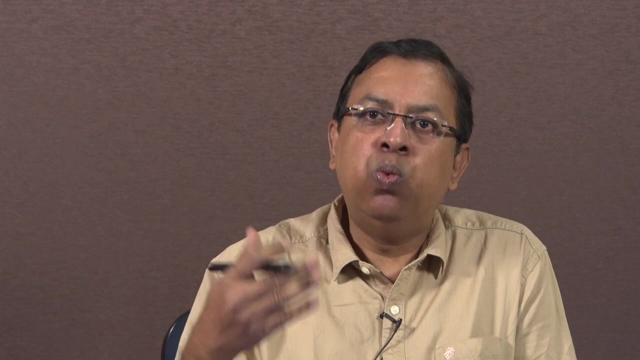 nx max. all others are constant. the y 0 is, the is basically a length scale in the y direction. Ok, Along the y direction, there is some value of y which is determined by, of course, a magnetic field. Now, this y 0 can at the most be L? y. the magnetic field can at the most be L? y of this, 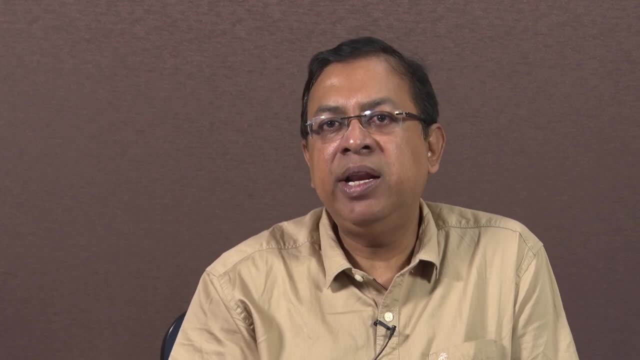 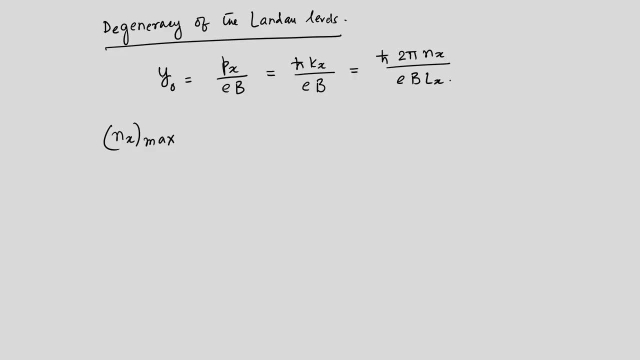 value of y 0.. So we want to find that what is the maximum degeneracy? We want to find y, that is the length of the sample in the y direction. that y 0 cannot be outside the sample. So the maximum value of y 0 will be L, y and so maximum value of N, x max can. 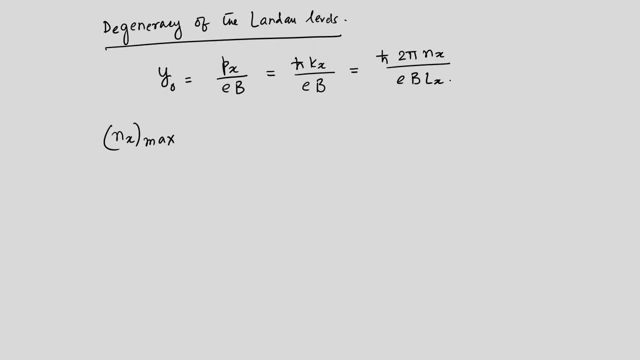 be obtained if you substitute y 0 as L y. So this is equal to E, b, L, x, L y, because I am putting y 0 as L y and this is equal to 2 pi h cross. So that is the maximum degeneracy. 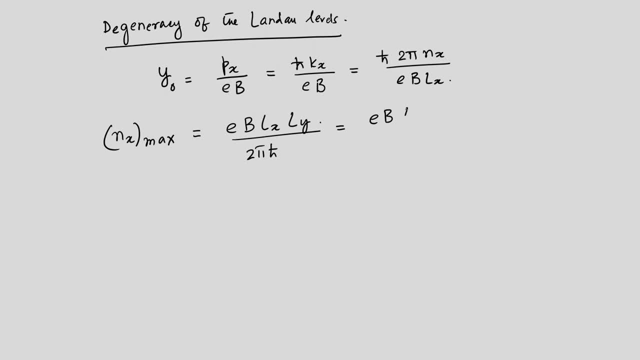 So this is equal to E, b into a. a is the area of the sample, do not confuse it with anything else. it is the. a is the area of the sample and divided by this, h, because 2 pi is the area of the sample. 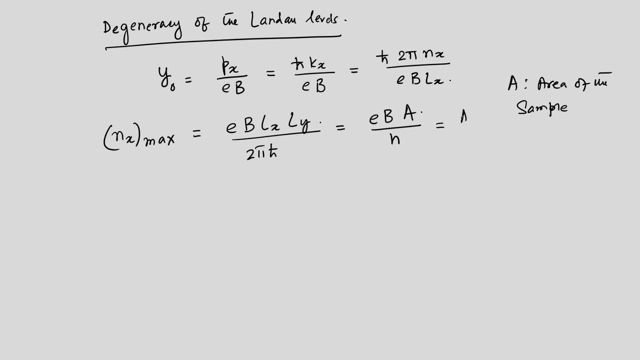 pi h cross is nothing but h. I can write this as a divided by h over e, and so I can take that b, this thing. I mean I can leave that b there and put this electronic charge below the in the denominator, because h over e is a very important quantity which is called. 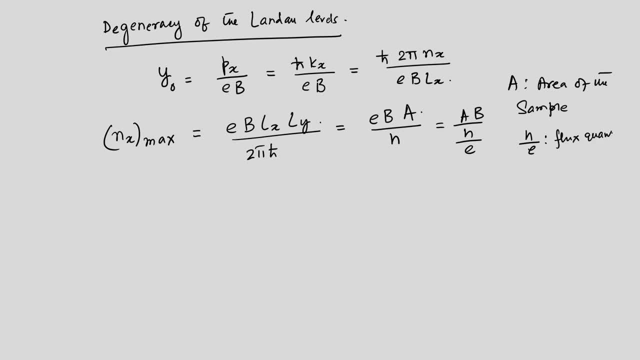 as a flux quantum which is denoted by some phi 0,. okay, So this is equal to a flux quantum which has a particular value in Weber, some 10 to the power minus 14, 10 to the power minus 15 value. So you see that let us call this as G, the. 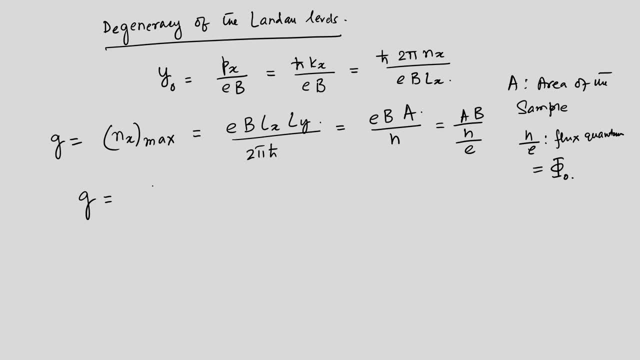 degeneracy, So G is equal to it- depends on the b, the magnetic field, the area of the sample. So and a, phi 0, and this tells you that this degeneracy can be infinite because a, b- if you go back to the first slide that we had and you see, here the magnetic field goes- 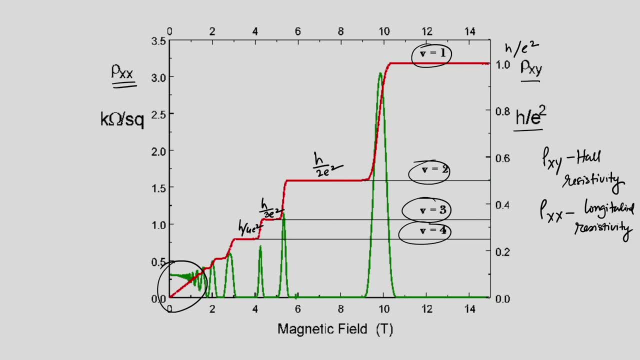 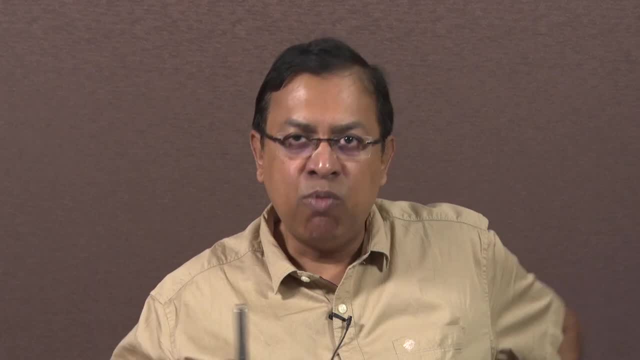 all the way up to 14,, 15 Tesla. So this is about 15 Tesla. So there is a 15 Tesla magnetic field. If you want, if you have facilities, you can increase that magnetic field even more. So and the sample size is up to 15.. 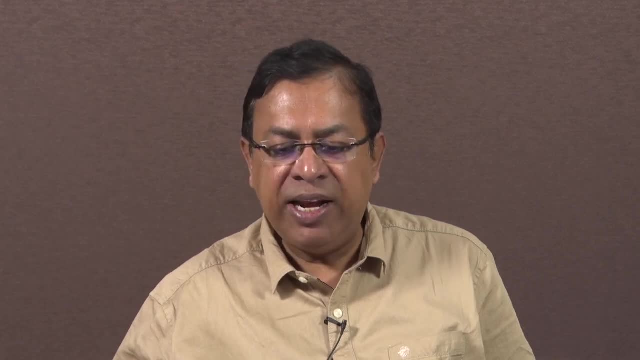 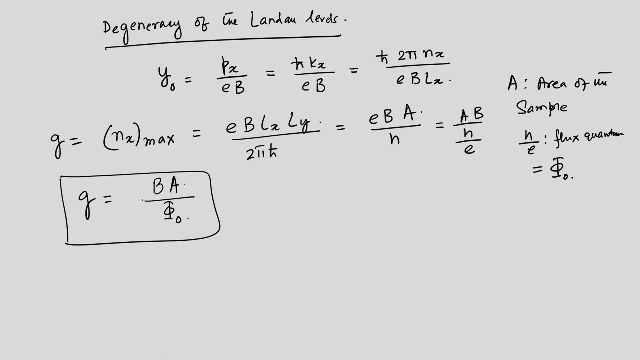 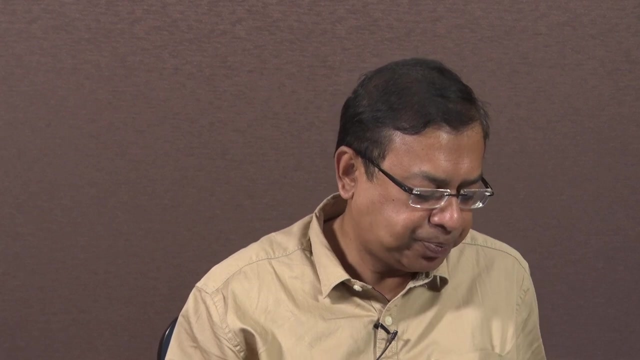 So this is up to you, okay. So this is really a very large degeneracy that is coming out of each one of the Landau levels are degenerate. In fact, this has important repercussions or implications on the fractional quantum Hall effect. okay, So two things that we notice. 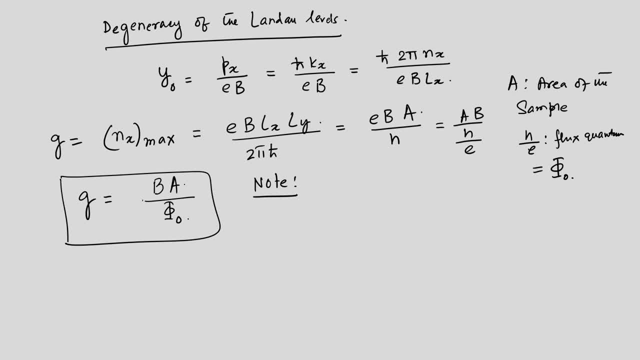 here. so you note that the degeneracy is, of course, what I told you, that degeneracy is proportional to, Is proportional to b and a. I told you b is a magnetic field and a is the area. and the second is that you know the trajectory can be, the trajectory is centered about some. 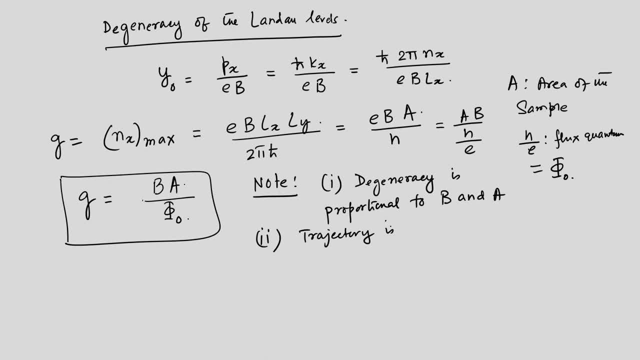 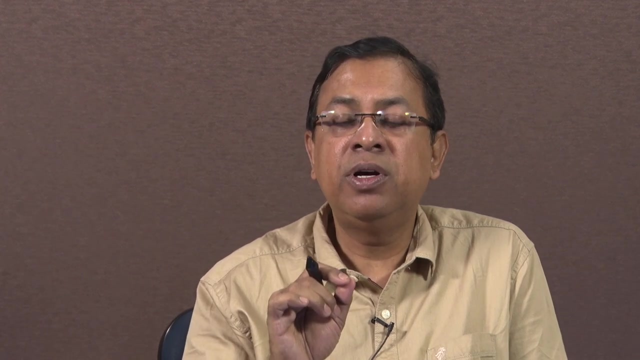 y 0.. Is- Is Is centered in y direction and centered about y 0.. So these are two very important. you know outcome of this exercise that we have done, That is, we have solved a charged particle, a single charged particle, in presence of a perpendicular or a transverse magnetic field. 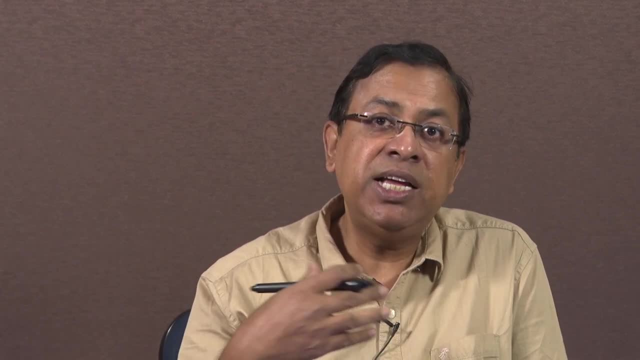 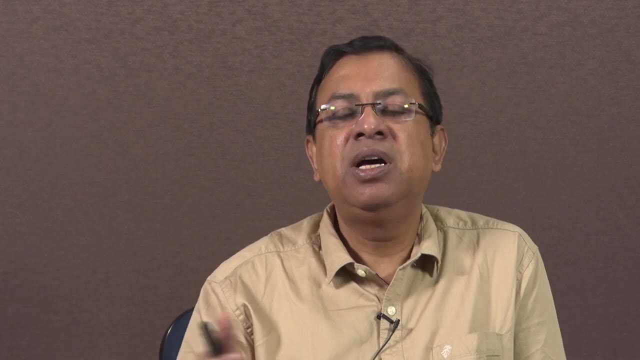 We have taken a particular gauge, and suppose we have taken the gauge in which the magnetic vector potential is in the y direction. in that case you will have just the x and y being interchanged, that the system, the particle, will propagate like a free particle in the 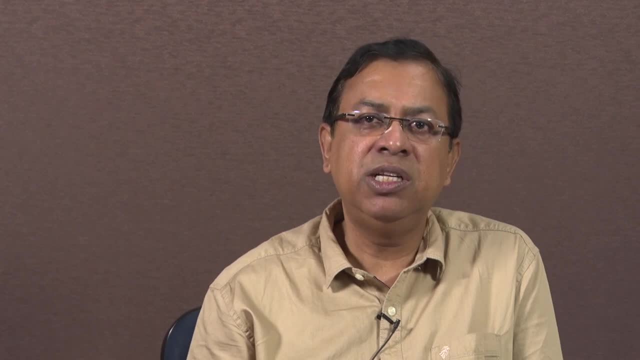 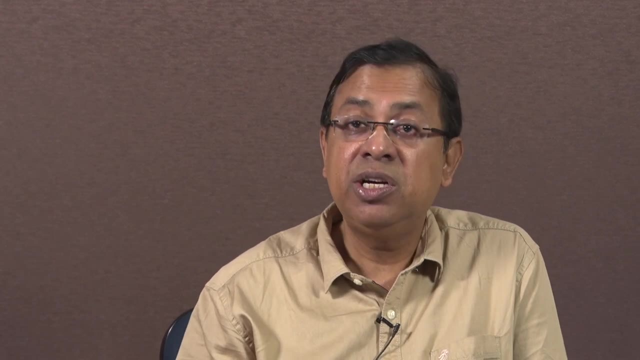 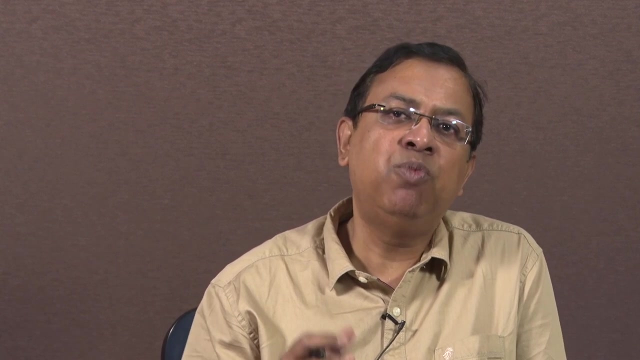 y direction and will execute a simple harmonic oscillation in the x direction. So x and y, they have no specific significance. and the third gauge, which we will talk about later. It is called as a spherical gauge or symmetric gauge, and in that case you have both x and 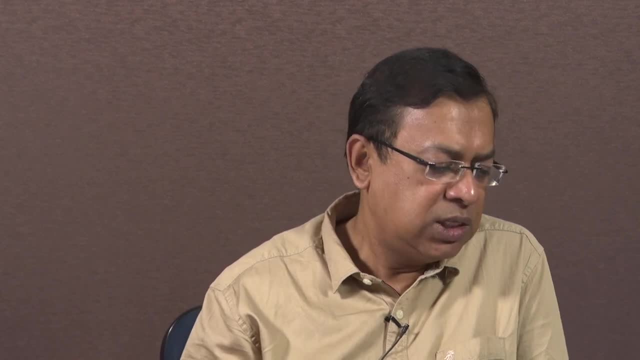 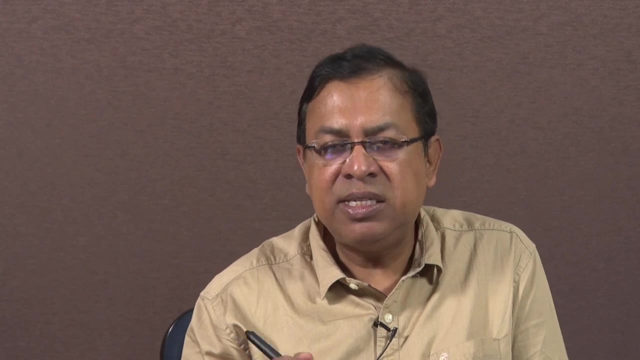 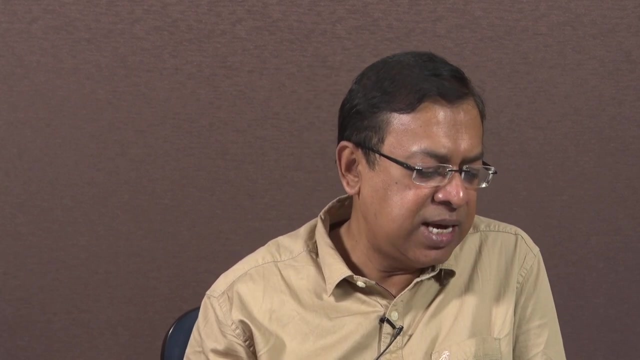 y component and these Landau levels are actually found out to be circular. Okay, So now there are some incidental similarities, which I will just point out and will discuss them as we go along. And the similarities are that the hall resistivity, it shows plateaus. 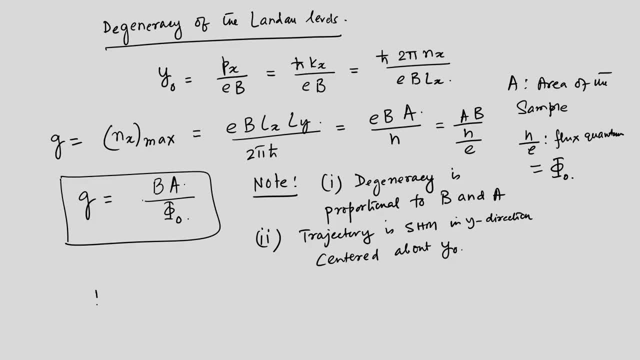 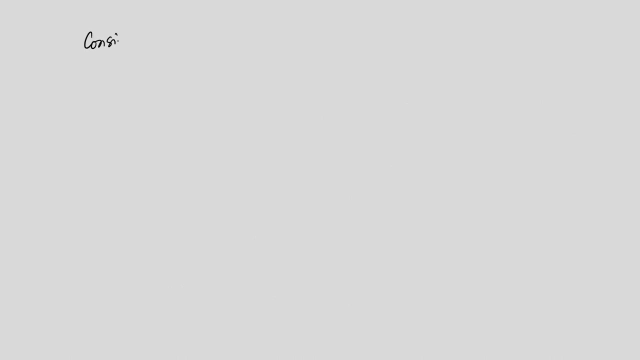 in multiples of H over b. these plateaus are H over E square. okay, So H over, say, N E square or something where N is an integer. okay, So consider to be N 0,. okay, that is the density of carriers. So 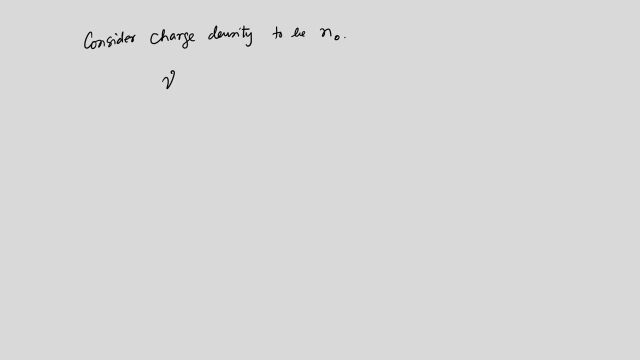 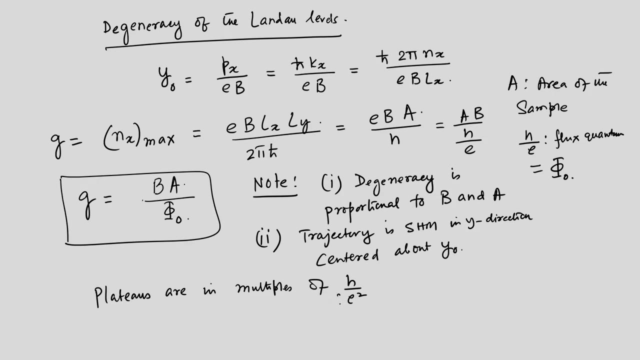 define a quantity called as nu, or let us call this as just what we called here as N. let me call this as N, this as nu, where nu takes values 1,, 2,, 3, etc. We just change this because the too many. 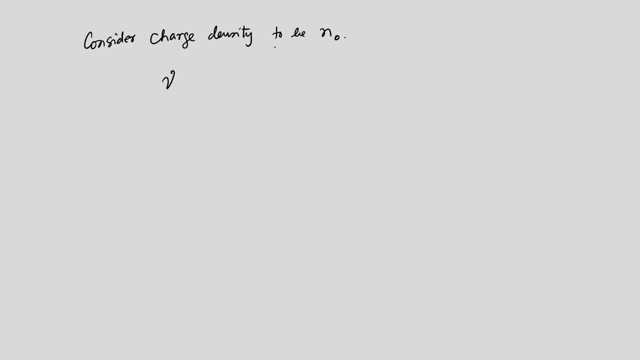 n's n is used for density as well. So consider charge density of the carriers to be n, 0. So nu is defined as n, 0 divided by G by A. Now this G by A is the degeneracy per unit area. So let us not have the geometry of the sample coming in, because you can have any. 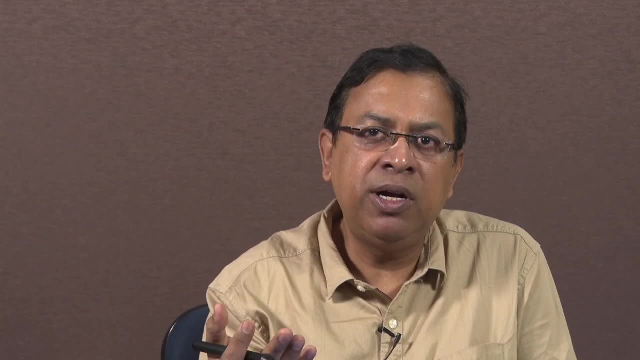 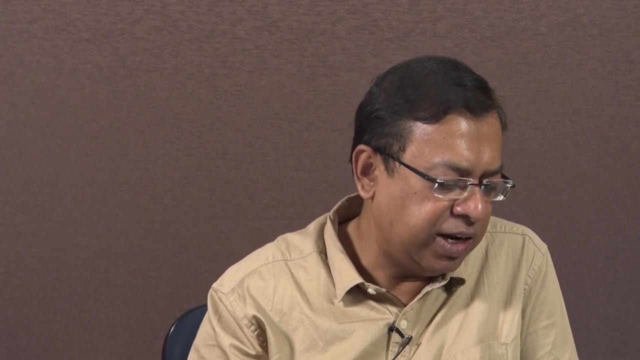 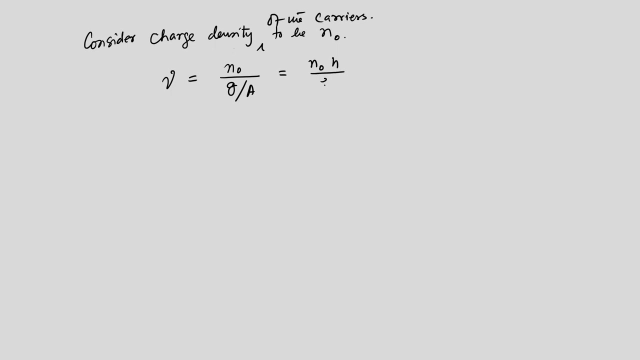 geometry. but if you divide it by A, then it becomes a fundamental quantity which only depends on the value of the magnetic field. And we are now talking about a given value of the magnetic field, And this is equal to nothing but n 0, H divided by E, B, and this is equal to: so this is equal to a number of. 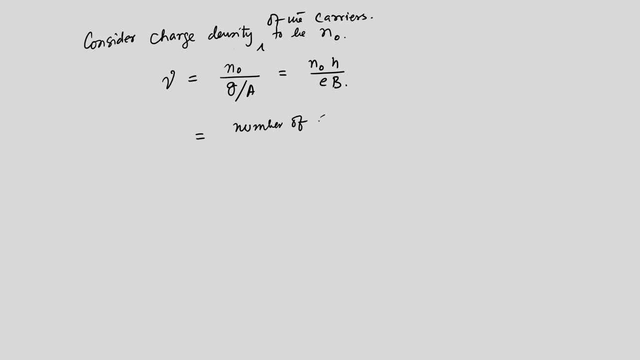 electrons, And I can, I can write this as n: 0 divided by H over E into B, so that is the flux quantum. So this number of electrons n divided by the, you know the number of B's, of flux quanta and so on. So if nu assumes a value integer, that is when the number of 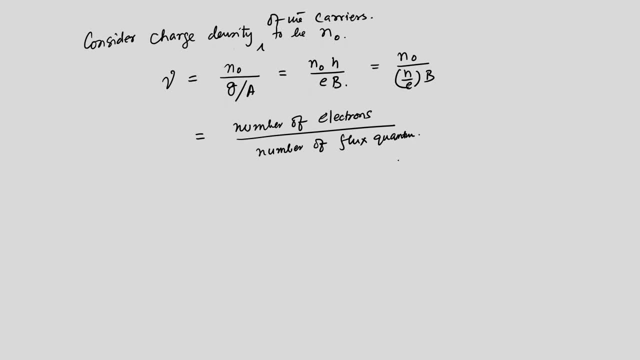 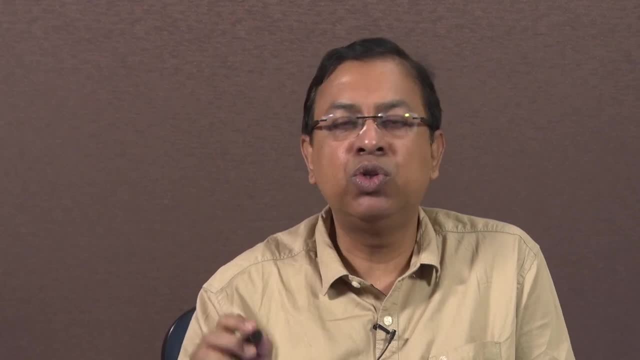 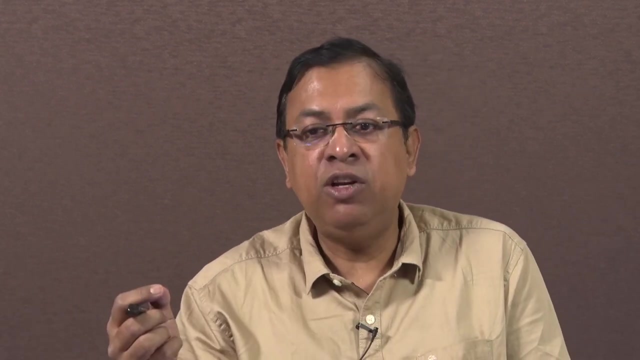 electrons and the number of flux quanta they become commensurate fractions or even fractions in the fractional quantum Hall effect. then there are plateaus that are seen in the resistivity. So these, depending upon- now you tune in- the value of the magnetic field, go back to this. 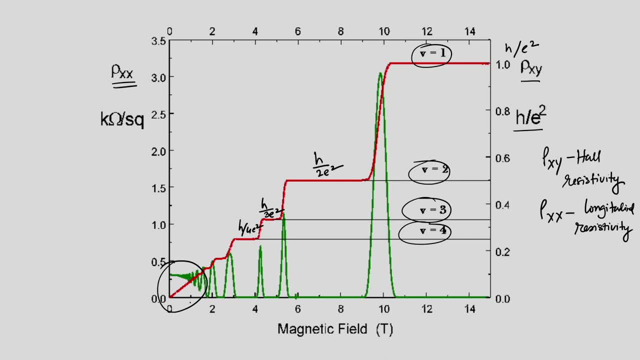 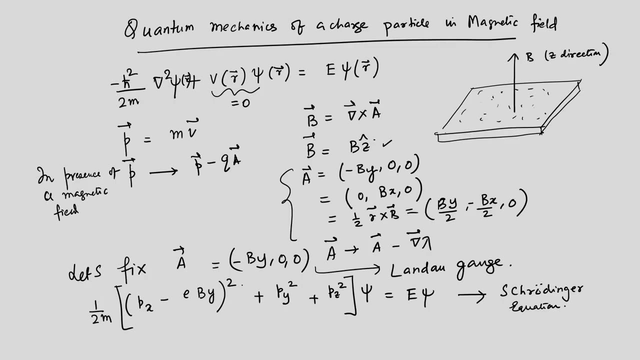 first slide which we had. you see, the magnetic field is being continuously tuned from a value 0 to 15 Tesla. So magnetic field is continuously ramped up and you are doing this experiment and what you see is that when this quantity which we just found out, that this quantity 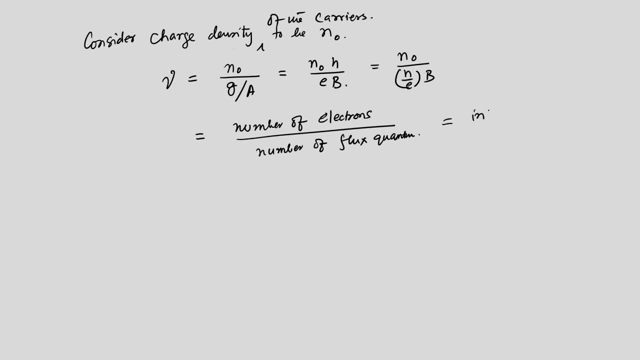 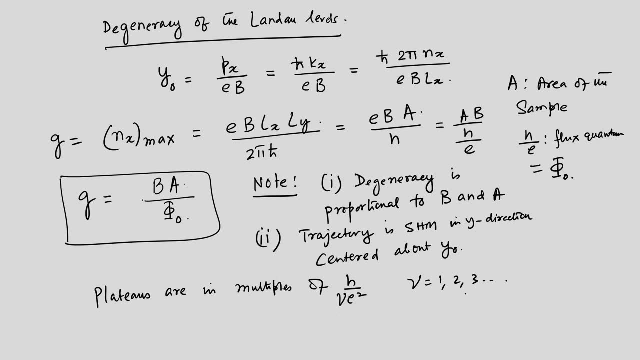 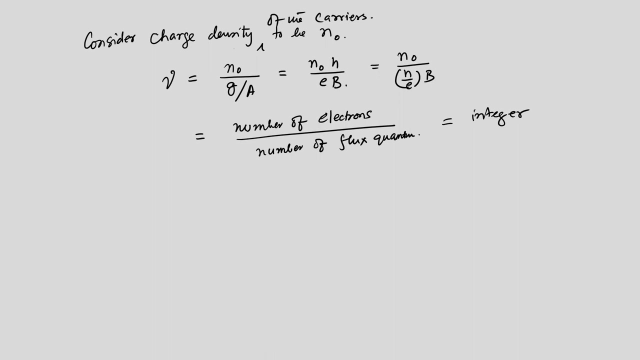 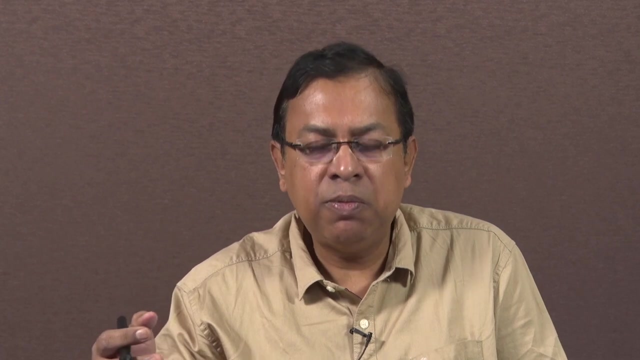 becomes an integer. Then there are these Hall plateaus which are seen, which we saw last. So when this becomes an integer, you have a plateau, which means that this ratio becomes an integer. you see plateaus. then you again tune B. this goes from being an integer to a fraction. then you no. 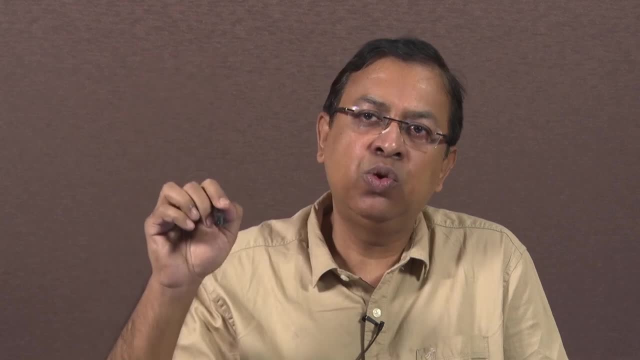 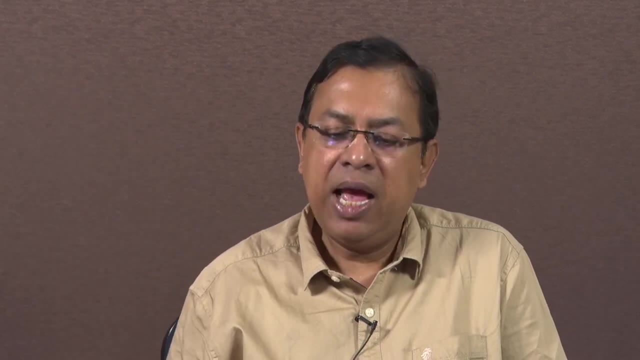 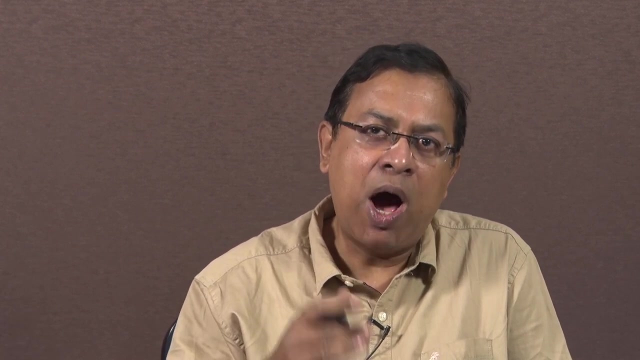 longer see plateau and then this thing, the resistivity gives, shows a jump, and then you go to the next integer, such that it shows another plateau. and that is how this nu actually would be. you know, sort of it will go from one integer value to another integer value. 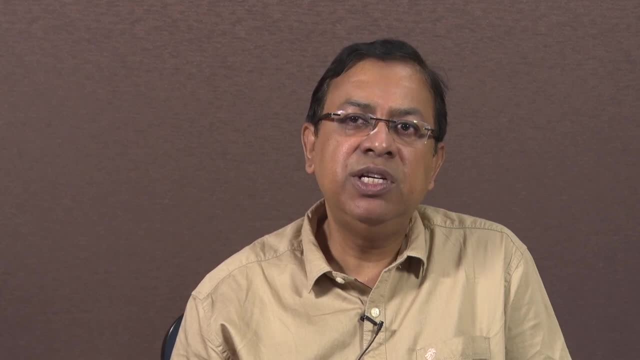 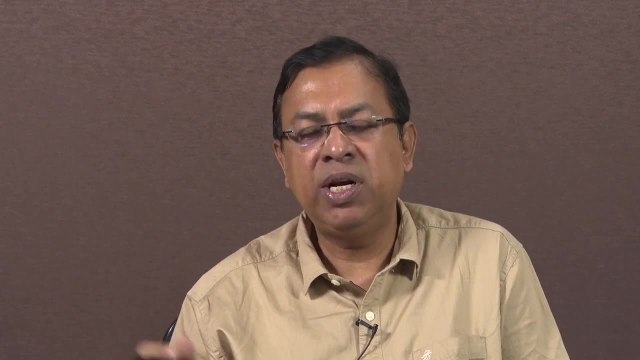 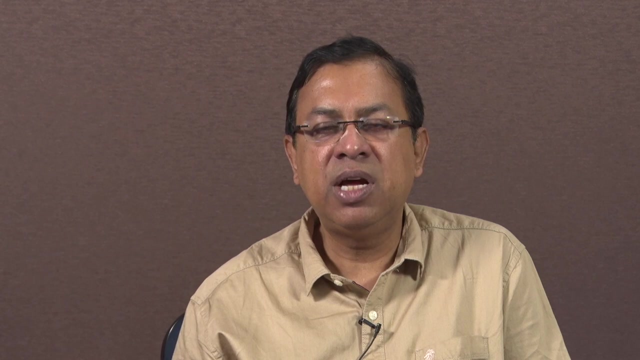 and it will pull along the resistivity of the material to be having plateaus and so on, and from one plateau to another, And this is what we are going to see more carefully. I will give you a list of references that you should follow. some of them are advanced.